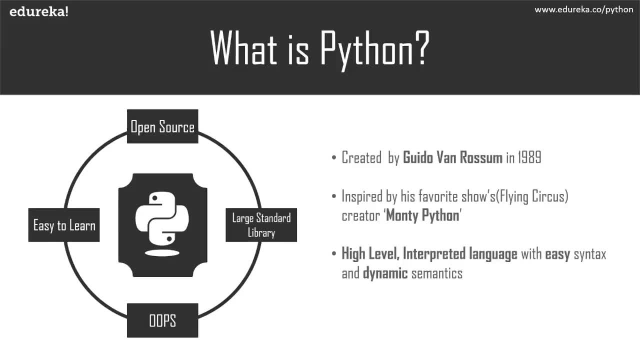 Python has gained popularity recently with the rise of machine learning and artificial intelligence, as python makes code writing easy and efficient. So, formally saying, python is a high-level interpreted language which has easy syntax and dynamic semantics. So what do these four keywords mean? Well, high level means. 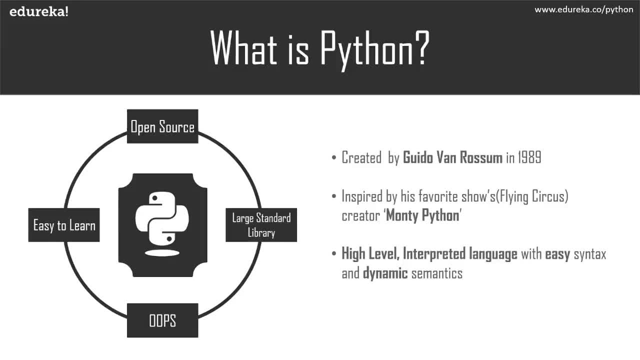 that python derives components from the natural language that we humans used to communicate with each other. This makes it easier for anybody to try and relate what exactly could be happening without the burden of going through tons of machine code. interpreted means that the python code is compiled line by line. 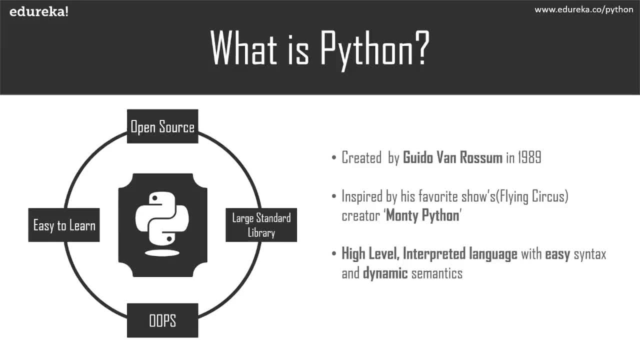 which makes debugging errors much more easier and efficient. But this comes at a cost, as python is much more slower than other programming languages. Python has easy syntax because it makes use of indentations instead of braces to distinguish what block of code comes under which class or function. 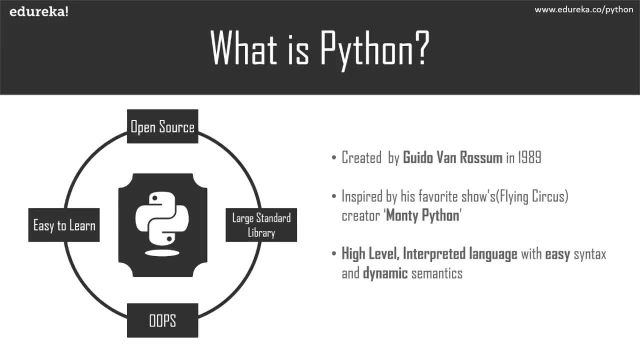 This makes the code much more distributed and easy for anybody to read. Python has dynamic semantics, meaning that you do not need to initialize anything before using it. Python does all of that dynamically, So I hope you have a clear idea of what is python. 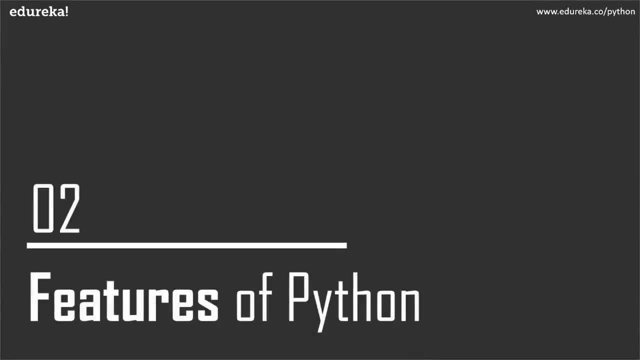 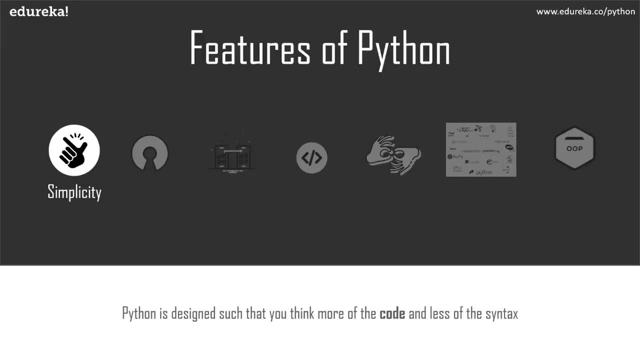 Let us go ahead and understand the different features that python provides us. So, as you can see, python has a variety of features that it provides us. Let us go ahead and understand each of these one by one. The most well-known feature of python is its simplicity. 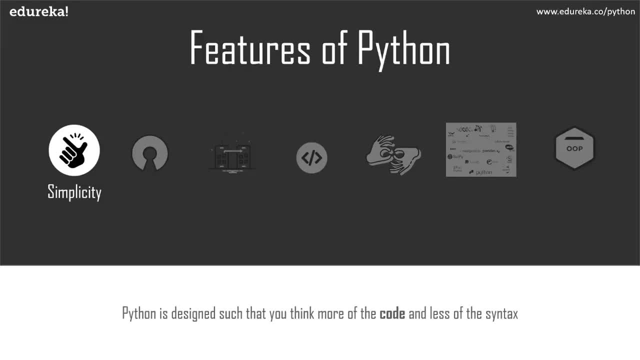 Python has made programming fun because it is simple. It makes you think more for obtaining the solution of your problem rather than thinking for the syntax of your code. The next important feature is that python is an open source language, which means that it is free for anybody to use. 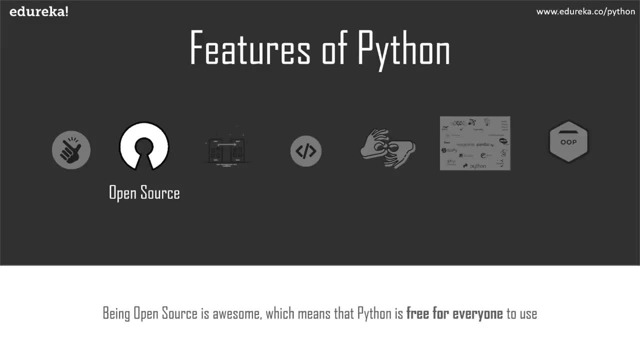 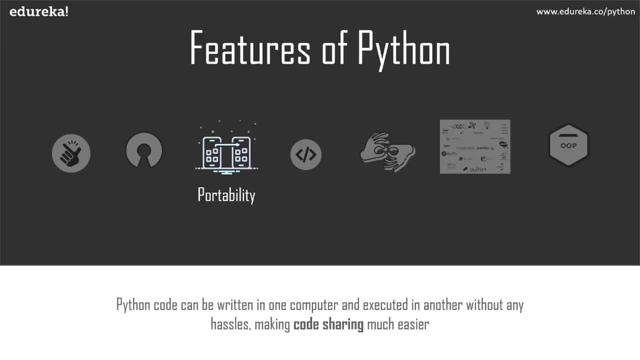 You can also modify python accordingly so that it better benefits your needs without any repercussions. which brings us to our next feature: portability. Python supports portability, which means that you can write your code and share it with your team members or anybody that you want to, and it would run the same way. 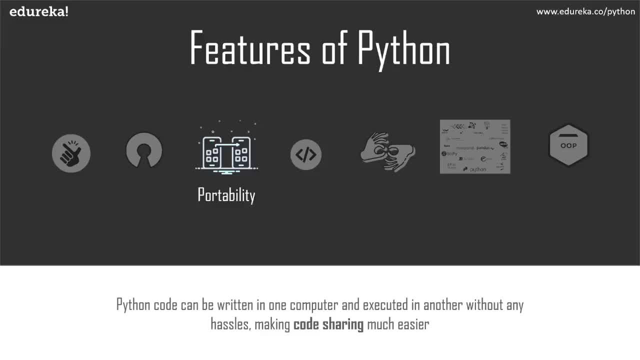 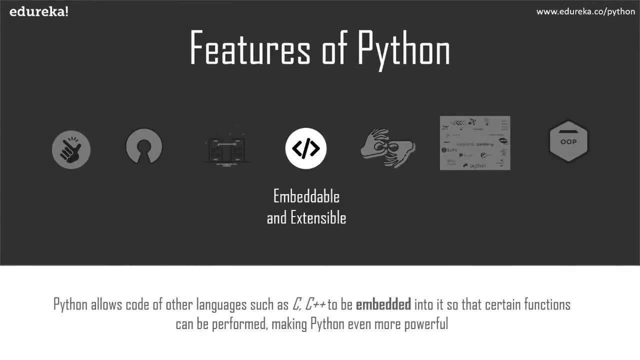 as it does for you. This makes it really helpful when you are working on an application with a team of people. Our next feature are the embedding properties. There may be chances that certain languages perform certain functions better than python, but that does not stop you, as python allows you to add. 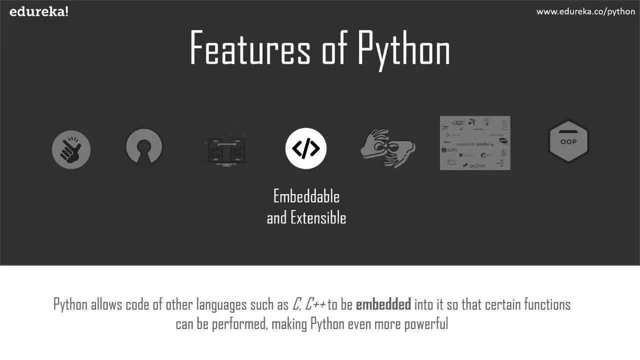 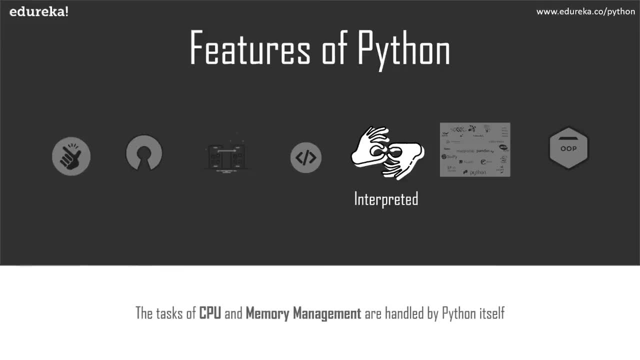 the code of those particular languages within itself, which makes python all the more powerful. with that, Let us move over to the next feature: interpretation. Python is interpreted line by line, which means that the management of memory and CPU is much more efficient and easy. 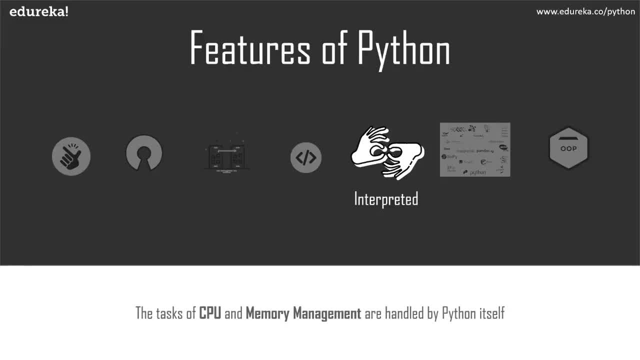 A whole program may take up a lot of memory, but python would take away the block of code that has already been executed. This frees up memory and makes the code run much more better. Now, if you are wondering whether python is the language to get started off with, let me tell you that it is. 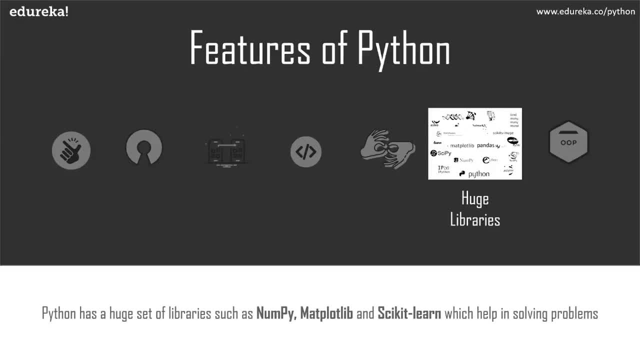 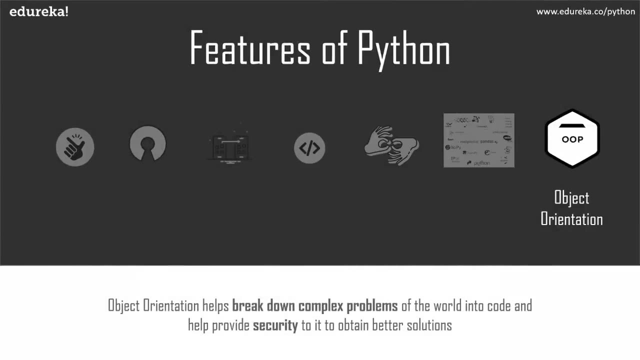 which brings us to the next feature: library support. Python has a huge library support which would help you to obtain solutions to your problems easier and much more efficiently. You can get started off with data science or web development on the go with python. You may have also had questions like: how do developers 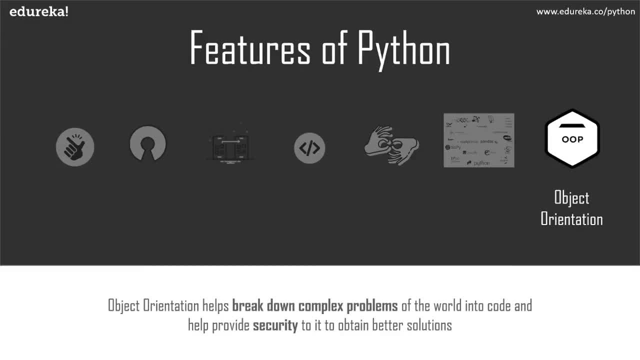 make applications that are so well related to a particular domain. That is because of object-oriented concepts. Python also supports oops, meaning that you can model a real-world problem into your code and you can have security for it, such that certain features only access those particular data elements. 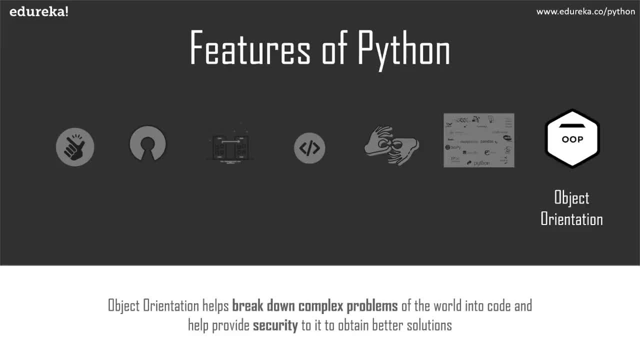 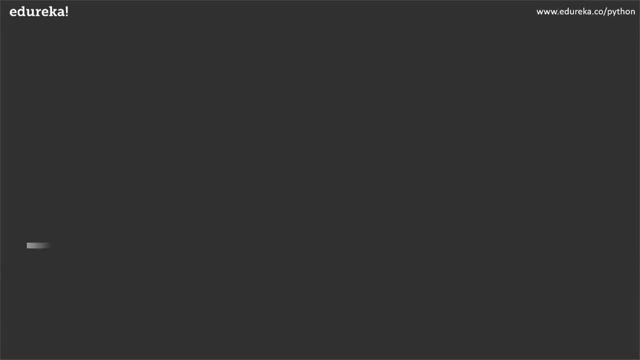 This can help you in remembering and replicating real-world problems. So we have gone through the features that python provides us. Now let us understand the different companies who use python in the industry. There are thousands and thousands of companies who use python for their daily business standards. 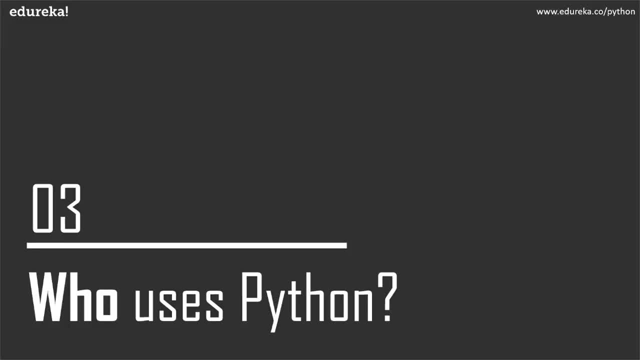 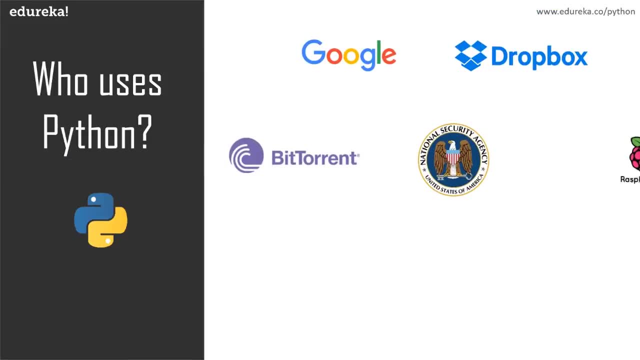 I have just listed a few of those, So let us go ahead and understand. how do these companies use python? We have companies like Google, Dropbox, BitTorrent, Raspberry Pi, National Security Agency, NASA, YouTube and Netflix, So let us understand how do these companies actually use? 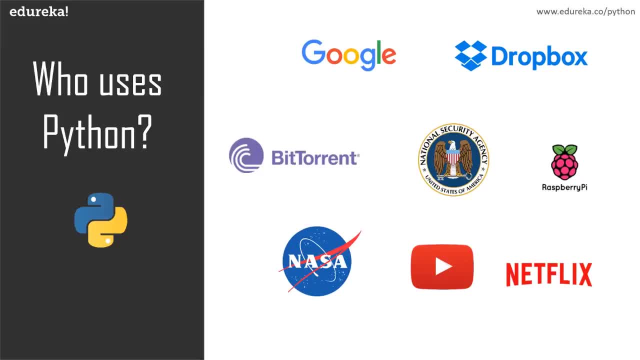 python to provide their features. Google uses python to provide better search features to its users. The Dropbox server and client applications have been coded using python. The National Security Agency uses python for cybersecurity analysis and also for encryption and decryption purposes. BitTorrent uses python to share files between the users. 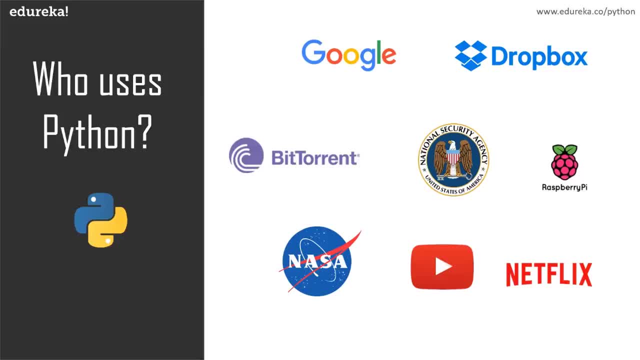 It had started out as a simple python file and is now an application that millions of users use. Raspberry Pi is a credit size computer which promotes python as its educational language. The scientists at NASA use python to perform scientific calculations. Netflix uses machine learning to understand and cluster. 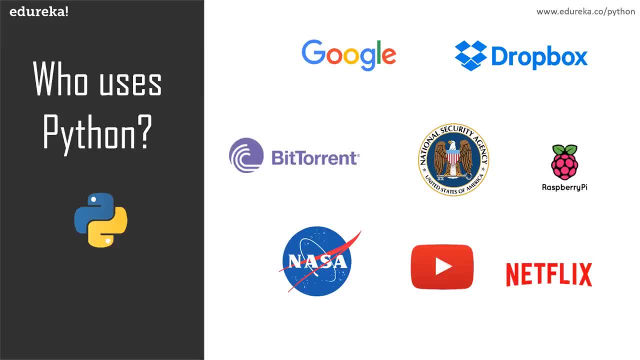 certain groups of its users and recommend them TV shows to retain them for longer. This machine learning is done using python. YouTube uses python to provide better searches to its users. So, as you can see, python is a really important language and there are huge number of companies who use it around. 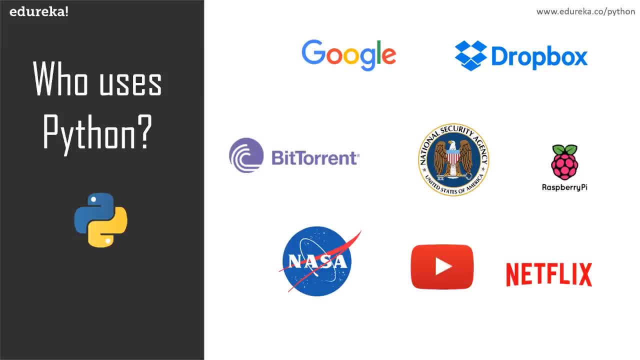 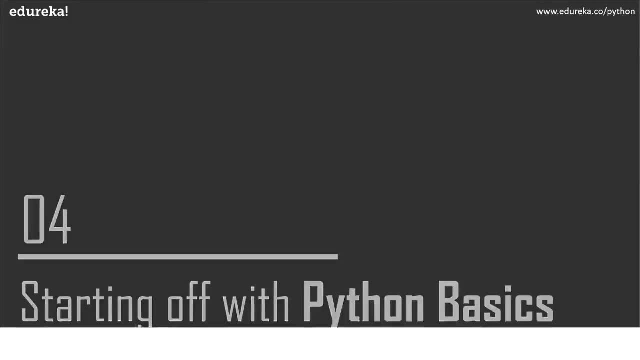 the world. So now, having understood what python is, what are its features and who are the companies who use it, Let us go ahead and get started off with our python basics. So to get started off with python, you would firstly need to install it onto your computer. 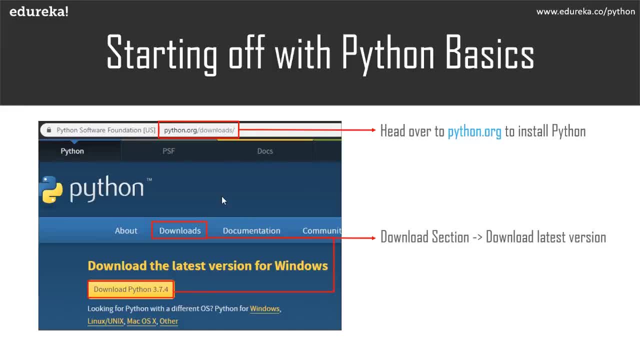 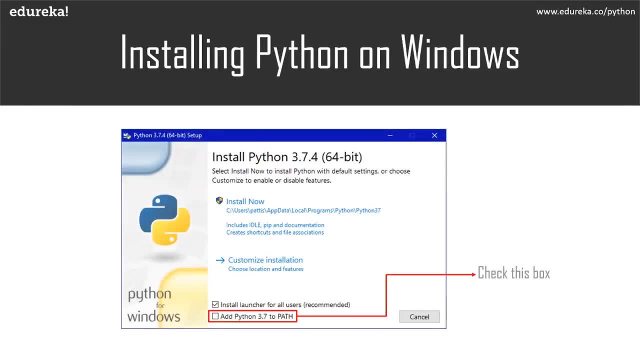 head over to pythonorg and download the latest installer that is available to you. Once the installer has been downloaded, run it and make sure that you check this checkbox. add python to path. What this will do is it will make sure that python is installed globally throughout your system. 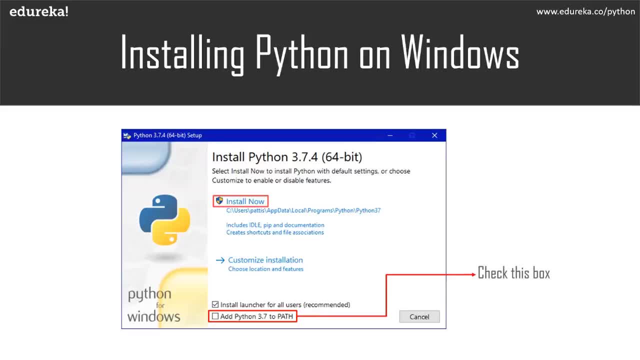 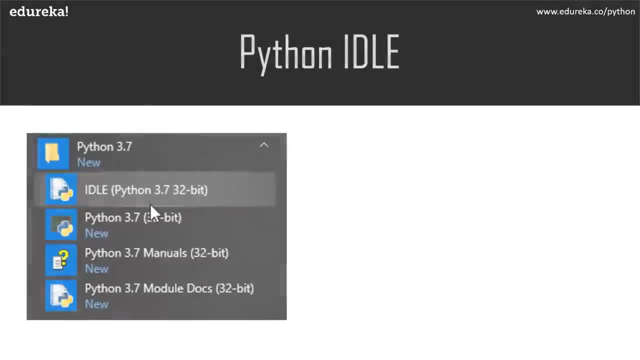 and you can access python from any place that you want to. then go ahead and click on install now and you will see python being installed into your system. Once the installation is completed, navigate and you will be able to find python installed on your computer. Go ahead and open IDLE. 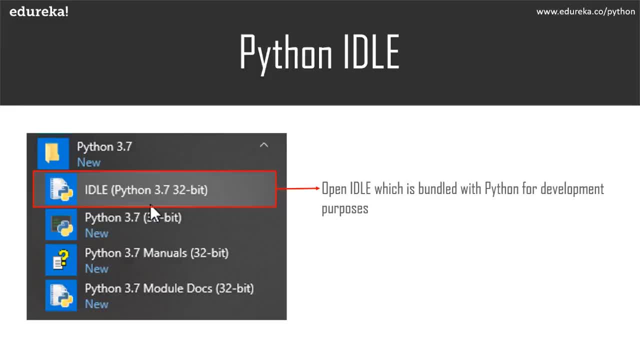 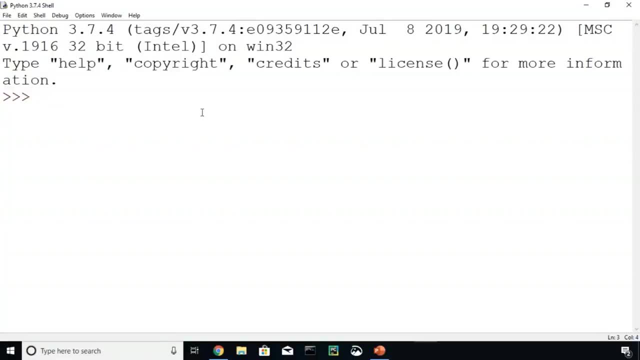 which is the bundled development environment with python. Let us go ahead and write a first program with IDLE. Do not worry if the font size of my IDLE is huge. I have done it So it is visible to you guys much more clearly. 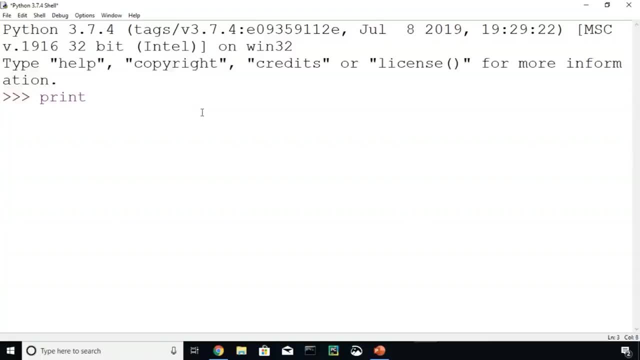 It may be small for you, So let us go ahead and write a first program that is to print: Hello users, Welcome to the basics tutorial. and let me hit enter and, as you can see, I have obtained the output. Hello users, Welcome to the python basics tutorial. 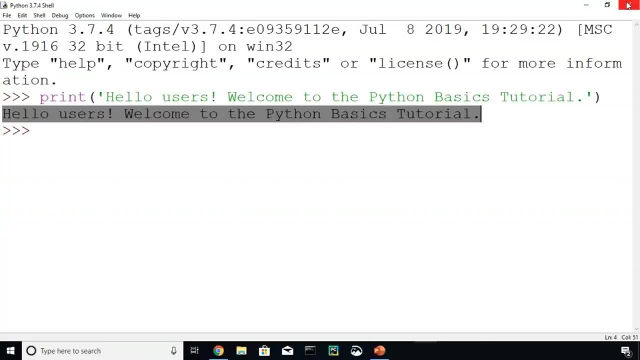 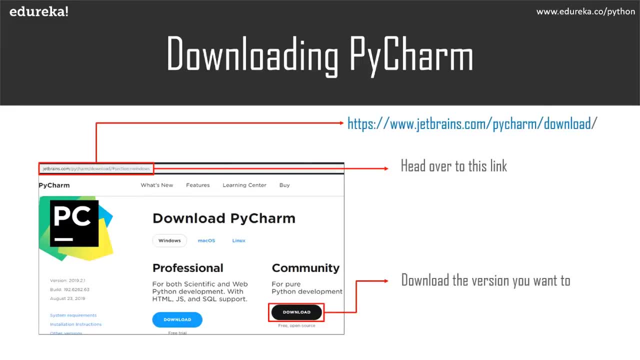 So it is that simple to write your first program in python. Let us close this and move back to my presentation. Now for the rest of the tutorial. I will not be using IDLE, because there are chances that I may have errors and it becomes difficult to debug those errors. 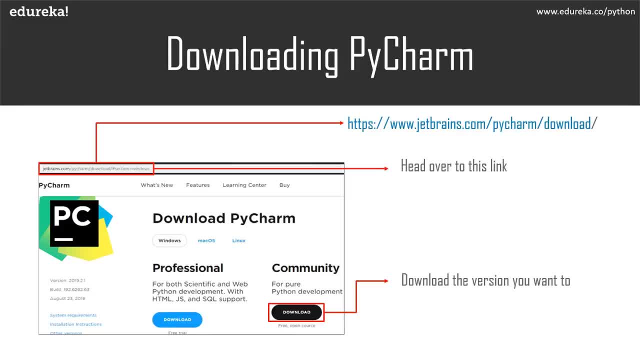 So instead I will be downloading pycharm, which is the ID for writing python files. So head over to jetbrainscom slash, pycharm, slash download and you can download either the professional version or the community version. for the purpose of the tutorial. I will be downloading the community version because it is free. 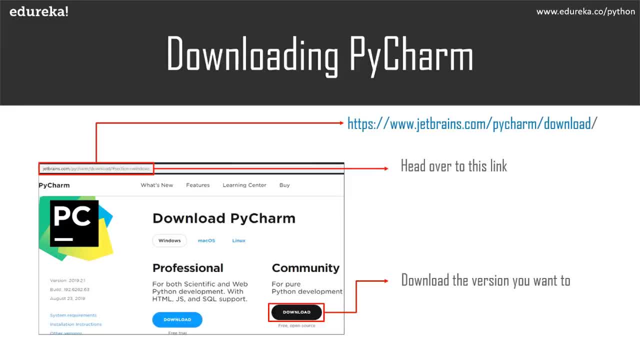 But if you want, you can even go ahead and download the professional version for a certain amount of fee. I already have pycharm installed in my computer, So let us go ahead and see how to work with pycharm and write a few programs with pycharm. 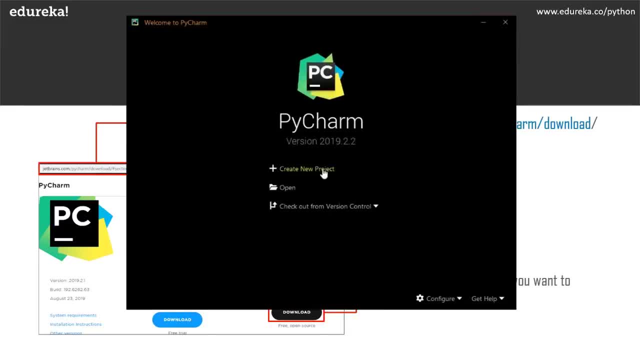 So this is the home page of pycharm. Let us go ahead and create a new project. Let us go ahead and give a name to this project. Let me see it as demo and click on enter or click on the create button over here. 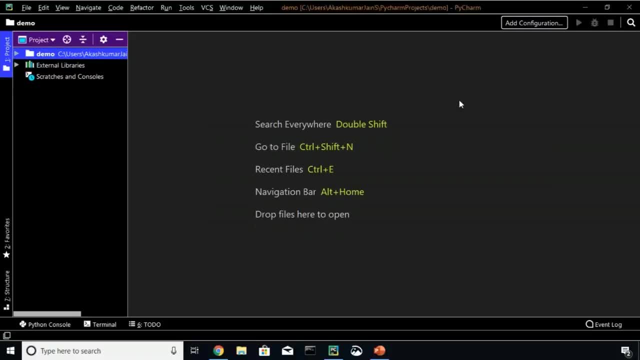 So, as you can see, pycharm has loaded my project. Let me go ahead and show you the files that are in my project. As you can see, there is something called as the venv, which is the virtual environment. This basically takes care of all the installations. 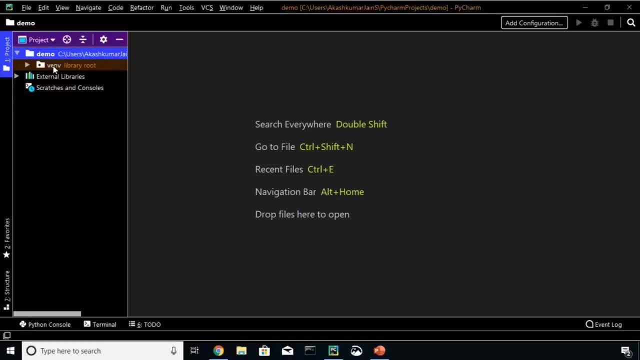 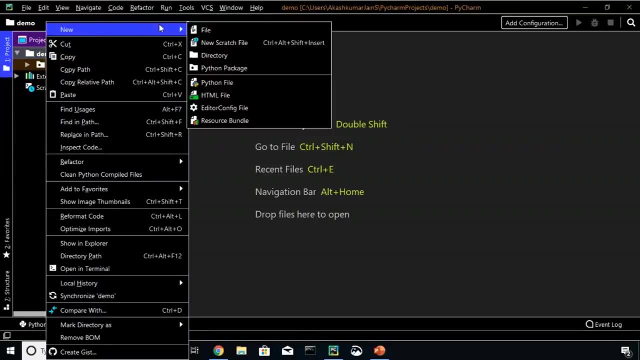 of all the packages that you would need in your program. So let us go ahead and create our first project over here. Let me right click on demo and go ahead on new and python file, and the extension for a python file is always dot py. 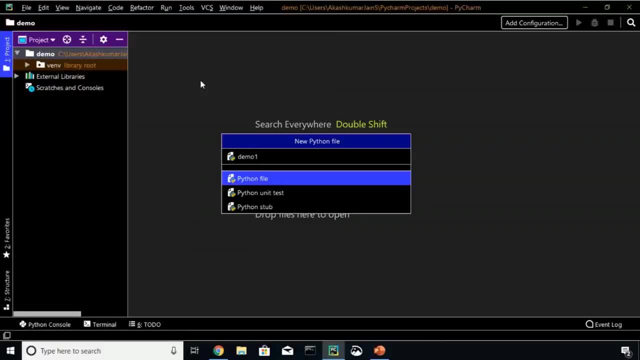 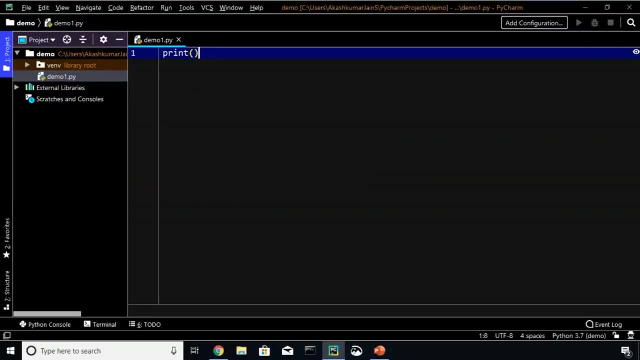 Let me just go ahead and name this as a demo one and hit enter. Let me just write a program over here to get a hang of it. So it was. hello users, Welcome to the Python basics tutorial. Let me go ahead and run this for you guys. 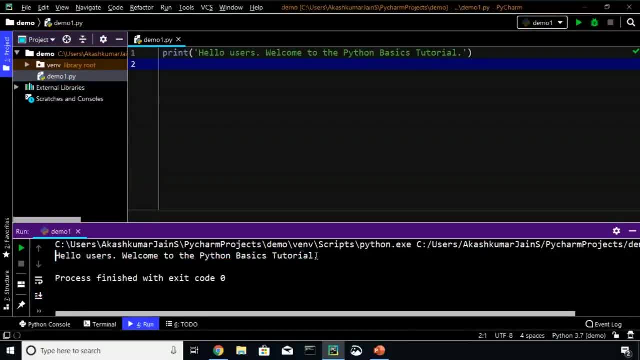 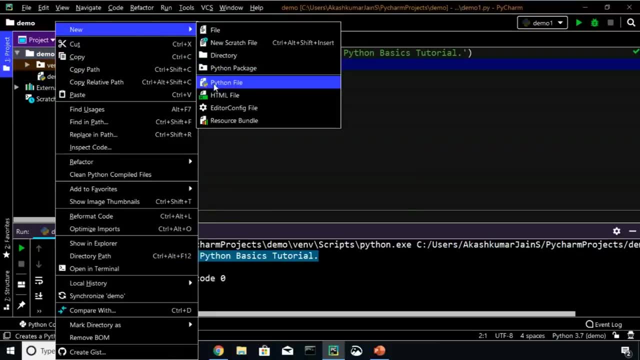 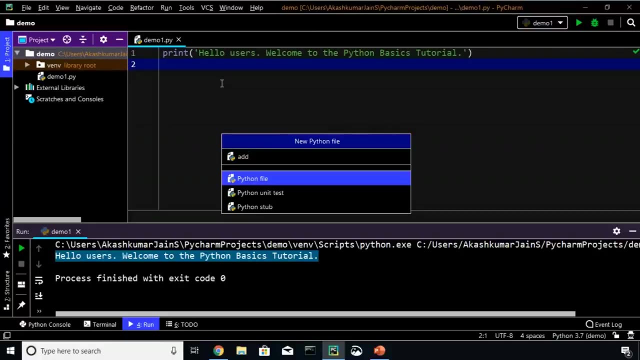 So, as you can see, I have obtained the output. Hello users, Welcome to the Python basics tutorial. So it's that simple. Let's go ahead and create another program and let's say: this will be used to add two numbers, So add, enter. 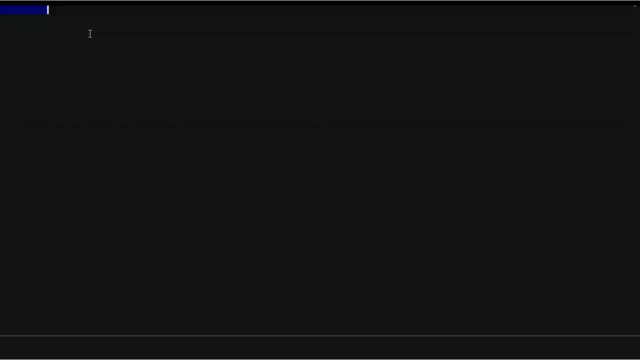 and let me write this in the presentation mode. So let's see. the first line is: a is equal to int of input enter number a. b is equal to int of input enter number b. and let me just write print: The addition of a and b is: 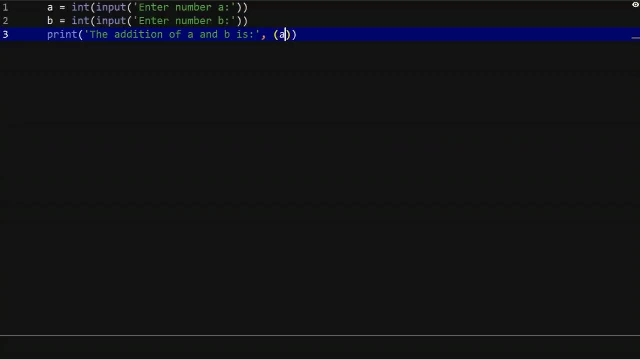 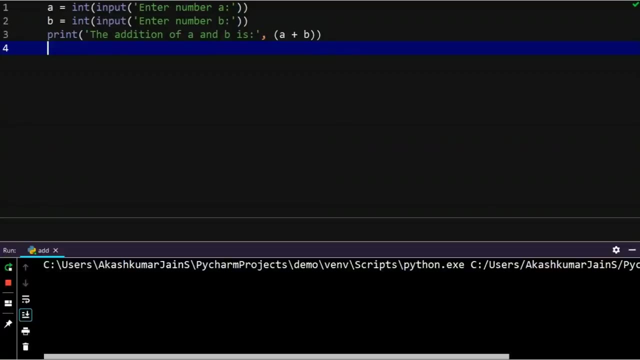 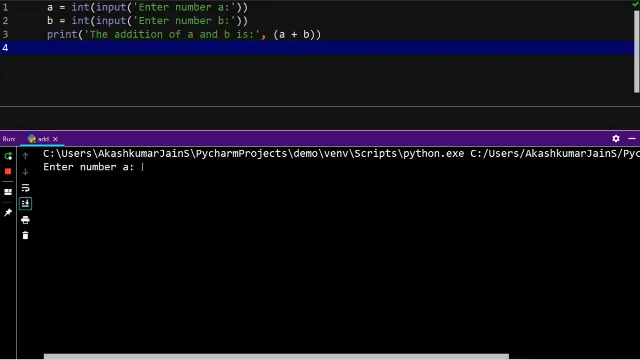 comma a plus b. So let me go ahead and run this program for you guys. So, as you can see, I have two numbers that I have to add over here. So let me just write five and five over here, Let me enter and, as you can see, 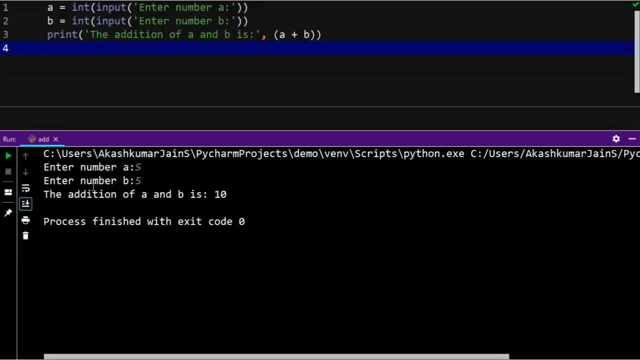 the addition of a and b is 10.. Now, what is the end over here? What does this do? Well, let me tell you how this actually works. So this is basically a function. So whatever is having parenthesis after it. So, for example, 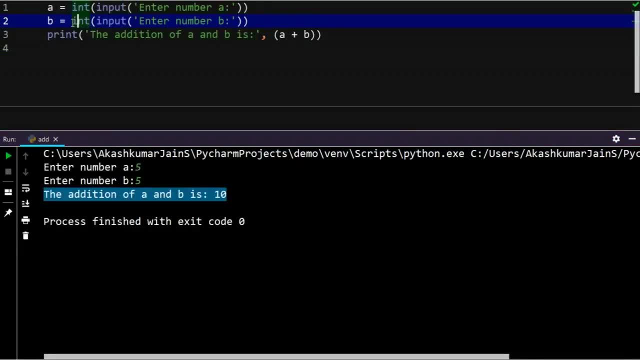 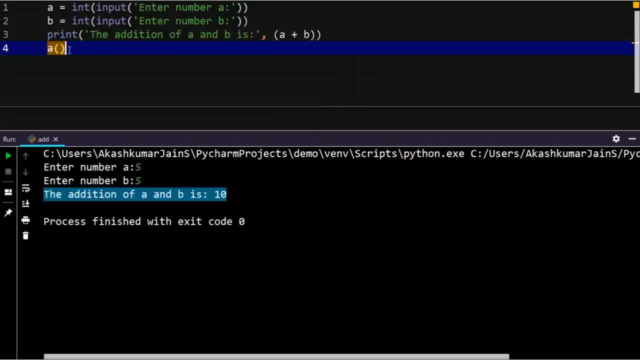 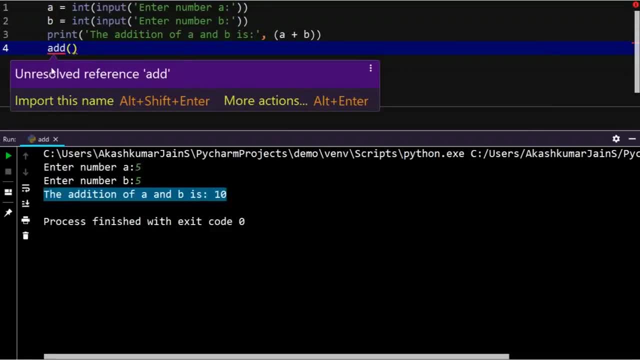 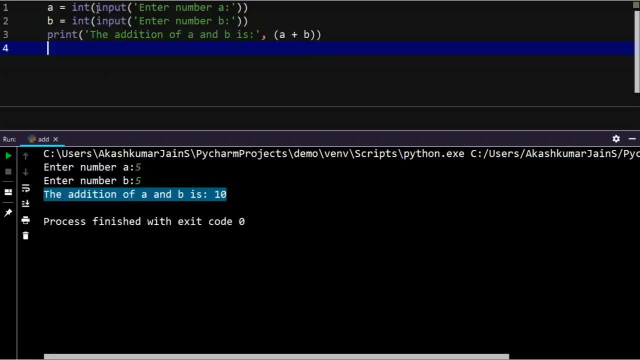 and I have two. You can just call the function accordingly. So now here input is a function and int is a function. So just let me remove integer so that I can show you what exactly happens. So input is used to take the users input and whatever is passed inside will be shown here at the output. 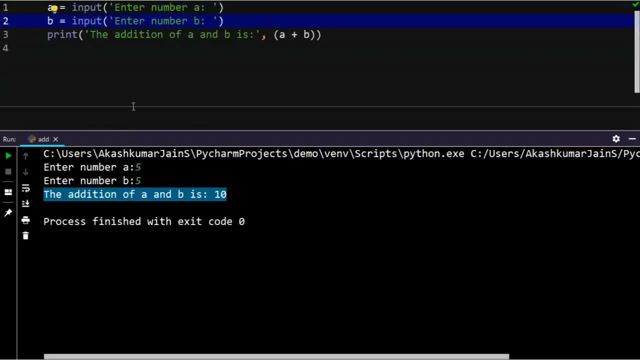 So this? let me give a space so that it's much more clearer. So let me run the program once again. So I have five over here and five. Let me just hit enter and, as you can see that the addition of A and B is 55.. 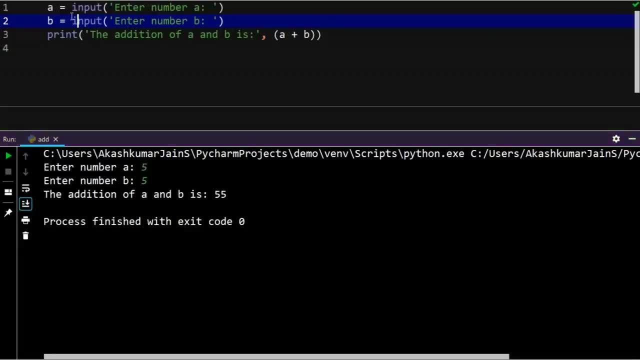 So let me tell you why this happens. basically, the input function, whatever input is taken from the user, is taken as a string or it is taken as a character. It is not taken as an integer or a whole number, which is actually used for addition. So if you add 5 and 5, 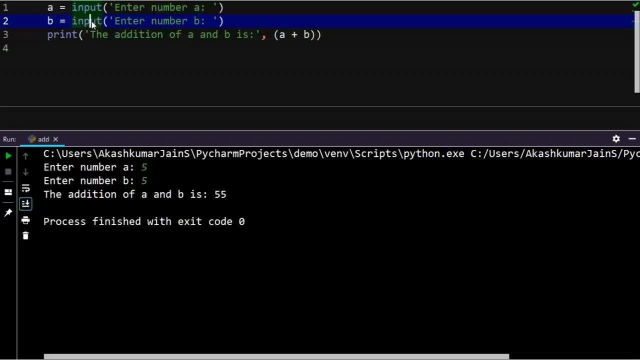 it should be 10, but that is in a number phase. What if those 5 and 5 are characters? So basically, it will be 5 preceding with 5.. That's the reason you have 55 year instead of 10.. So how do you resolve this? 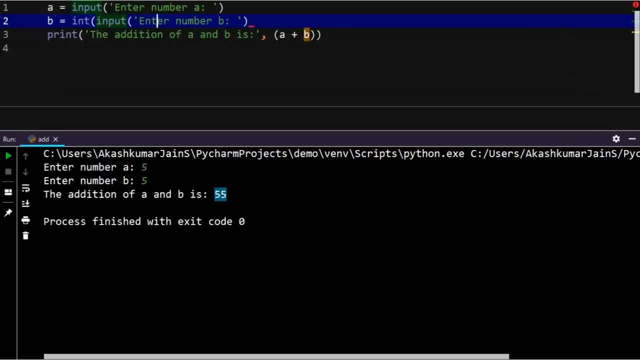 I just call the in function which is used to convert the string. right? these characters that I am passing are string characters, So I am converting the string characters into the integer characters. So let me just go ahead and do this. and now, if I run the program and give the same inputs, 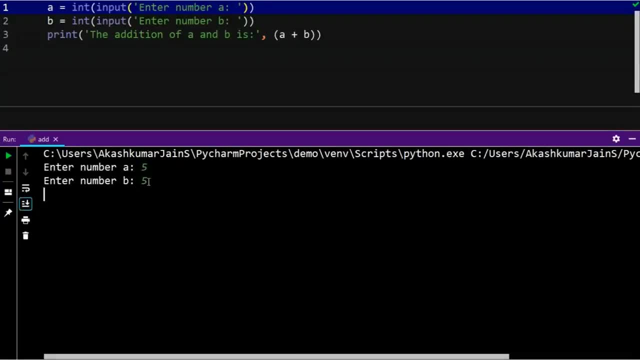 so I give a 5 over here and 5 now what you can see? that I have 10.. So that is basically a simple program that can help you to get used to pie charm. What I am doing here is called as type conversion, meaning that I am changing the data of one type. 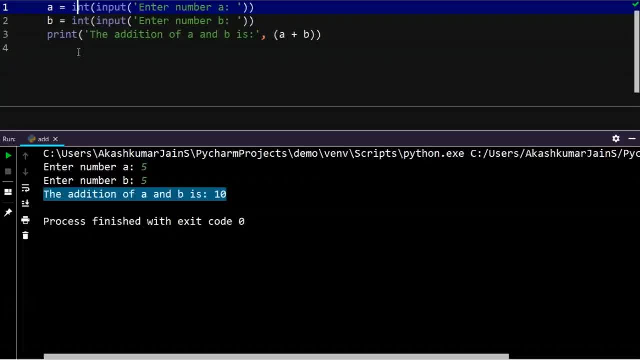 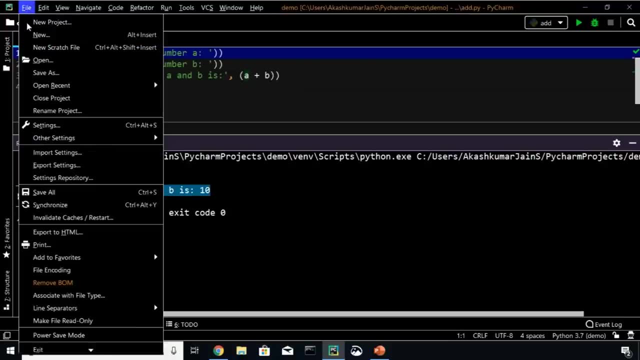 to another data type. So this is basically what happens over here. Let me just come out of the presentation mode and let us move ahead with the next part of our tutorial. So I hope all of you are clear with this. Let me close the project. 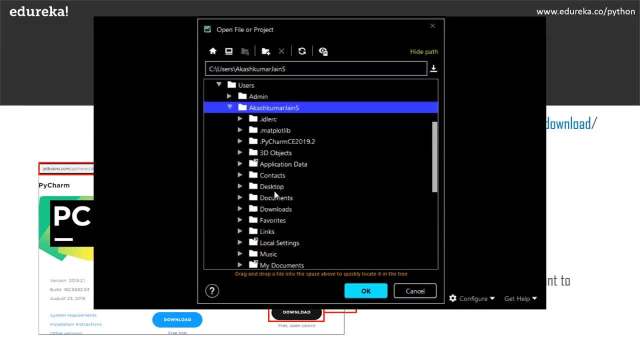 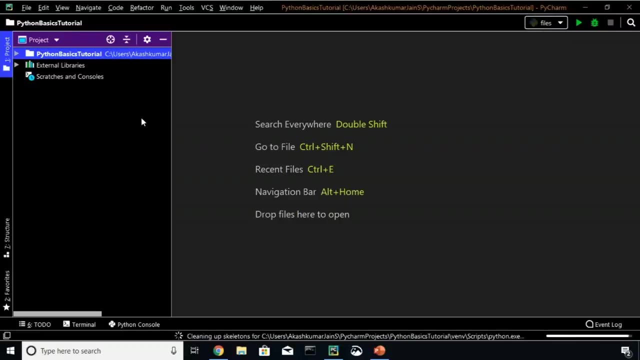 and open up the project that I have ready for you guys, so that it does not waste much time for us in typing. Let me go ahead: pie charm: Python basics open. So, as you can see, I have all the different topics that we will be covering: the data types, file handling. 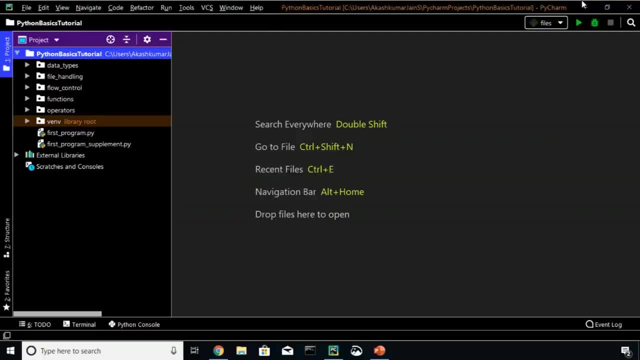 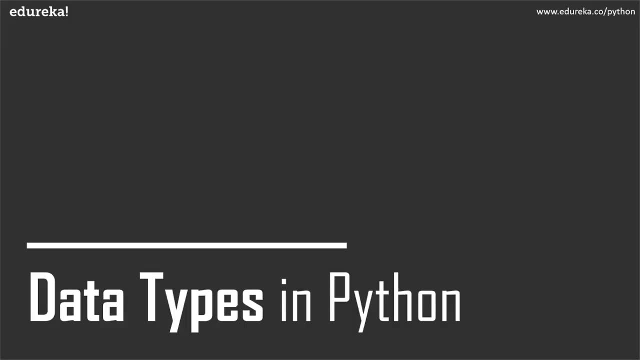 flow, control, functions, operators, all of this. So let me just close this up and move back to my presentation. Now let us understand what are the different data types that we have in Python. We basically have six data types. What do you mean by a data type? a data type is basically: 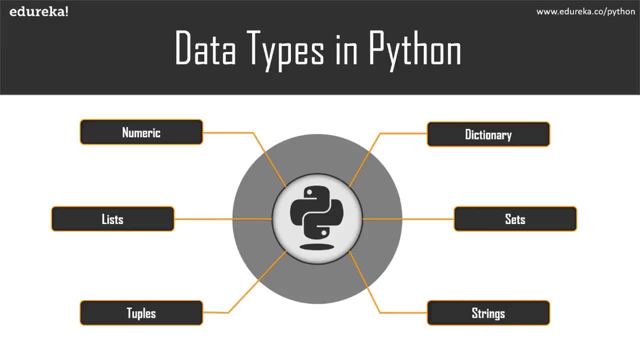 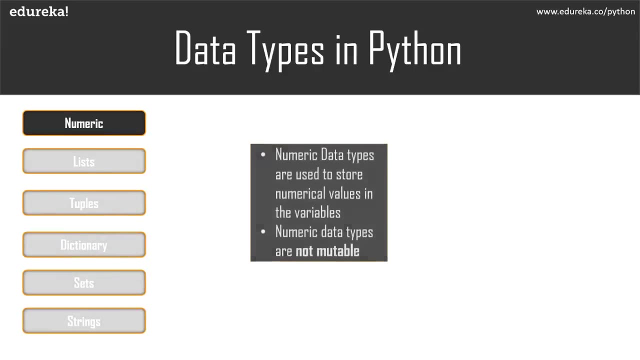 the type of data that you are trying to store in Python. So there are six. So we have Numeric lists, tuples, dictionary sets and strings. Let us go ahead and understand each of these data types one by one. So the first data type is the numeric data type. 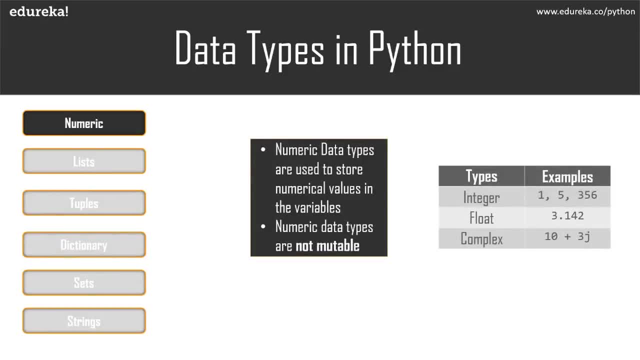 So, as the name suggests, the numeric data type is used to store the numeric values. now you need to know the difference between a value and a variable. So now let me help you understand this with an example. Remember that we had a is equal to 5 or a is equal to 10. 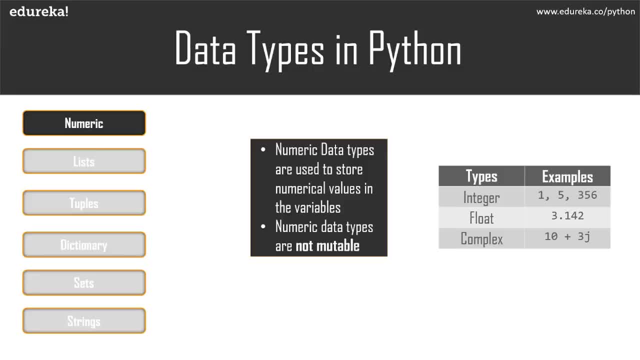 something like that. right Now, a is the variable, which means that it is the name, and the value that I pass to it is the value for it. So, basically, I am giving a name to the value. So the name over here is a and a is the variable and the value. 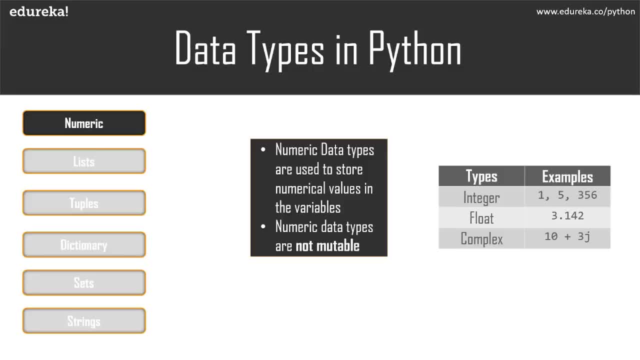 10 is the value that I have given to the variable. The other thing that you have to remember are that numeric data types are not mutable. What do you mean by mutation? mutation is basically change, meaning that the numeric data type cannot be changed. What do you mean by this? 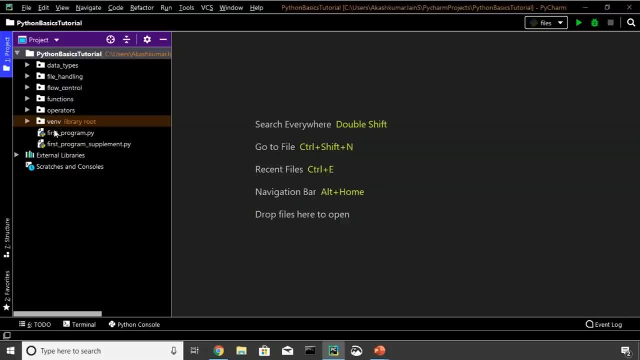 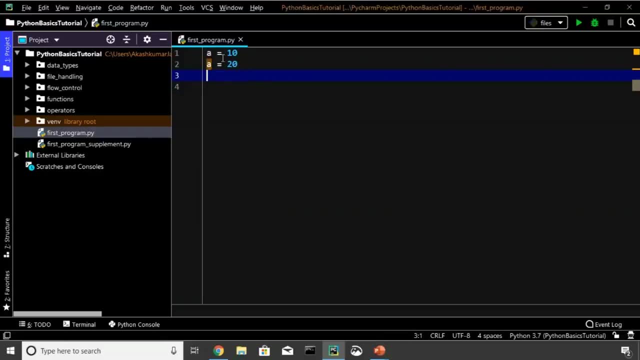 Let me help you understand this with an example. So I have a first program over here now, as you can see that I have a is equal to 10 and I have a is equal to 20 if I print the value of a. and let me just run this. 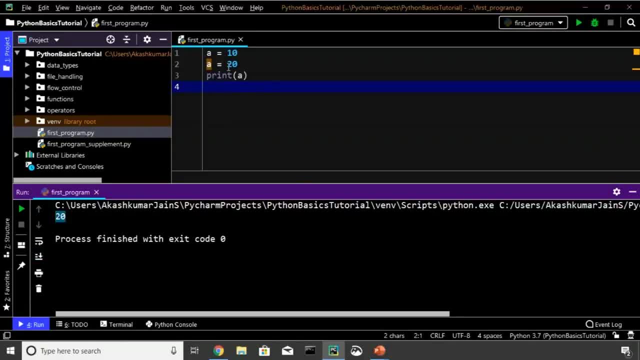 as you can see, I have obtained the output as 20, but what if I wanted to change a off? As you can see, I am getting an arrow over here which says that class integer does not define get item, meaning that I cannot change a particular value inside the 20. 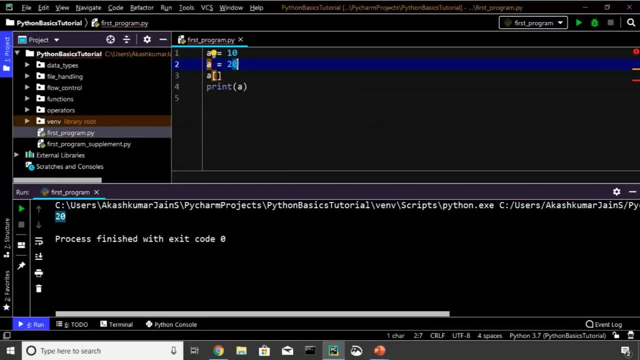 meaning that if I want to change the zero of this to some other value, that is not allowed in python. But if I wanted to change it into 21,, this is allowed in python. So this is what it means by numbers are not mutable. 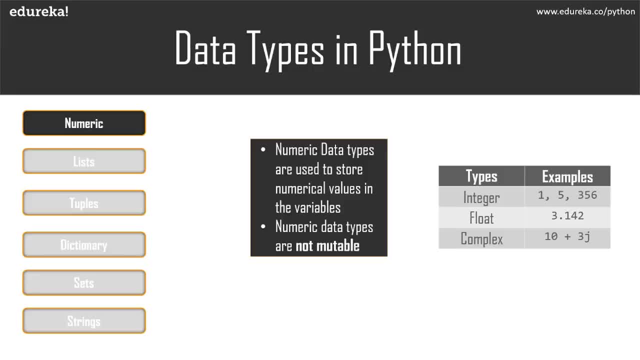 We have three data types in numeric data types. These are the integers, floats and complex. What are integers? integers are basically integers, whole numbers, positive numbers, negative numbers. We have floating values, which are basically the decimal numbers, and we have complex numbers, also in python. 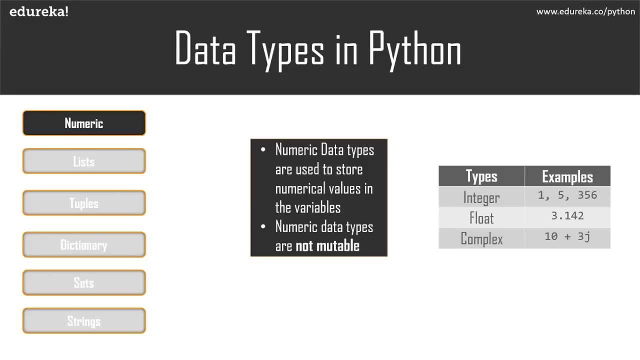 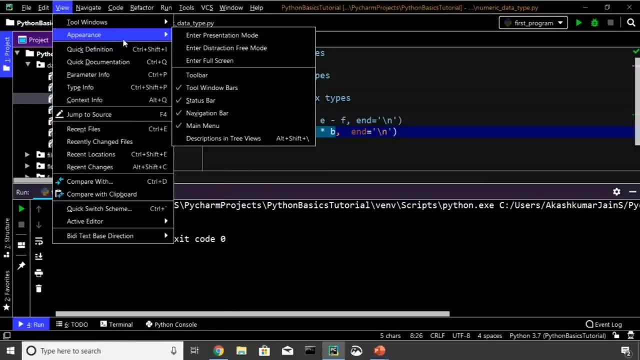 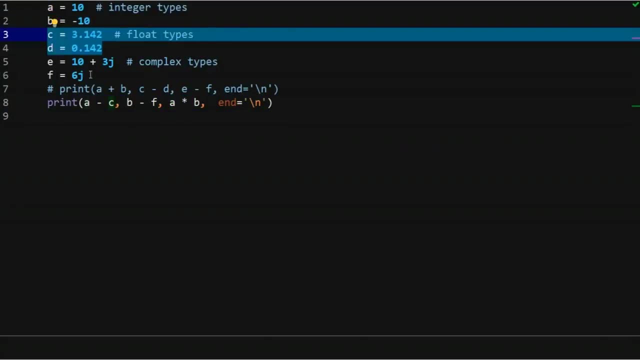 Let us move ahead to the tutorial that I have prepared for you guys- data types- and let's move over to numeric data types. and let me move back to the presentation mode. So, as you can see, I have integer data types, I have floating data types and I have complex numbers. 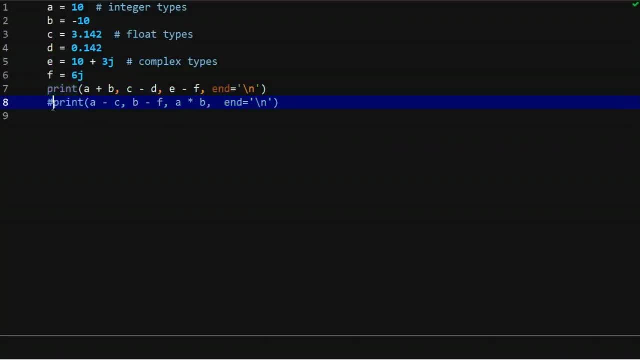 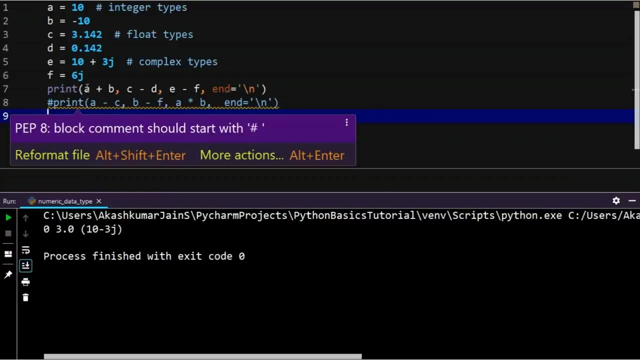 So let me just print it out and let me comment what is not required. for now. Let me run the program. So, as you can see, these are like simple operations that we are trying to perform here. We have a plus B, that is equal to 10 minus 10,. 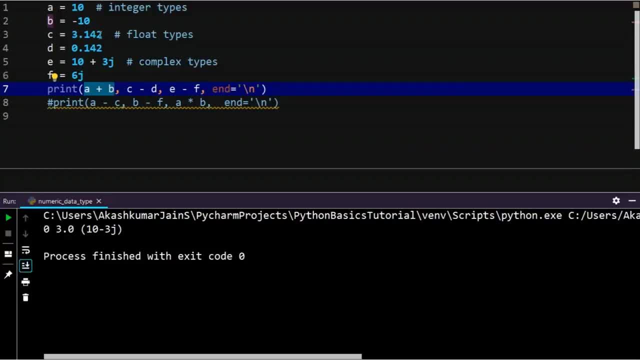 which gives us the output: 0 C minus D is 3.1 for 2 minus 0.1 for 2, which is 3.0, and 10 plus 3 J minus 6 J, which gives us 10 minus 3 J. 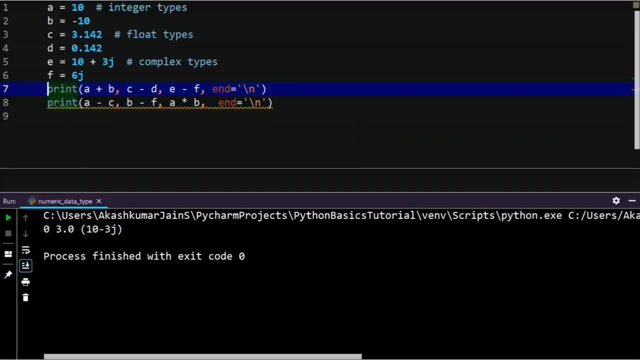 So these are simple applications over here, but the second one is where it is much more important for you to understand. Let me rerun the program Now. as you can see, we have a which is an integer and see which is a floating number. 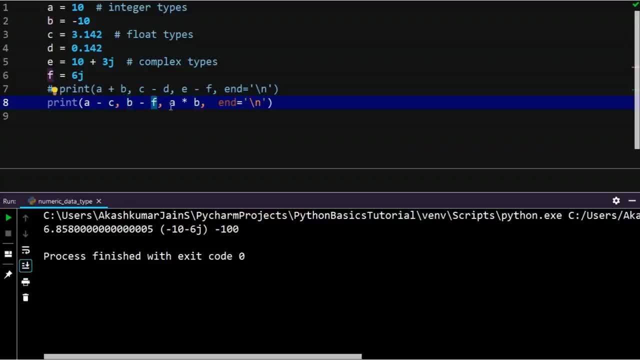 Then we have B, which is an integer, and F, which is a floating number, and then we have a simple operation of multiplication, that is, a into B. but you would think that if it is an integer and if you are working with a floating number, shouldn't it? 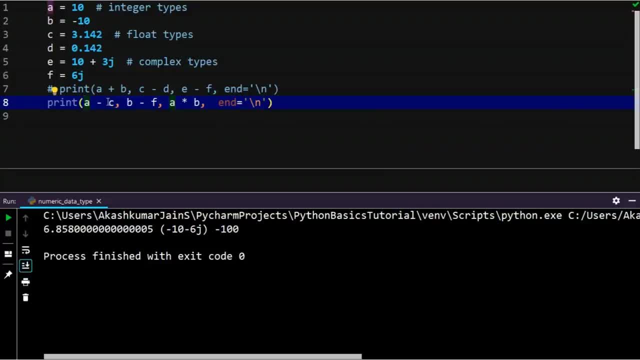 give us an error. Well, that does not happen. Why is that? This is something known as implicit type conversion. If you remember the previous program that we were doing, where we had int of input that was converting the string into a integer number, That's the same thing that it happens. 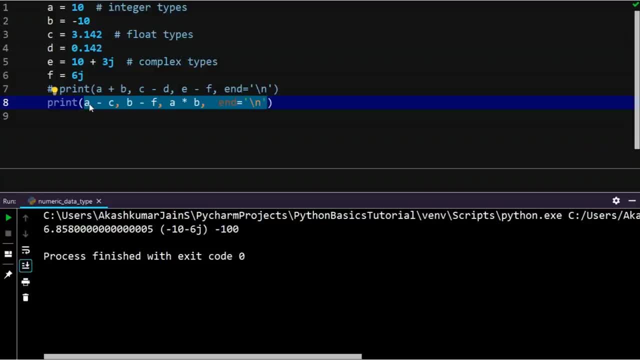 But here we do not need to do it explicitly. This is done internally by Python itself. So it converts the a, which is an integer, into a floating number. So a here will be 10.000 up to the 16 digit part, and then minus 3.142. the same goes over here. 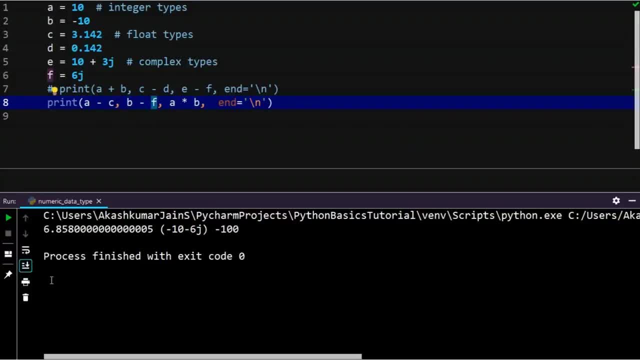 It will be minus 10 plus 0 J, minus 6 J. So that is the reason we have the output as 6.85800 up to 5, and then we have minus 10 minus 6 J, and then the last one is a simple multiplication. 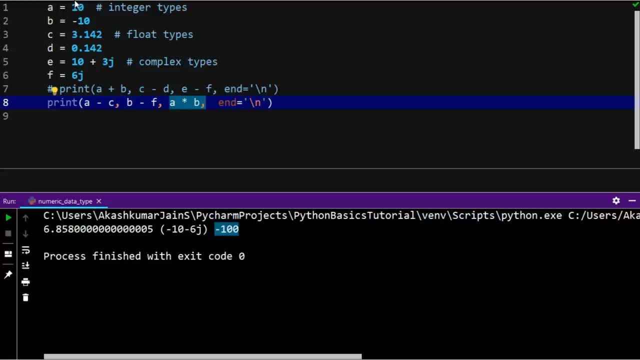 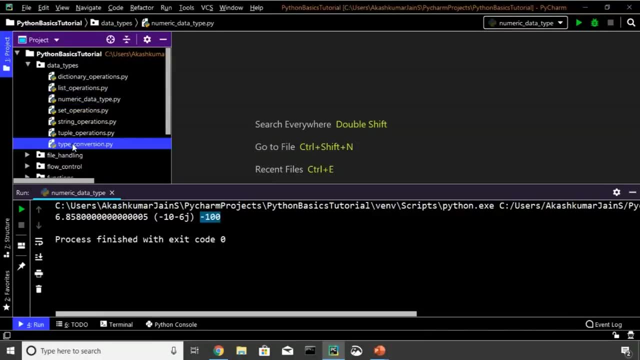 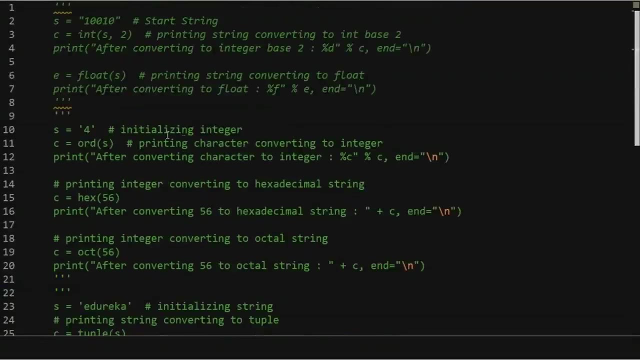 where we have minus 100. So I hope you are clear with the numeric data types. So let us go ahead and close this and understand what are type conversions. as you may remember, type conversions are basically used to convert a data type from one phone to another. 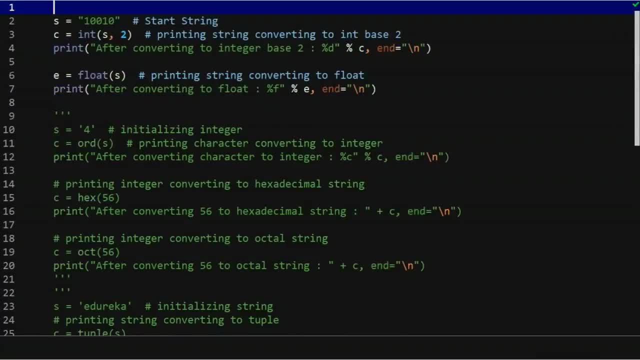 So let me just go ahead and uncomment what is required for now, because if I have the whole program running in a sequence, it becomes really difficult for you guys to understand what's happening. So let me go ahead and run this for you. So I have a string which is 10010. 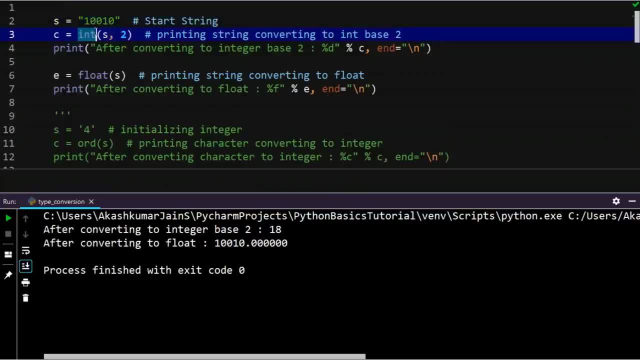 I'm telling that I want to convert it into an integer, and this number that I am wanting to convert into an integer is in the form of a binary number. So that's the reason I get 18, because 10010 in binary is 18. 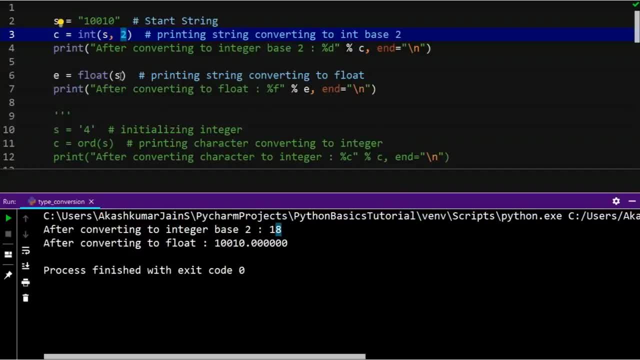 and then we have a floating number which is converting the string that is 10010.. So is converted into a floating number. So it is one zero zero, one zero point, zero, zero, zero. up to how many other numbers? let me go ahead and show you some of the more functions that are available. 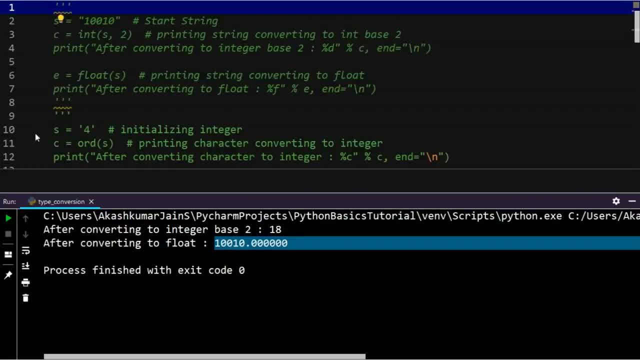 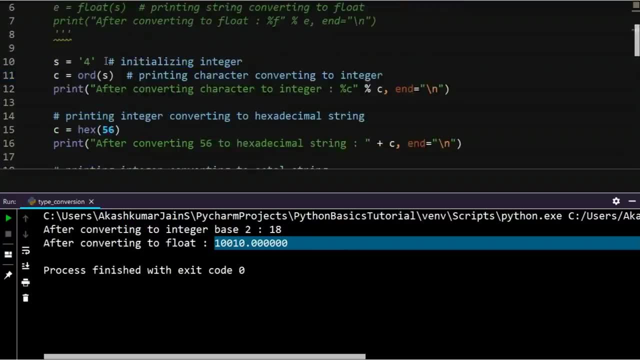 to you which you can use for type conversions. the type conversions that you follow are called as explicit type conversions, and type conversions that python does by itself are called as implicit type conversions. Let me go ahead and run this for you. So I have a string which is having the value 4 over here. 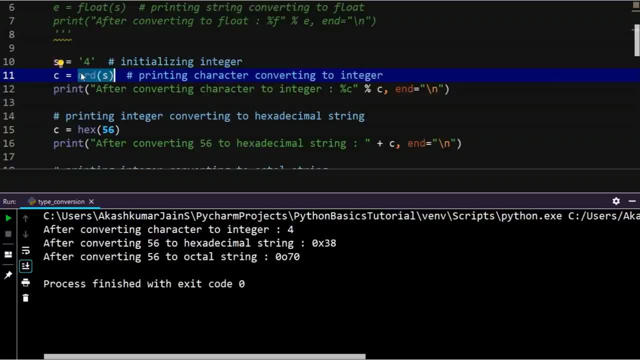 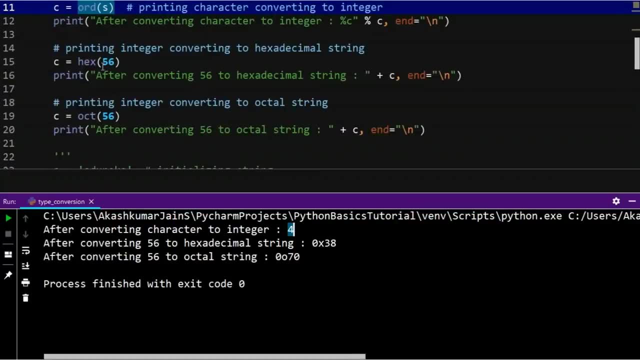 and then I want to convert it Into an integer, which is done using the ORD function. So this is now an integer. now I want to convert 56 into a hexagonal number and 56 into an octagonal number, So that is done using hex and Oct functions. 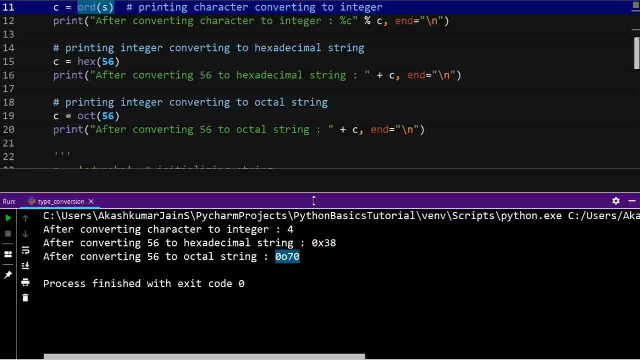 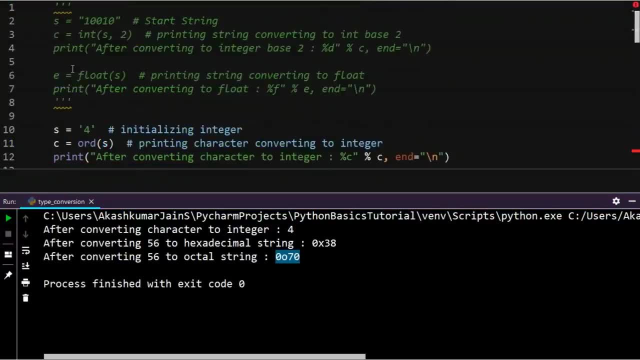 So we have 0 x, 3, 8 and 0, 0, 7, 0, which is 56 in hexadecimal and octal. let me move ahead and show you some more and let me just comment up everything and comment What is not required. 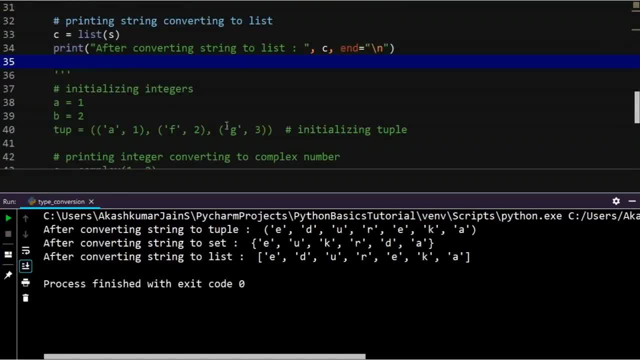 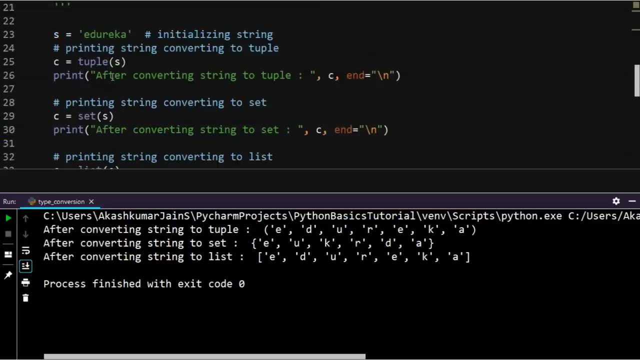 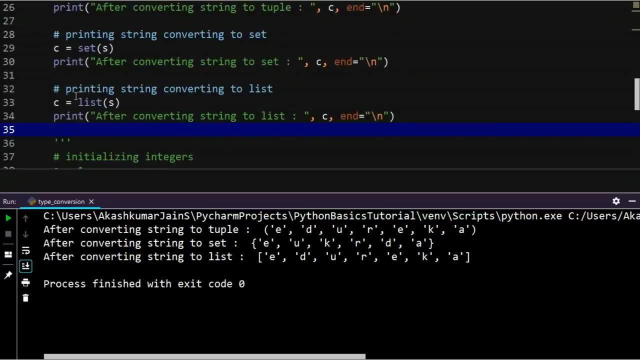 Let me run this. I have a string called edureka and I am converting it into a tuple set and a list. that is what is being done here. I can do this using the tuple function, the set function or the list function. You will understand more of these later in the tutorial. 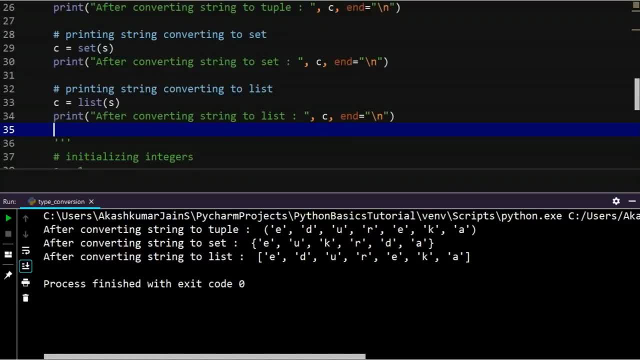 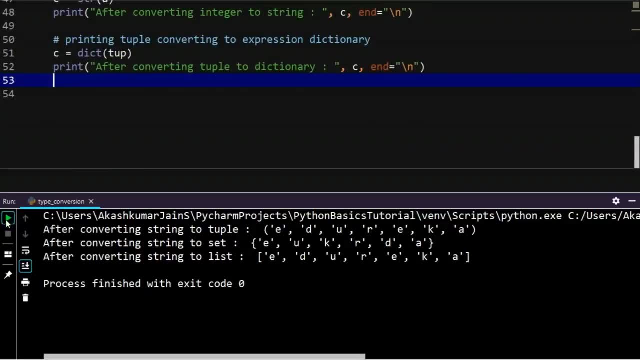 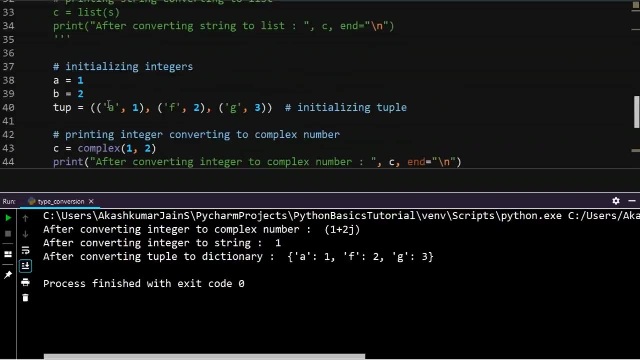 but for now you can just understand that this is how you convert it into. Let me move ahead And run the program. So, as you can see, I have a and B as 1 and 2 and I have a tuple which has a comma 1, F comma 2. 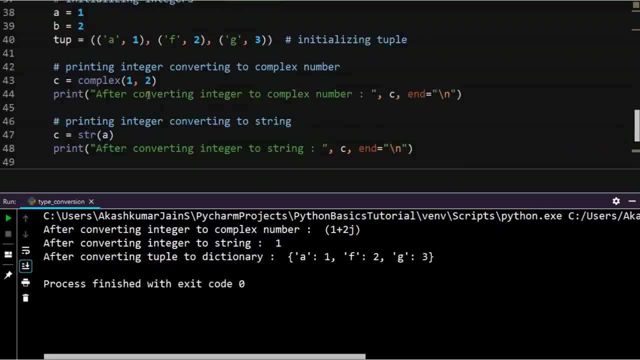 and G, comma 3. if I want to make a complex number, I can use the complex function and pass the values to it. This will give us the output as 1 plus 2g. then I want to convert A number into a string. that is done using the STR function. 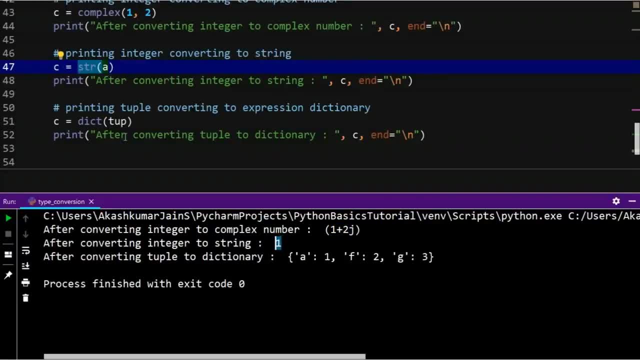 So the number that you have here is basically a string, and then you have the dict, which is used to convert it into a dictionary. So I have a 1, F, 2, G, 3, where a is the key, 1 is the value, F is the key, 2 is the value, G is the key and 3 is the value. 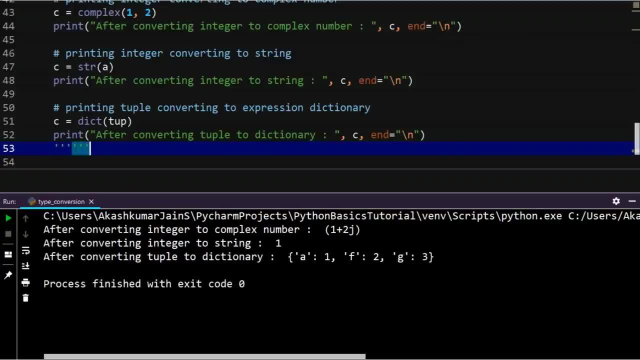 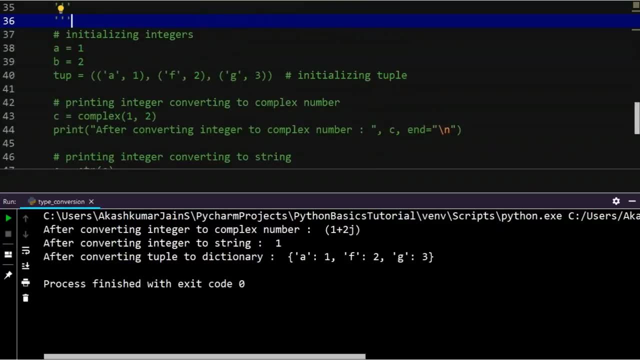 These are just simple examples of how you can use type conversions. Now you may be thinking: Where exactly would you want to use type conversions? This may be better understood if I give you a simple example. think of a company who has the data of their employees in a 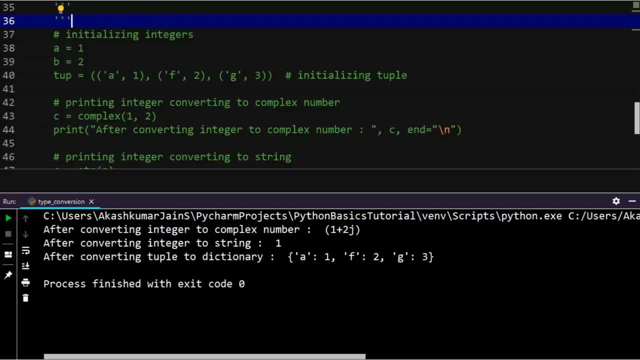 tabular format and all of the data is stored in a string. Now, if you remember from the first part of the pie charm project that we did that, if you do not convert a data, it would be concatenating it into a string, right? 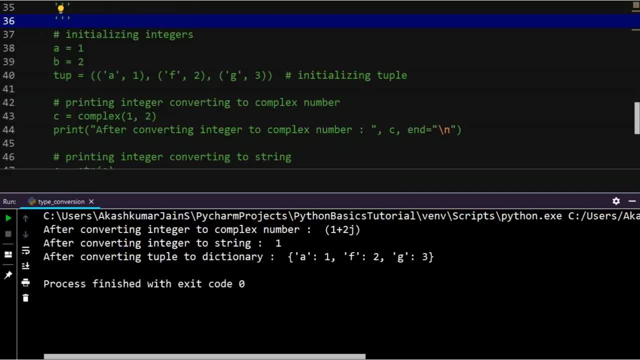 So you do not want that because it may give you wrong output That you would not want. So instead of doing that, you just type converted into an integer or a floating number and accordingly you can perform your own calculations. So that is one simple example. 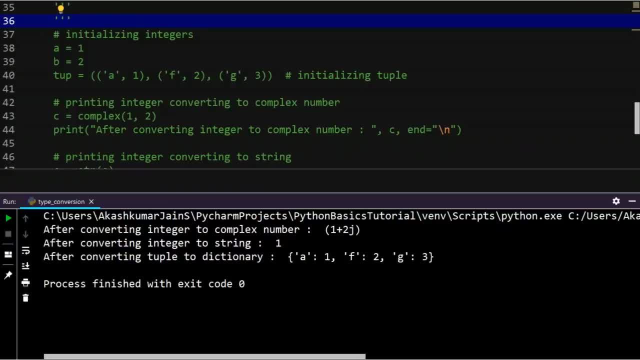 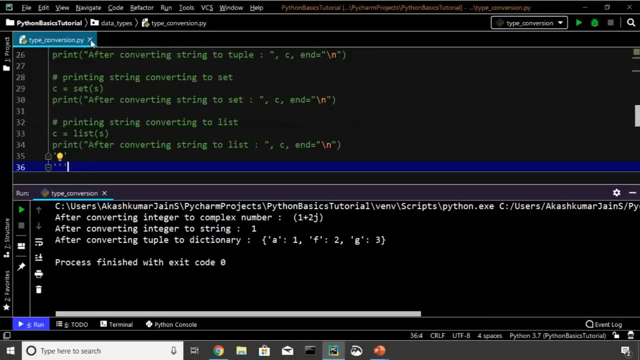 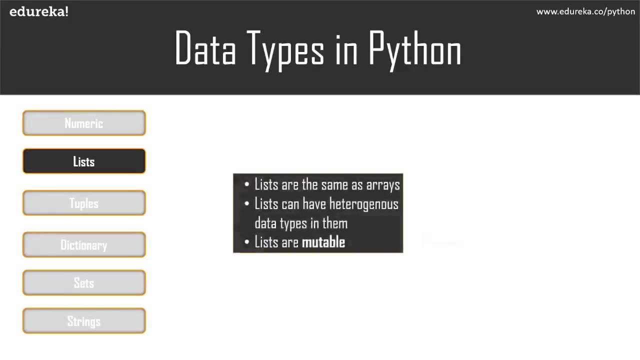 where you would actually use type conversions. There are many, which may depend on the application You're working on. So I hope all of you have understood type conversion. Let us move ahead with the next data type data lists. What are lists? lists are the same as a raise, with one exception. 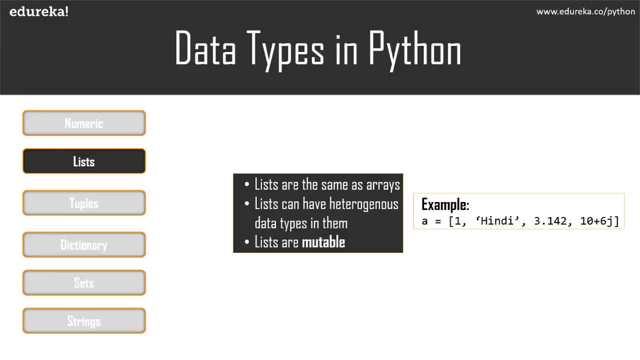 that they can have different data items inside them. I raise would only have a particular data item within them. So, for example, if an array had an integer, it would only have integer values. If it was a floating point, it would only have floating values. lists are not like that. 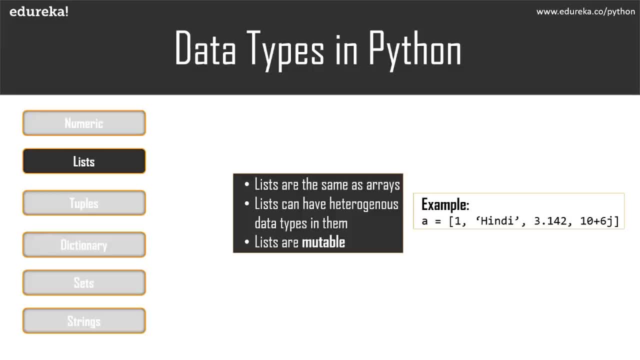 It can have integers, floats, complex numbers, strings, lists, tuples, dictionaries- There can be so many other different data types That a list can hold- and lists are also mutable, meaning that you can change particular items in the list. now for any of you who do not know what arrays are arrays? 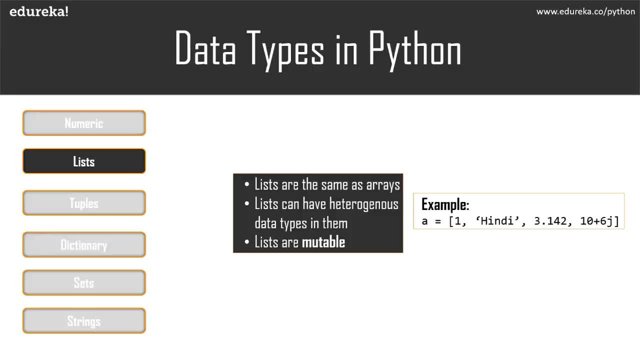 are basically used to construct data structures. Now, what are data structures? data structures are basically the way in which you arrange your data. For example, at home you have a bookshelf where you want to arrange the books in a certain way that is comfortable for you. that makes it much more easier. 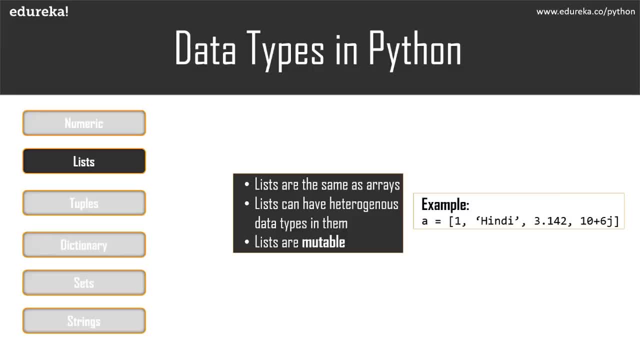 for you to work with. Now, that's the same case with data. data also has to be stored in a particular manner so that it is much more helpful for you to work with. that's the reason arrays are used to make up stacks and queues and so many other data structures. 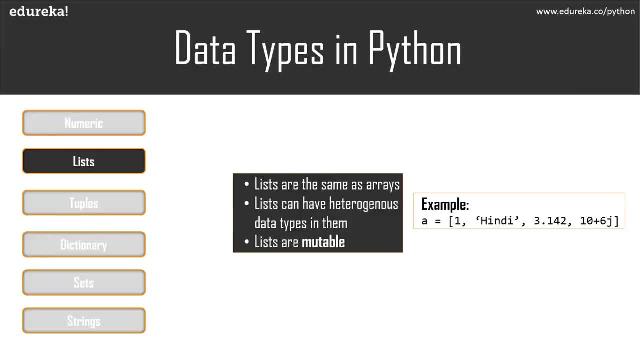 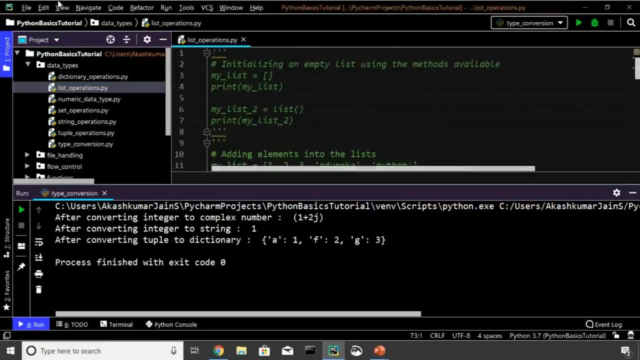 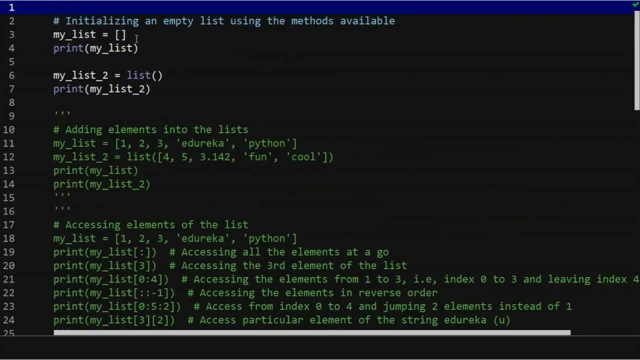 that you have. this is where arrays are used. Let us go ahead and understand lists much more clearer with the operations that I already have prepared for you guys. Let me go back to the presentation mode. So how do you initialize empty lists? It is using square braces. square braces are used to denote. 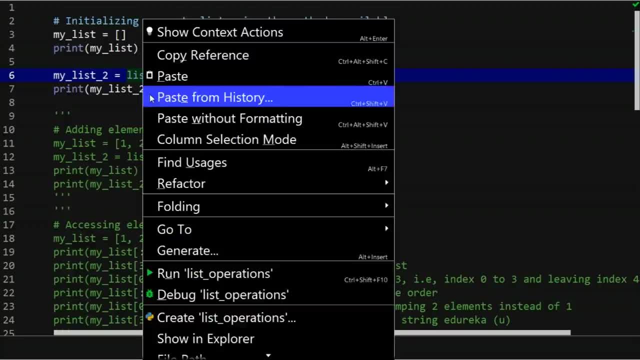 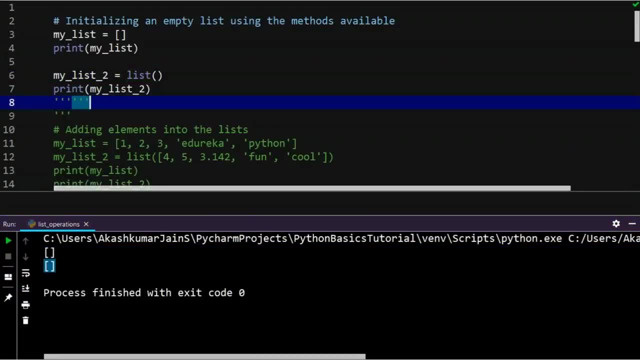 a list or you can do that using the list function. So let me run the program and you can see the code over here. So, as you can see, I have empty lists over here. So that is really simple for you guys to understand. How do you initialize a list? you just add data. 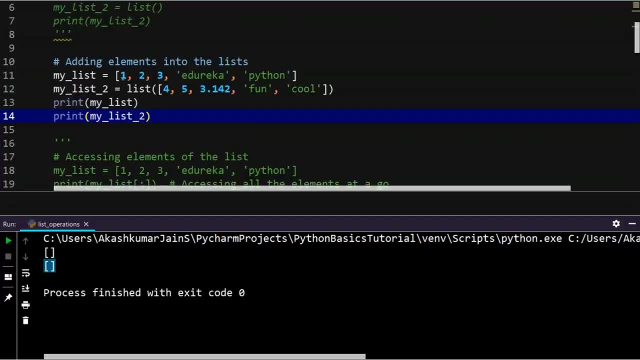 in that particular way. using the square braces, You just have element comma, element comma. accordingly, But if you are using the list function, you have to make sure that you pass it as a single parameter, because if you don't, this will throw an error to you. 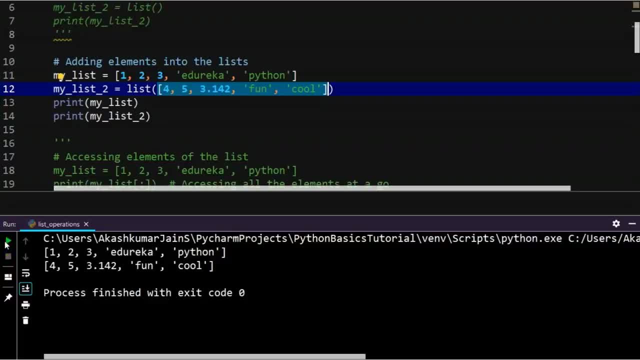 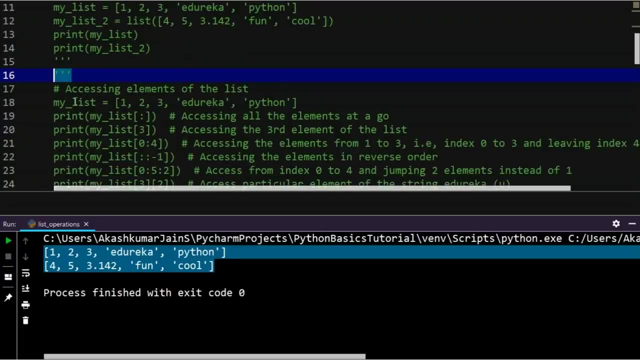 So let me go ahead and run this program. So, as you can see, this is the data that I have in my lists. Let me go ahead and comment all of this. And we have accessing the elements of the list. So how do you access the elements in your list? that is basically. 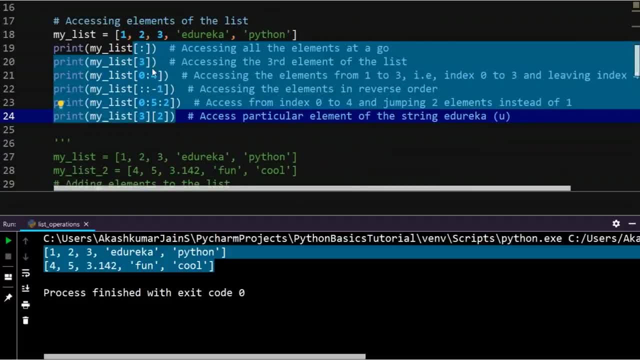 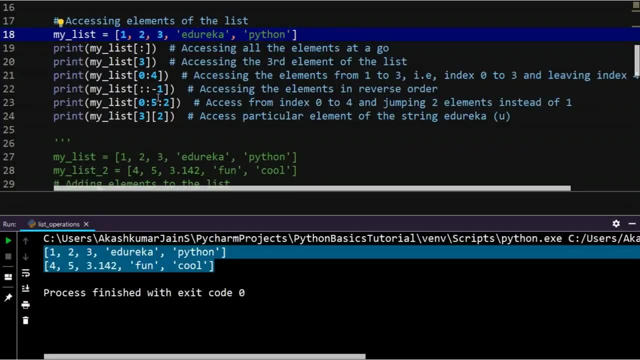 done using Indexes. now it is really important for you to understand what indexes. index is basically the address in which the data is stored. This may be true for lists, tuples and even for strings, So let me show you how the address is stored in python. 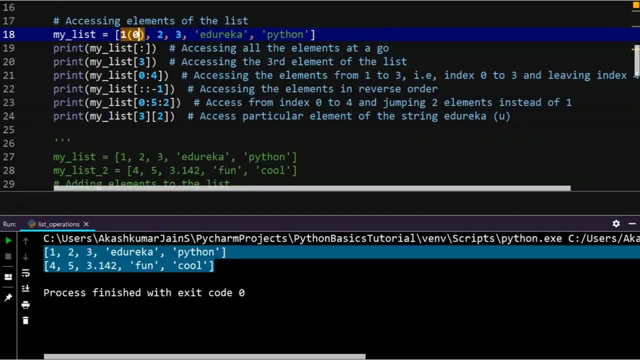 So if I have the element 1, it is stored at the index 0. if I have the element 2, it is stored at the index 1.. So the address always starts with 0. Up till how many ever numbers you have, so this will be 2.. 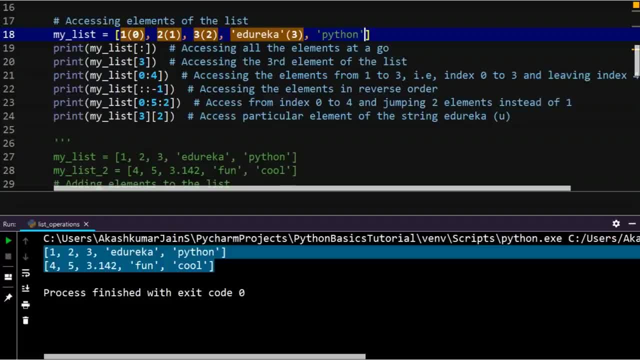 This will be 3.. And this will be 4.. So the address of element 1 is 0, address of element 2 is 1, and so on. There is also something which is called as the negative indexing in python, which can help you to access data from the last. 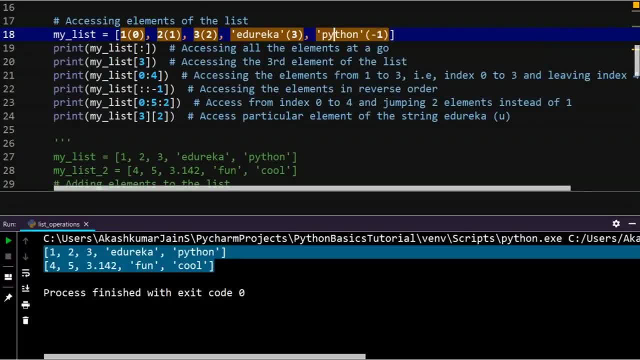 or the bottom part of the list. So how is that? it starts from minus 1? So this will be minus 2.. Sorry, This will be minus 3.. This will be minus 4.. And this will be minus 5.. 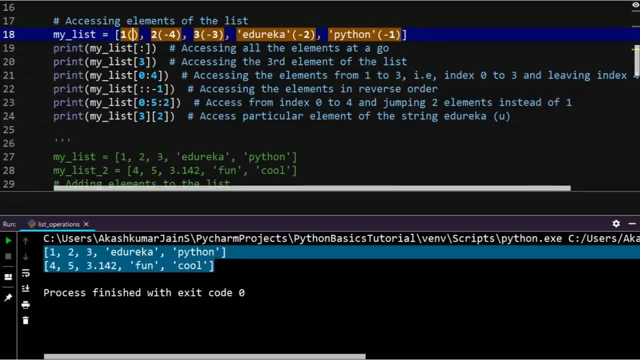 So I hope you've understood what index is. Let me go ahead and just take out all of this. Yes, So now how do you access the elements of the list? It is done using splicing, So basically, what this means Is that you want to particularly print certain parts. 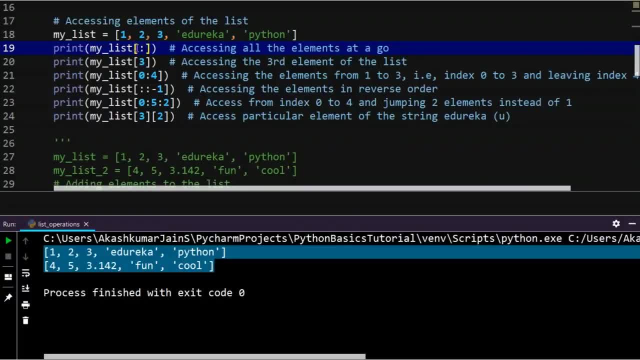 of the list or string or tuple. there is something called as the starting index, stopping index and the skip index. here I have not given anything, So python assumes that I want to print everything, So let me just print out the program for you. Yes, 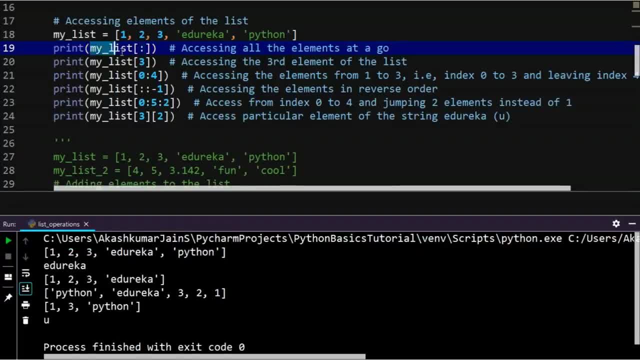 So, as you can see over here, I am just seeing that print of my list. So these are the different methods of how you can access the elements of your string. It's done using splicing, So splicing always has a starting index. 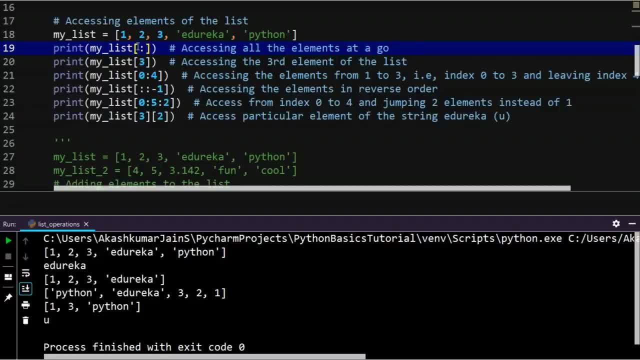 It has an ending index and it also has a skip index. So over here I have not given the starting and the ending index. What this means is that python will automatically think that I want to print all of the data. That is the reason I have all the data. 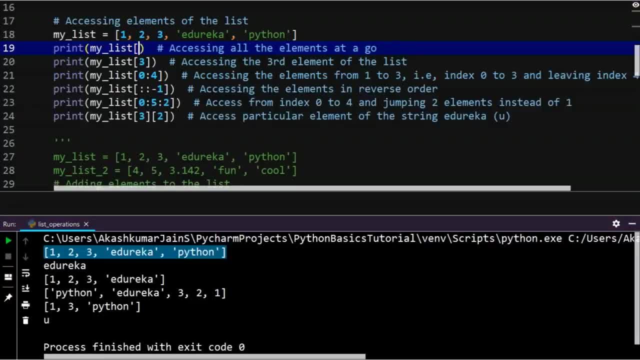 that is being printed over here. If I do not pass this, it will still give me the whole list that I have, So let me just run this again. As you can see, it is printing the whole list, So if I want to access a particular element, 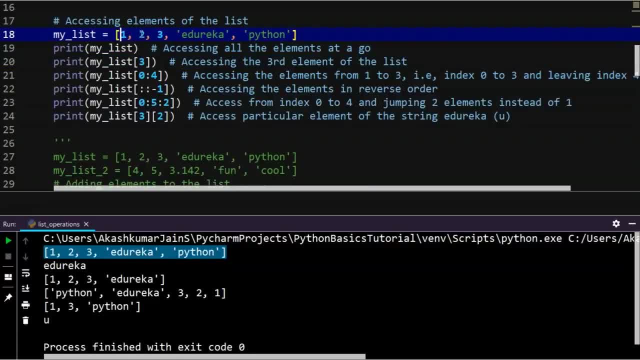 I have to pass the index value of it. So if this was zero, this was one, this was two and this was three. right, I am basically going to print edureka and that is what is being printed over here Now. it is with the starting index and the ending index, meaning 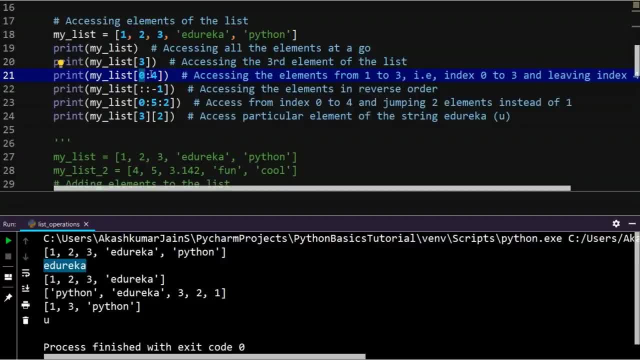 that you have to start from the index 0 and go up to index 3 and you have to exclude index 4. so that is what happens over here. So it is 1, 2, 3 and edureka. that means that I start from index 0. 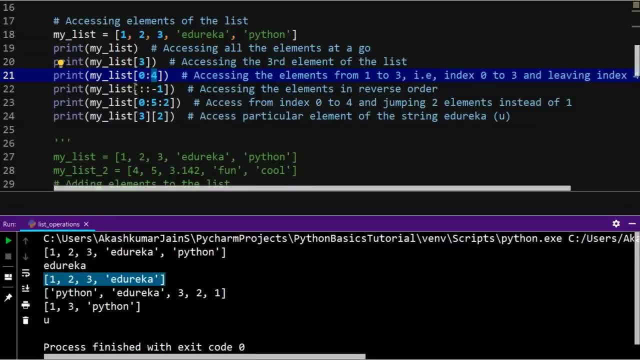 go up till 3 and I skip 4. if I want to reverse it, I do not give any starting or ending index, I just do it from minus 1.. So the list is being reversed over here. So that's what happens over here. 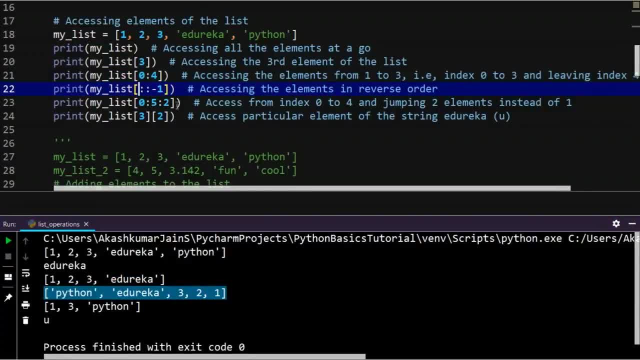 As you can see, next is something called as the skip index. right now, I start from 0, go up till 5 and skip two elements, Meaning that I print one, I skip 1 and I skip 2 and I print 3, I skip 3, I skip edureka and I print python. 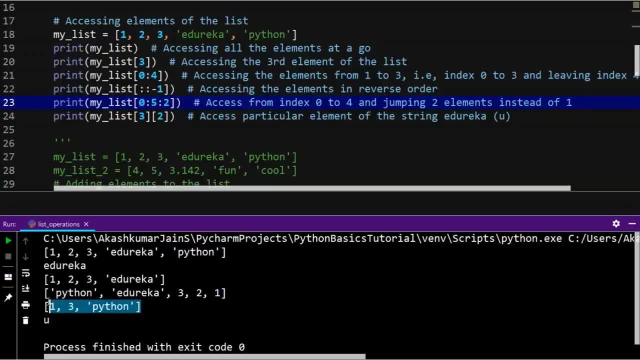 So that is what happens over here. As you can see, that is how you have obtained the output. next is the third element and the second next. the next is: I can also access particular elements within the elements. So, basically, what I am saying over here is that I want to. 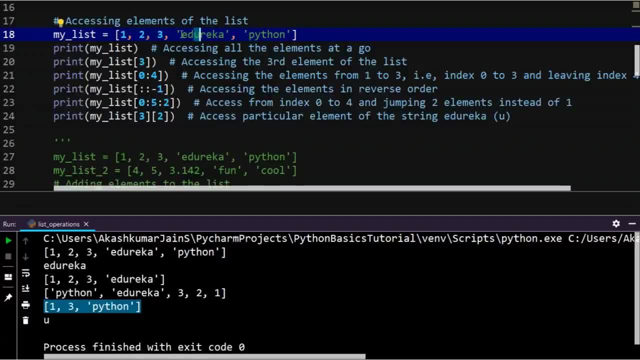 print you. How do I do that? I know that edureka is at index 3 and I also know that you is at the index 2, so I just add that over here. So I have 3 and 2 and that's the reason I have you. that is. 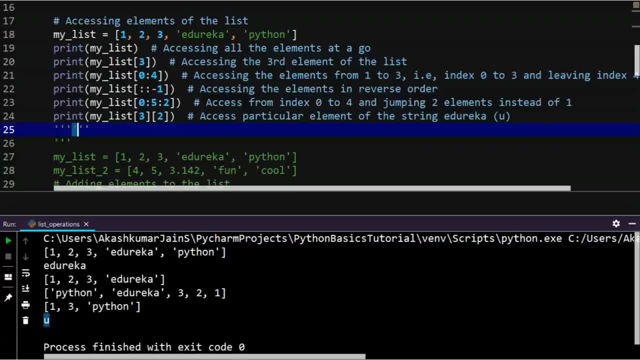 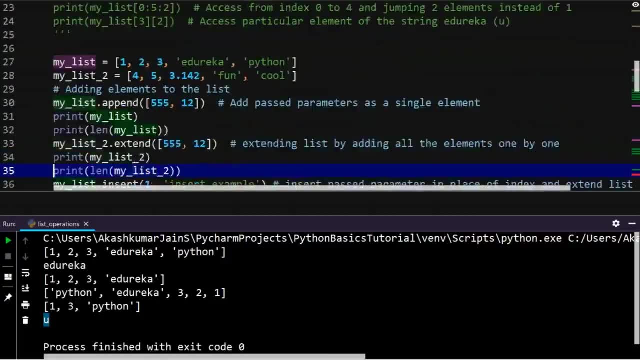 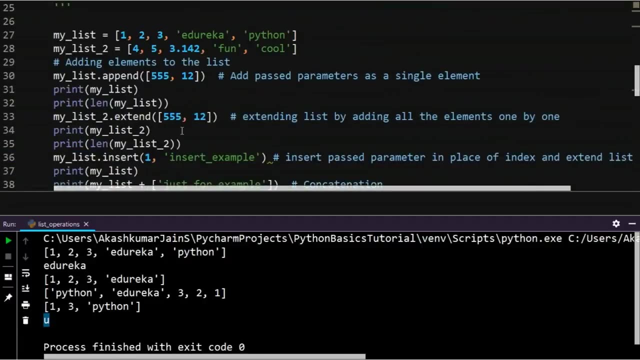 being printed over here. So I hope you have understood what is indexing and how you can access the elements using splicing and indexing. Let us move ahead and add data into the list. How do you do that? You do that using the append function, the extend function. 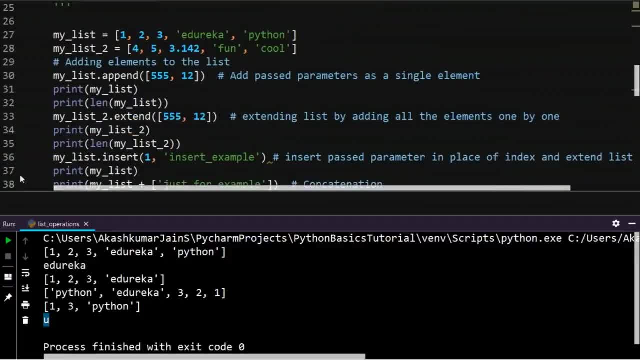 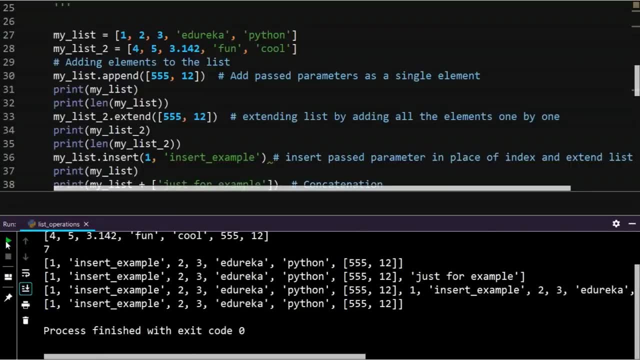 And the insert function. So let me just go ahead and show this to you. How is how it is being done now? So the append function as the element at the end of the list. the extend function also adds the element at the end of the. 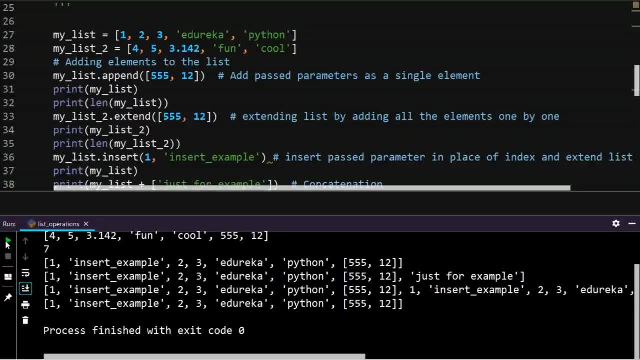 list. So what is the difference between them? Well, the difference between them is that the append function adds it as a particular element, It adds it as a single element. The extend function does not work like that. It adds all the elements one by one. 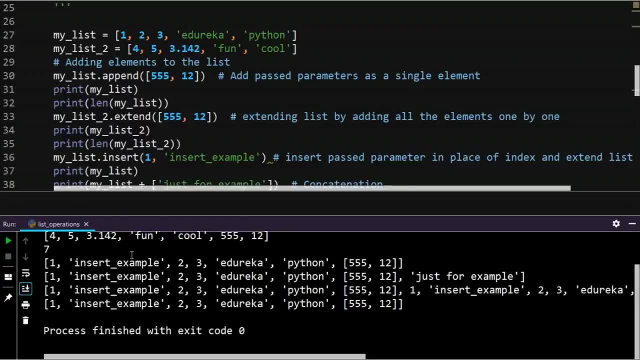 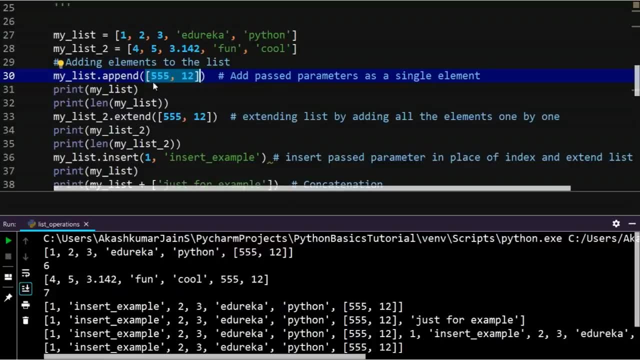 Whereas the append function just adds it as a single element. That's the reason. if you go over here, you can see that triple Phi and 1, 2, which is being passed actually as a list, is added as a list itself. So I have 1, 2, 3, Edureka python and I have triple Phi and 1, 2. 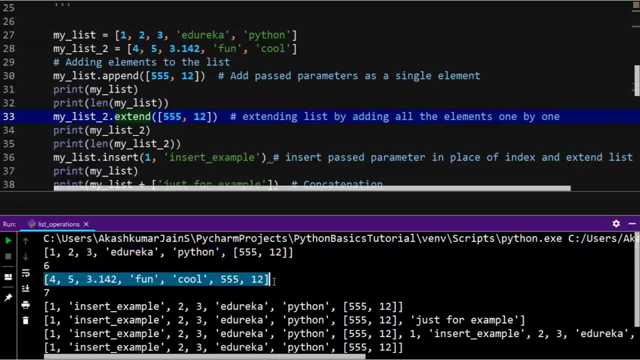 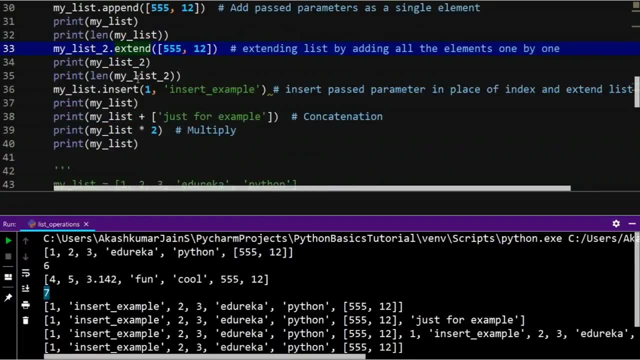 but whereas in the extend function I have triple Phi and 1, 2 independently, and that's the reason I have 7 as the length of the list. The length of the list is basically to show how many elements are there in the list. And then I have the insert function which takes the index. 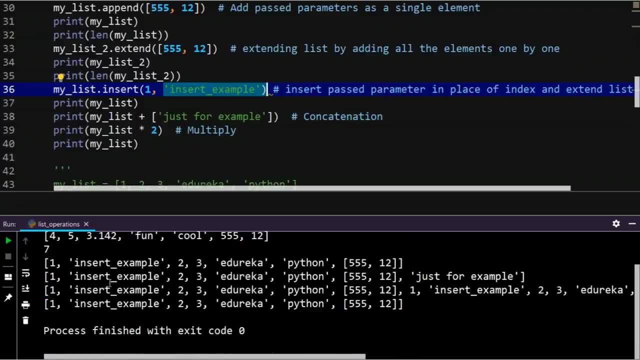 at which I want to insert the particular data as the reason over here. If you can see, I have one insert example and accordingly the data is not deleted when you use the insert function. The next ways are to use the concatenation and multiplication, but they do not affect the actual data of the list, as you. 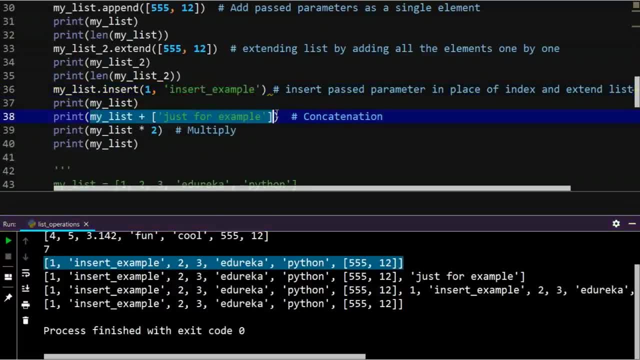 can see over here, I just have printing of my list, But if I was not printing it it would actually change the data of it. But since I am using it in the print function, the data will not be changed. So, as you can see over here, I have one accordingly and just. 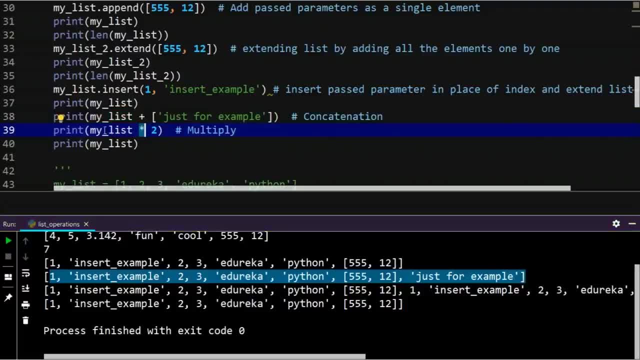 for example, and then multiplication is multiplying the list accordingly to the number you have told it to be multiplied with. so the whole list will be multiplied 2 times. and then, just to show you that if I am printing all of this, it does not change the actual data. 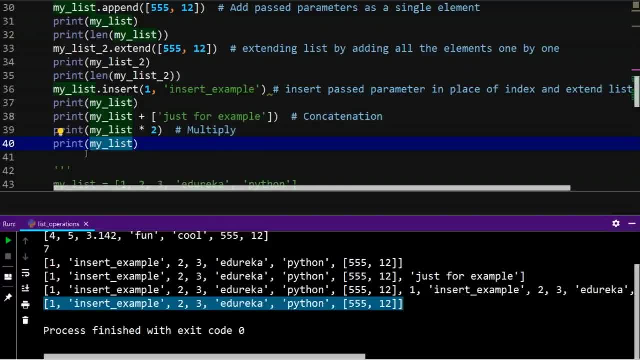 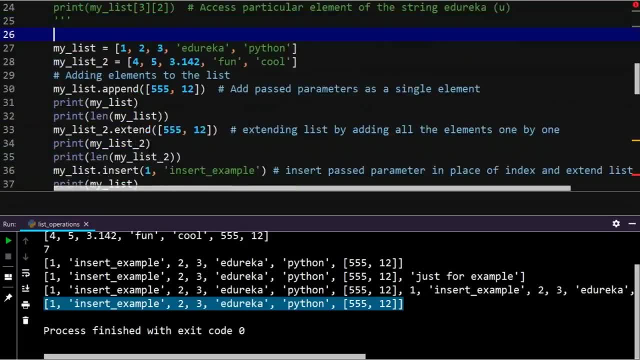 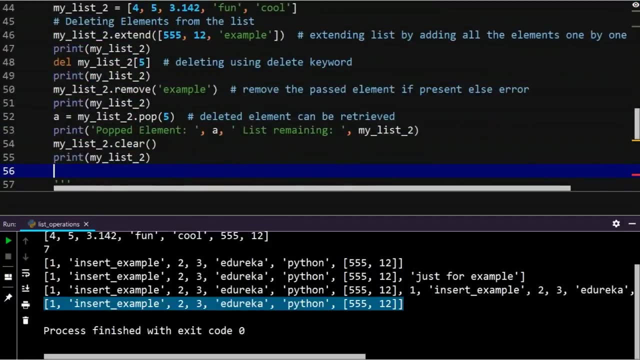 I have printed my list and you can see that my list is unaffected. So that is basically how you can add elements. Now let's move ahead and see how we can delete elements from the lists. Let me go ahead and run the program. 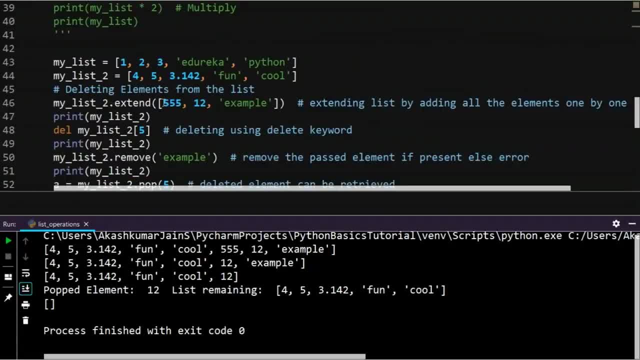 As you can see, I have two lists and I have extended my list using triple five. one to an example. one way of deleting is by deleting it using the del keyboard. I just say delete and pass the element that I want to delete and it will be deleted. 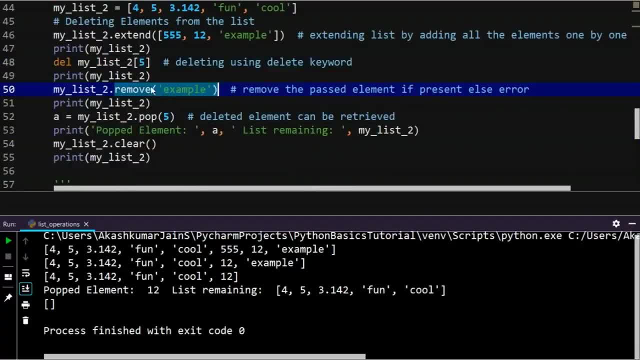 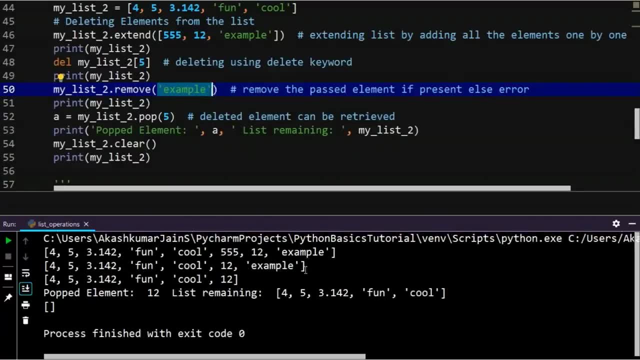 The next one is using the remove function, So I just pass the element that has to be removed from the list and accordingly, that will be removed. So that's the reason here. as you can see, triple five was deleted using the del keyword and example was removed using the dot. 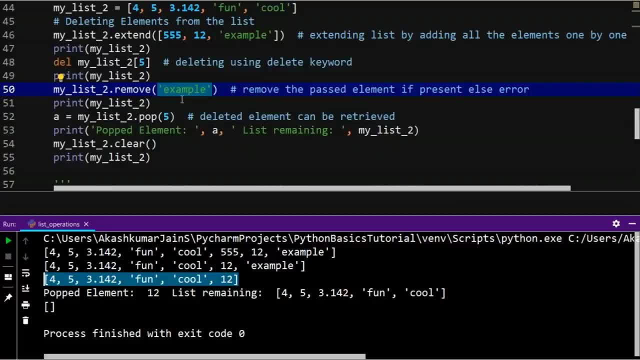 remove function. The next is the pop function. the pop function and the delete function are basically doing the same thing, with one exception: The delete keyword does not return anything, whereas the pop function returns the value back to you, so you can use it accordingly to how you want. 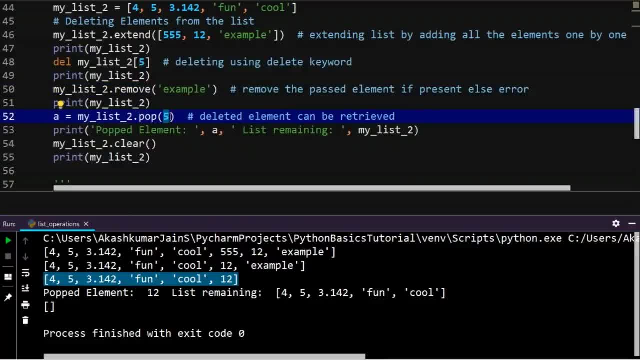 So I'm just seeing that pop the element which is at index 5.. That's the reason the pop element over here is 12 and the remaining list is 4, 5, 3.1, 4, 2, fun and cool. And then the last function is the clear function. 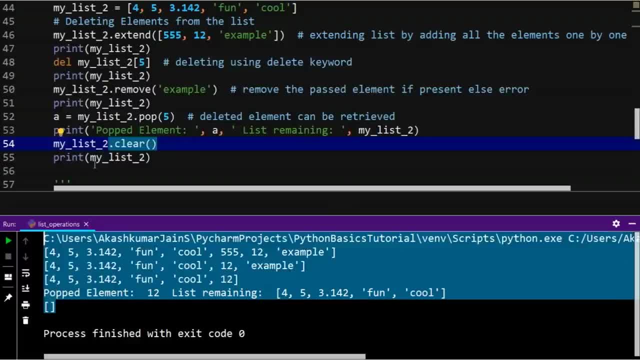 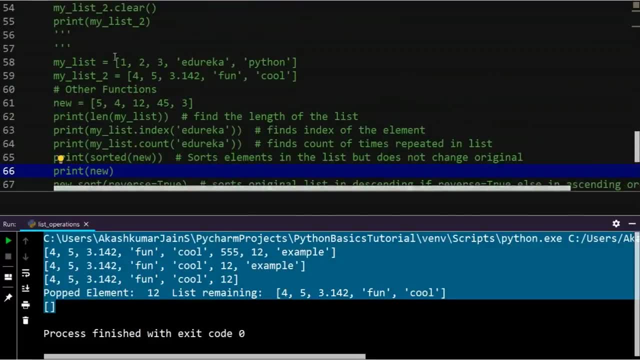 which returns an empty list. So I hope you've understood what are the different ways that you can delete the data from your lists. Let's move ahead to just see the different other functions that are there in Python, If you remember, the length function is used. 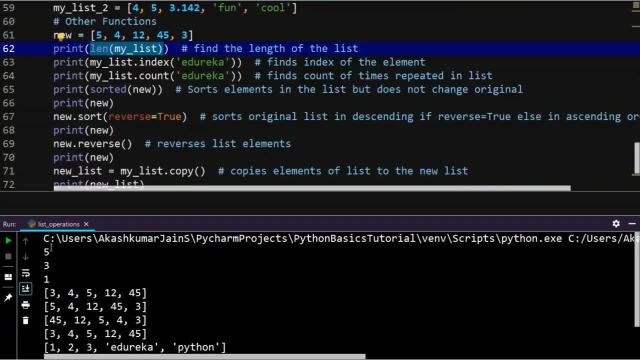 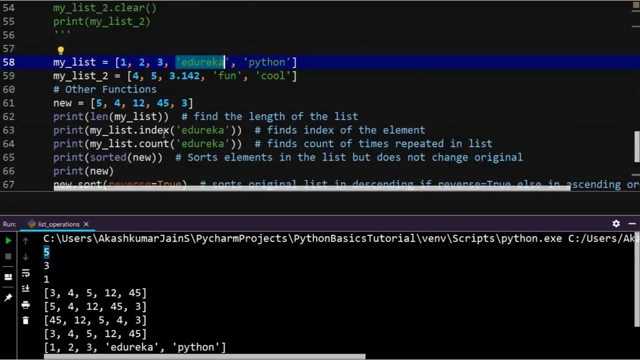 to return the length of the function, and that is the reason we have obtained 5 over here. The next is the index function, which is used to return the index where this particular element exists, and this element exists at 3.. That's the reason we have 3 at the output over here. 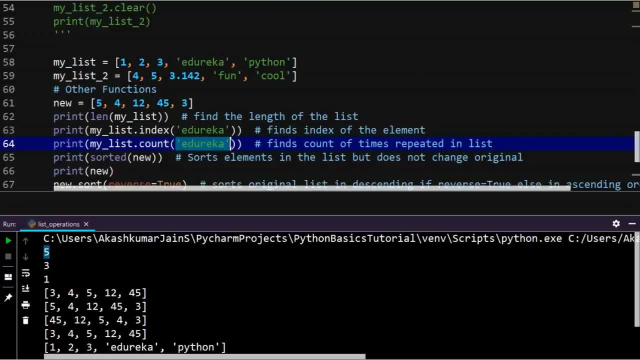 Then we have the count, which basically tells that I want the count of a Durie come, which is being repeated in this particular list. So in our example it is repeated just once. So that's the reason we will only get it as one over here. 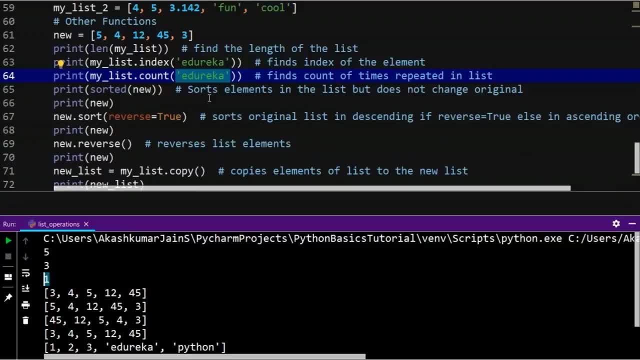 So now we have the sorted and the sort function. the sorted has a return type, whereas the sort function does not have a return type. So if you want to use either the sort or the sorted function, you need to make sure that the data that you have is of the same data type. 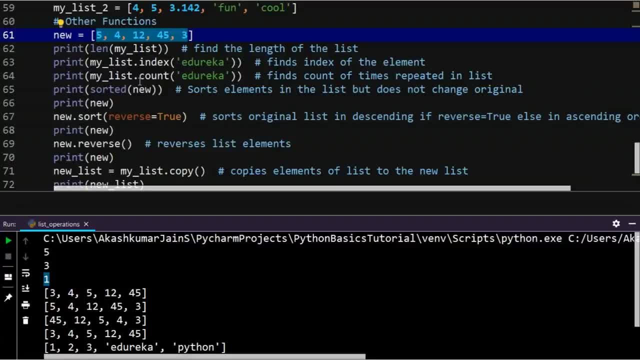 If I try to use the sort and sorted function on these, it would not work. That's the reason I have a new list over here, So I'm just printing the sorted value over here. So that is 3, 4, 5, 12 and 45. 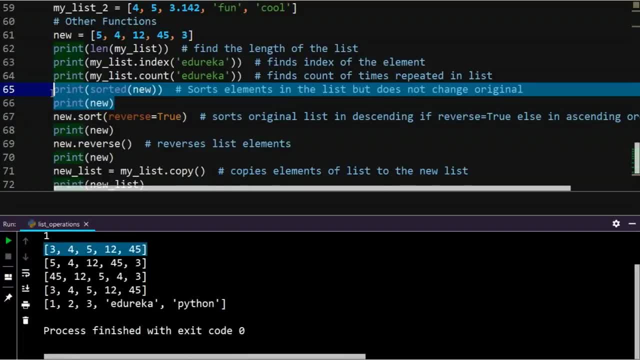 and then I am going to sort 45 and then you can see that it has not affected the actual list. That's the reason I have it over here. So sorted does not change the actual value of the list, It just prints it accordingly. 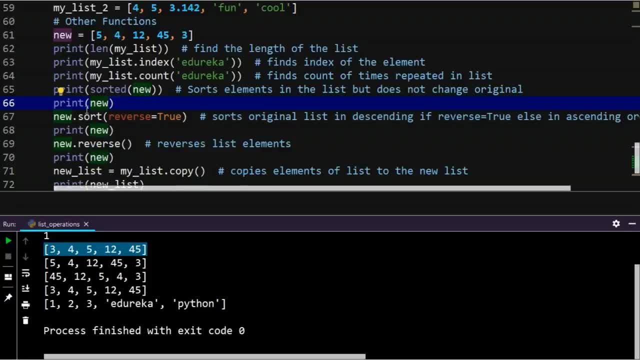 But if I use the sort function it would actually change the value of the list. So if I have a sort and it uses a keyword which is a reverse is equal to true, If the reverse is equal to true, it will sort it in the descending order. 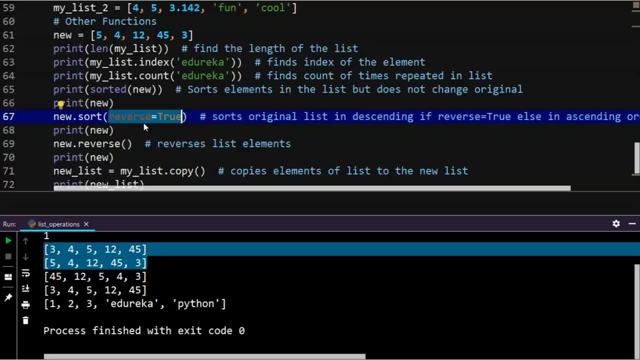 If the reverse is equal to false, it will sort it in the ascending order. So that is what is happening here. So this is in the descending order right now, And then I just reverse it using the dot reverse function. So the data will now be reversed. 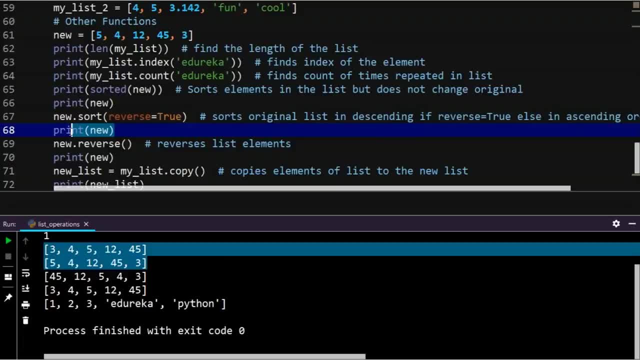 which is basically now in the ascending order. and then I have the dot copy function, which is used to copy a list into another list. So it is my list, dot copy into the new list. So if I have printed the new list you can see. I have the data of my list. 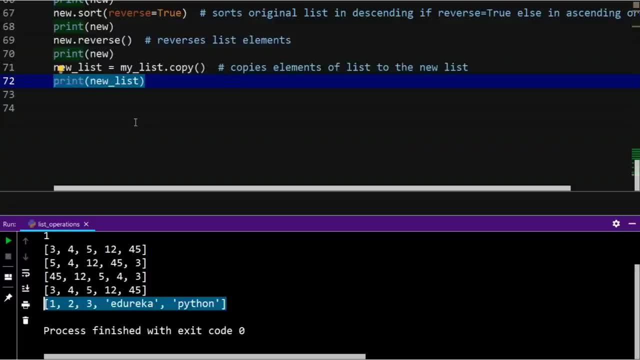 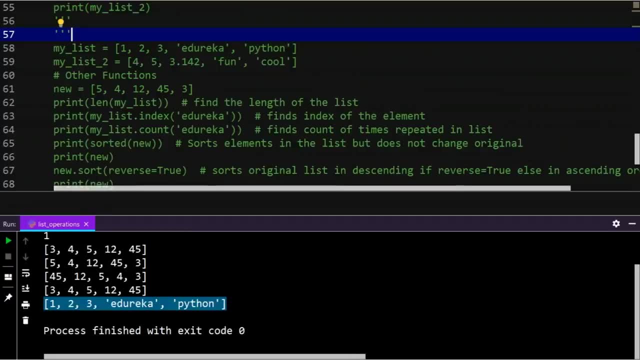 So that basically wraps up list operations. I hope all of you are clear with it. So let's move ahead with the next data type. Let me just close this up. So the next data type that we have are tuples. What are tuples? tuples are basically the same as lists. 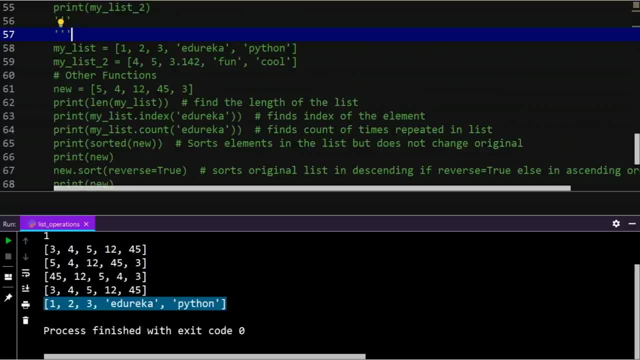 with one exception: that they are not mutable, meaning that you cannot change the data in tuples. This makes tuples much more faster than lists. So how are tuples written? They are written using the parenthesis, So let's move ahead directly to our tutorial. Let me run this. 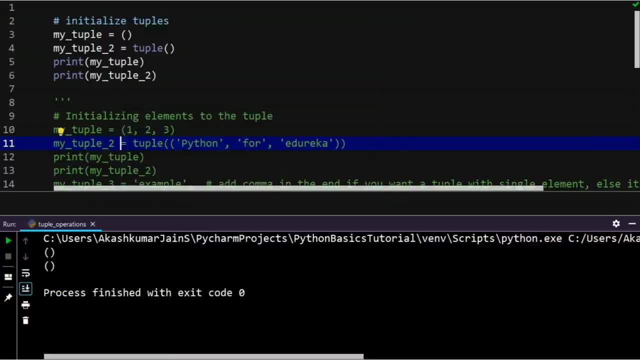 So, as you can see, I have either the parenthesis or the tuple function, and it is the same over here. Also, if you want to initialize the data, you will have to send it as a single variable in the tuple function, Whereas you can use commas in the parenthesis. 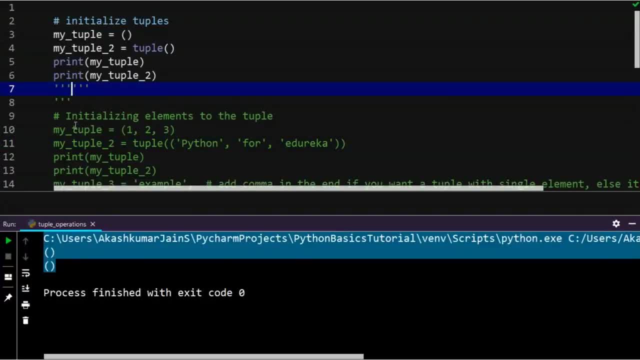 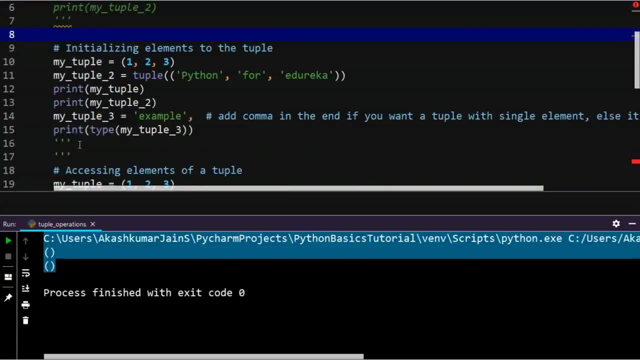 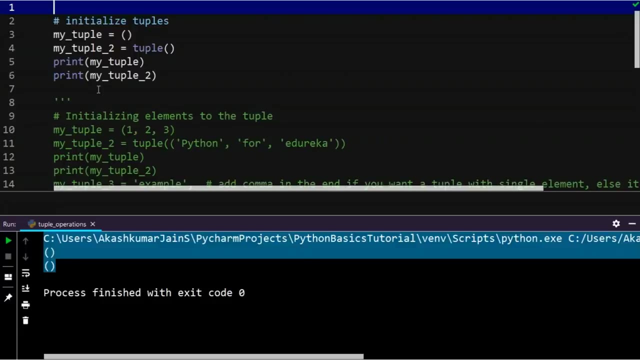 You can see here We have empty lists. Let me go ahead comment this out And let me uncomment all of this. Where would you use empty tuples? It would be cases where you do not know what exactly data has to be sent into the tuple. 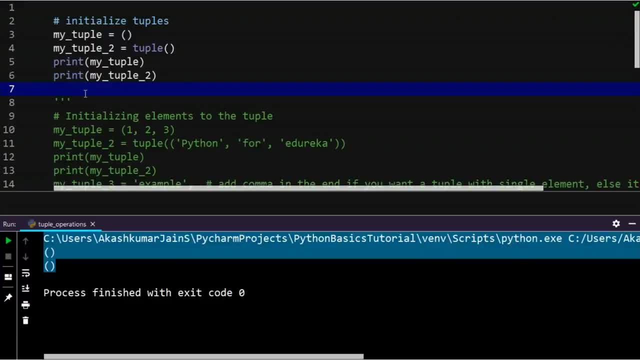 So what do you do over here? You can just concatenate data into it. So, for example, my tuple equal to my tuple plus 1 comma, 2, comma 3. let me print my tuple over here. Let me go ahead and run this. 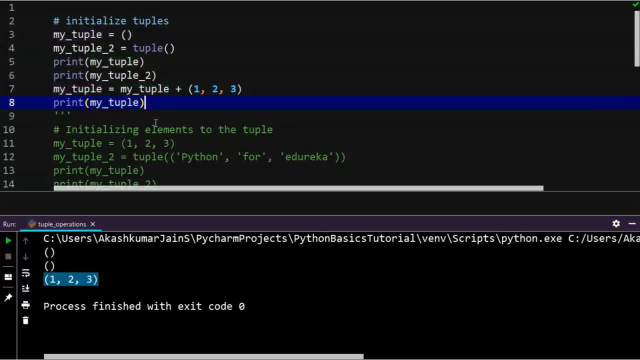 So, as you can see, I have 1, 2, 3 in the tuple. this was because I did not know what do I need to add in my tuple in the previous example, but as soon as I kept doing some sort of operations, I was able to understand what data I need to add. 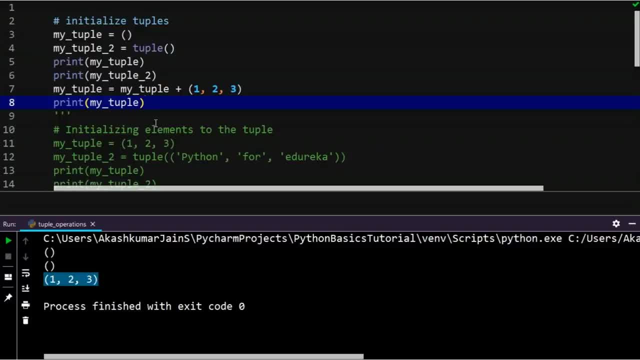 and that's the reason I concatenated it using the tuple. But now, if I try to change my tuples data, as you can see, that statement seems to have no effect, meaning that the tuple will not have any sort of changement or it cannot be mutated. 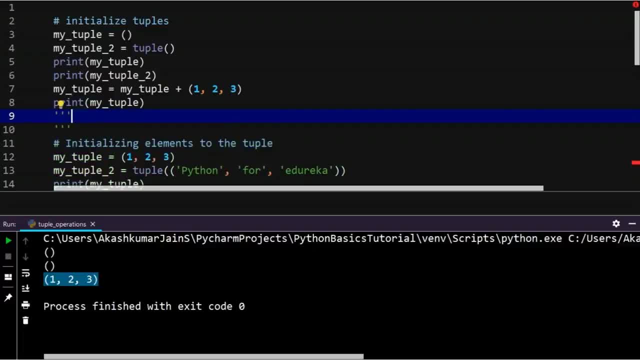 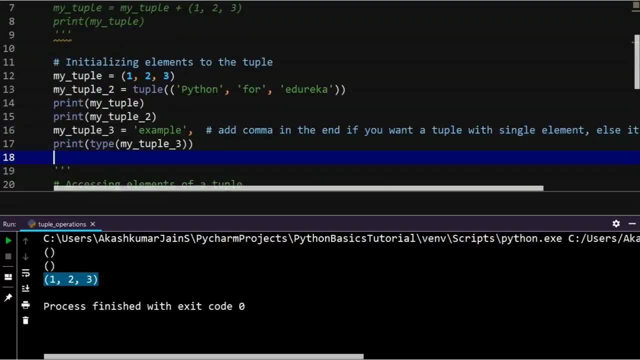 So that's the reason you may want to have some sort of- you know- empty tuple which you may later be populating. So that may be one reason where you want to use Empty tuples, where you do not know what data you need to have. 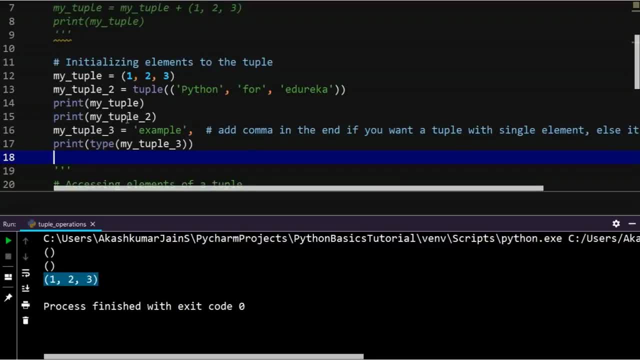 but slowly, slowly, you can populate it accordingly. This is basically how you initialize your elements in the tuple. Let me go ahead and run this So, as you can see, I have a 1, 2, 3 and couple and all of this is sent to it as a single element. 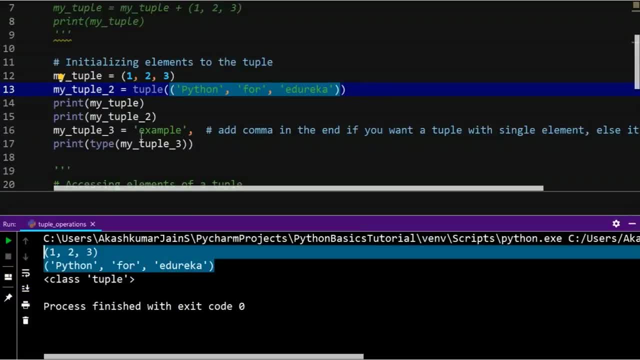 So that is what is happening over here. Now, there is one thing that you always need to remember: when you want to have a tuple with a single element, Make sure that it is always with a comma at the end. Why is this important is because, if I remove the comma, 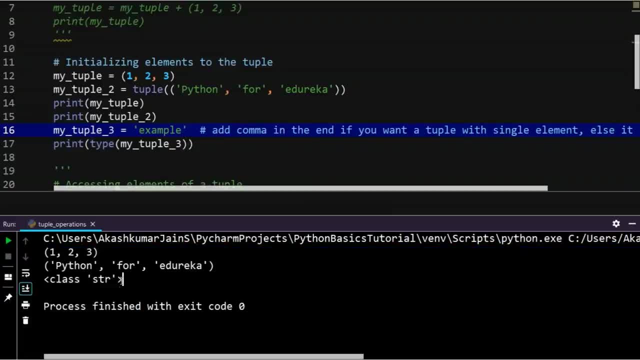 and I show you the type. that is my tuple 3. it is now a string data, So that is the reason a comma is needed, so that you can have a tuple with a single element. So I hope you have understood. How do you initialize the data. 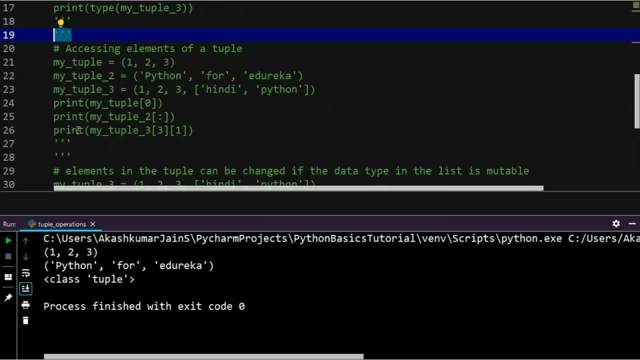 The accessing of elements is the same way as you do it with the lists. Let me go ahead and run this, As you can see: 1, 2, 3, Python and accordingly. So the 0th element of my tuple is 1, over here. 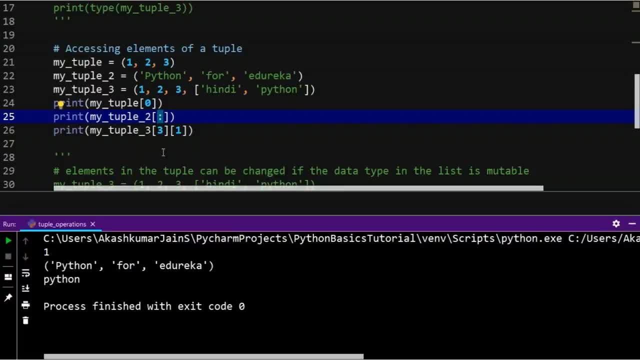 and I want to print everything. So python for Eureka is printed, and then I have the third element, which is a list over here, and I want to print the element which is at index Number one, that is, python. This is how I access the elements. 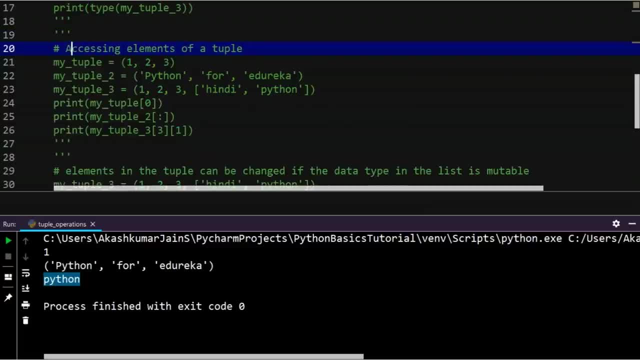 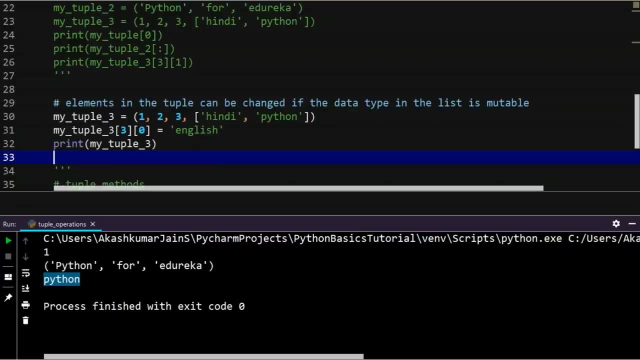 You can actually change the data in a tuple if the data you are trying to change is mutable. So here I have 1, 2, 3, Hindi and python. Now you know that this is a list and a list is basically mutable, right. 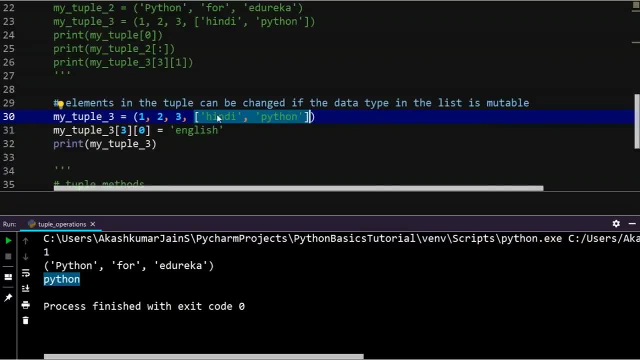 So I can change the data in this particular list, but I cannot change the whole list. Why it's? because it is a part of the tuple. So I'm just saying: go to the list index and then change the 0th element, that is Hindi, change it to English. 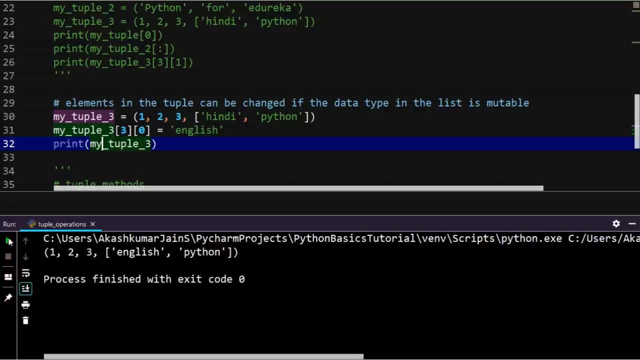 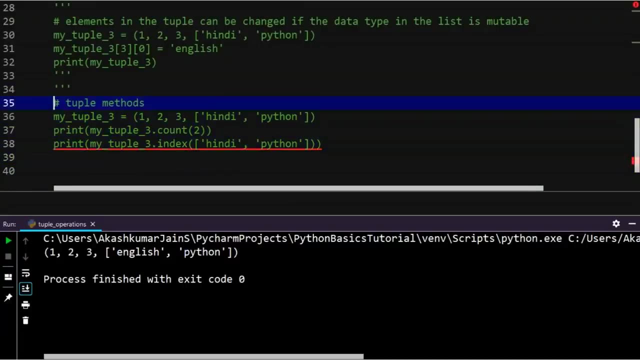 So if I print this, I have a 1, 2, 3, English and python over here, So that is one way you can actually change the data of a tuple. and we have just a few more methods, which are the count method and the index method. 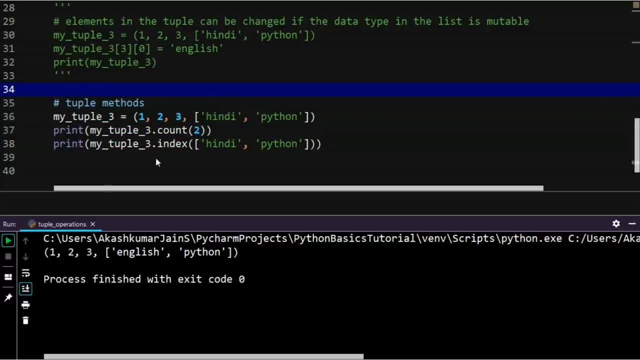 which is the same as how it works in lists. So the count of two is actually just one and the index of Hindi and python is 3.. So I have 1 and 3 as the output. so that basically wraps up tuples. Let's move ahead to the next data type, which are dictionaries. 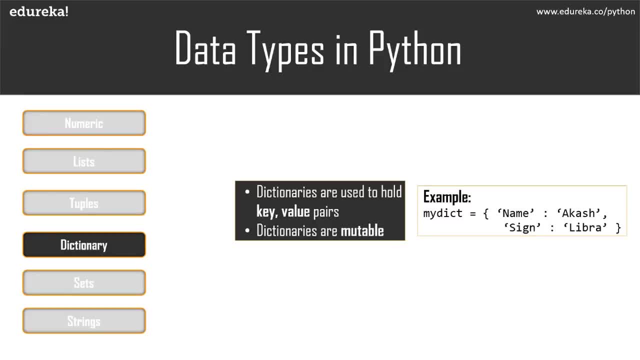 So dictionaries are used to hold key value pairs and they are mutable. now you may be confused. What are key value pairs? So let me help you understand all of this with a real-world example. Okay, think of your contacts application on the cell phone. 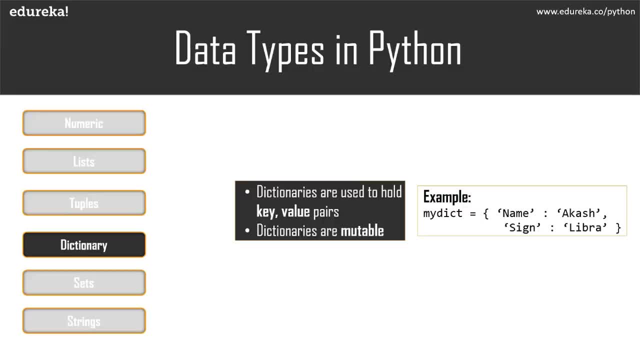 If you see it and go ahead to add a contact, you will always see a few fields that are common all the time. You have name, you have phone number and all the other data that you want to add accordingly. Let us just understand how this works. 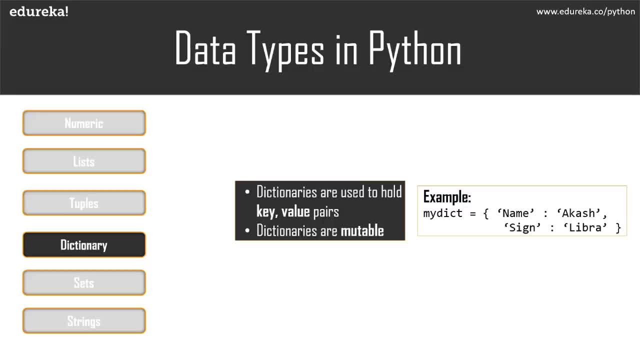 The data we have is name, which is the key- It is always common for everybody. and we have phone number, which is again the key, which is common for everybody. but the value that you enter in those particular fields It will be different accordingly, because you have a name. 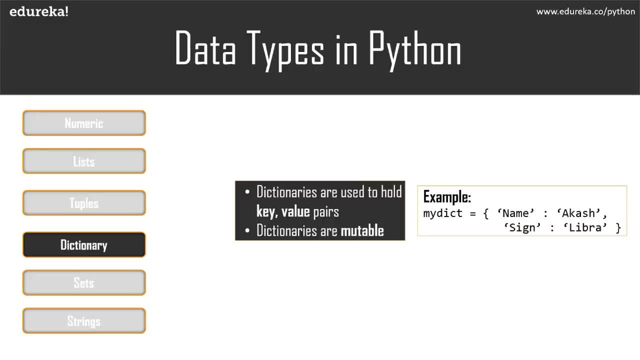 and the value you enter for that name. you have a phone number. You have a different phone number for that particular name. So that's how it works, right. So it is basically key and value. So you have the name, which is the key. 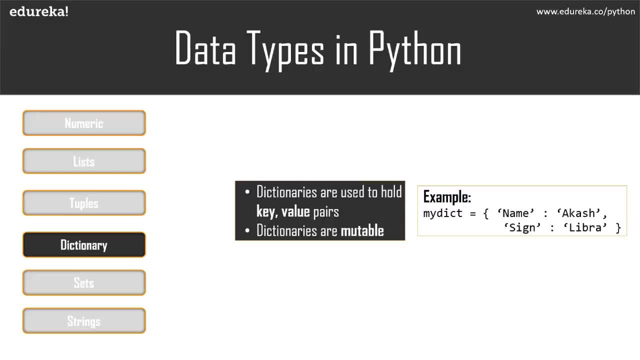 and the value that you enter is the name of the person. So that is basically what is a key value pair. So, for example, over here, I have a name that is my name, That's our cash and I have the horoscope sign of mine. 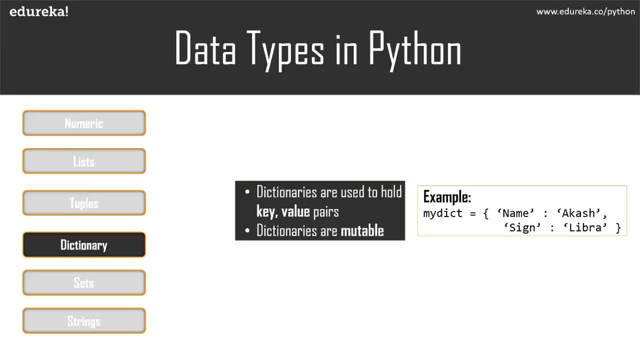 That is the Libra. This is one way how you can have a dictionary. It is to store the horoscope sign of all the people you have. name as Akash and sign as Libra, where name is the key and Akash is the value, sign is the key. 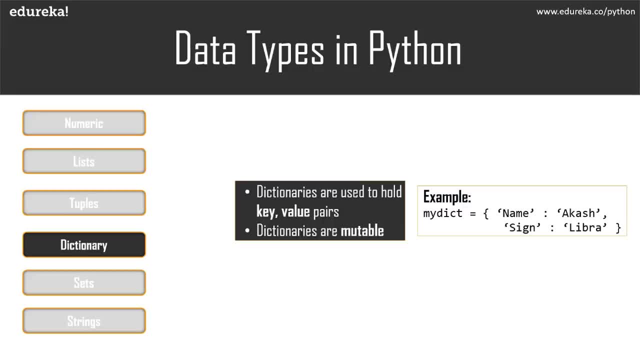 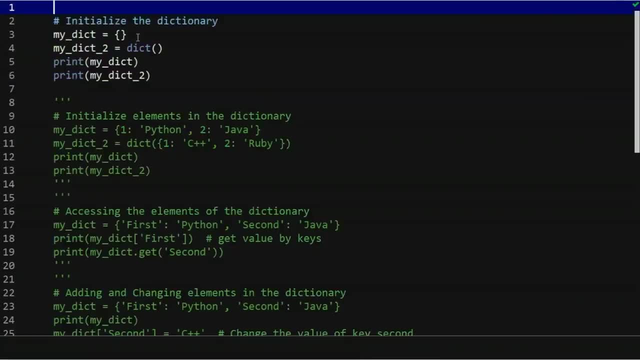 and Libra is the value. So let's move ahead and go to the tutorial that I have ready for you. How do you initialize an empty dictionary? It is done using the flower braces or it is done using the dict method. Dict. Let me run this. 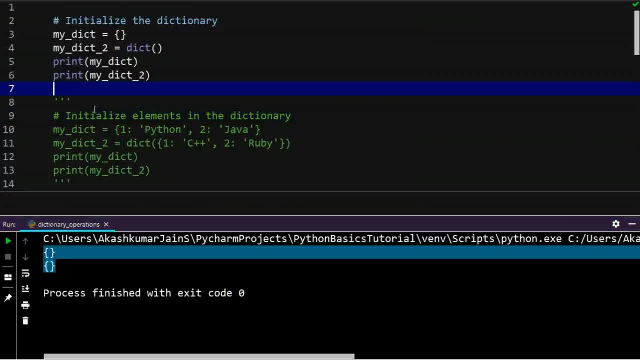 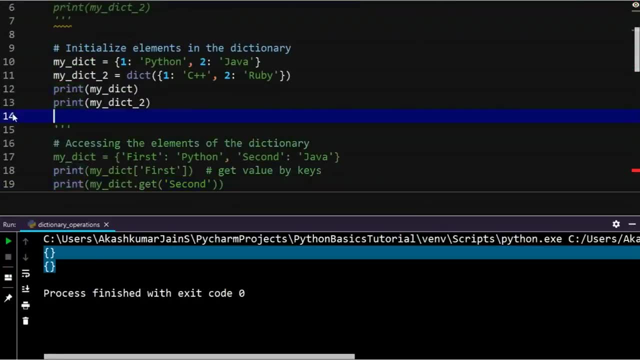 and you will be able to see that there are empty dictionaries over here. Let me go ahead and add back and remove braces to where we need it. So how do you initialize the elements in the dictionary? It is the key and the value. So that is how you actually do it in dictionaries. 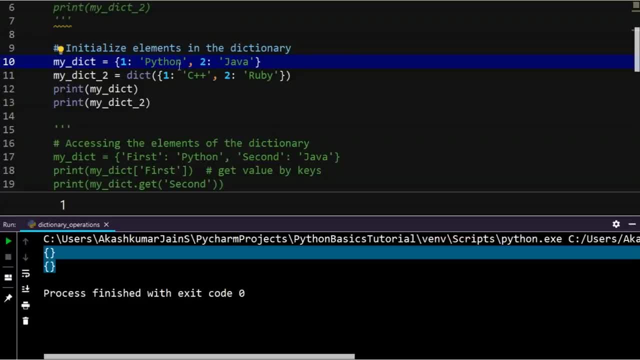 So always a key value pair is taken, because dictionaries are basically key value pairs. So let me go ahead and run this: one is the key, followed by a colon and then the value that that particular key has. So I have one Python to Java, 1 C++ and to Ruby. 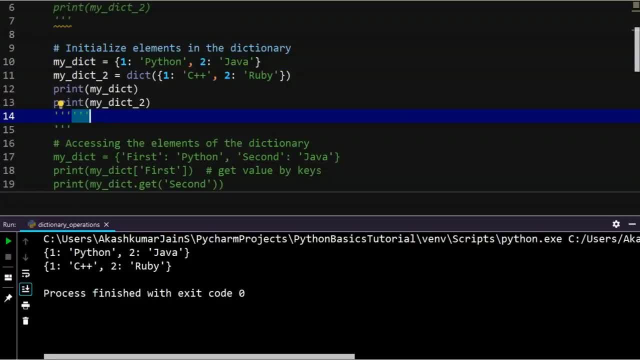 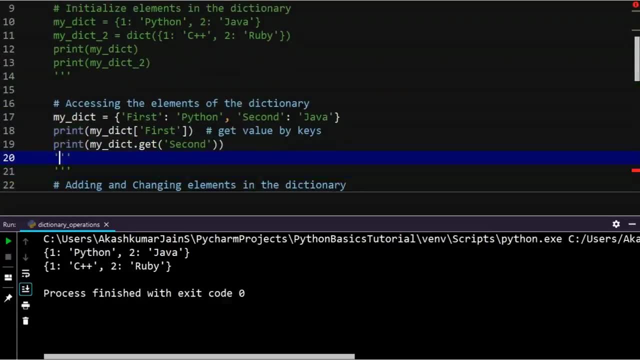 That is how you initialize your dictionary. Let me go ahead and uncomment the next session. So the next is to access the elements. So to access the elements of the dictionary, you do it using the keys. So I have the first as the key and python as the value, second as the key and Java as the value. 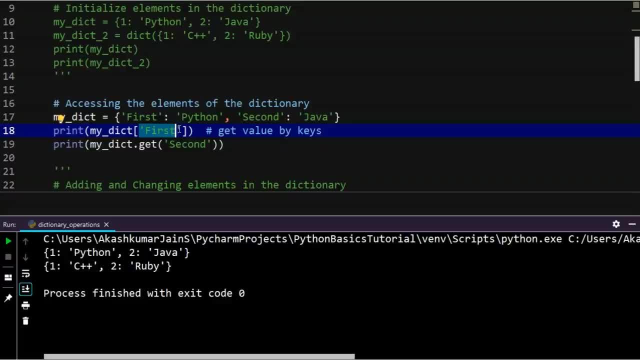 So I have my deck and then the key name, which is first. give me the value from this dictionary where the key value is first, and I can do that even using the dot get method, where I just pass the key value of that particular element. So let me go ahead and run this. 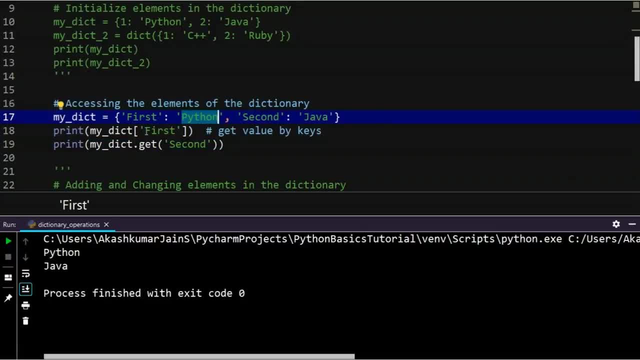 So, as you can see, I have obtained the value python, because I said that I want the value in my dictionary and it has the key. first same thing is done using the get method, where I get the value for whichever I have the key as second. 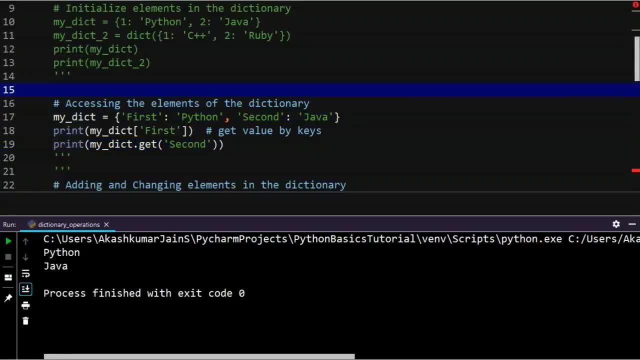 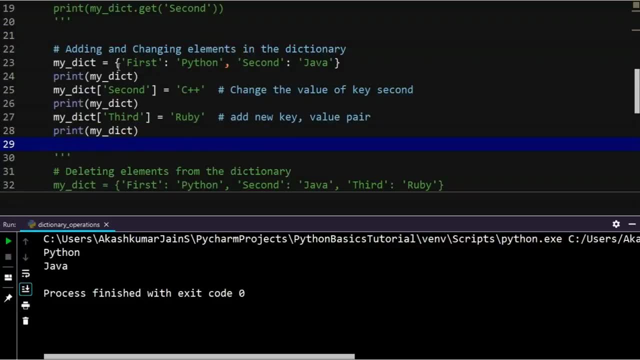 So I hope that makes sense to you guys. Let me show you how you can change and add elements into your dictionary. So this is the dictionary that we have over here, and then I want to change The data that is in a second, saying that I do not want Java. 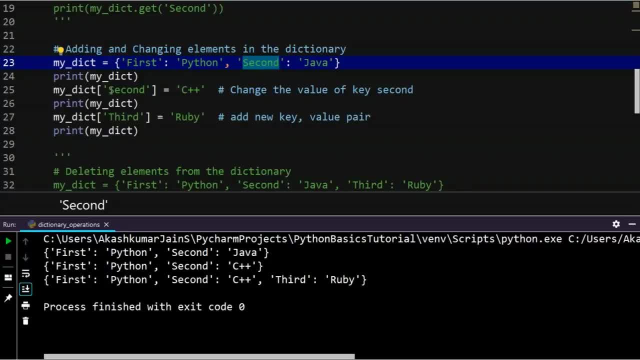 I want this to be C++, So I just say my dict of second and I want to change it with the value, So I just pass the value to it. So now, if you can see here, Java is now being changed with C++, right. 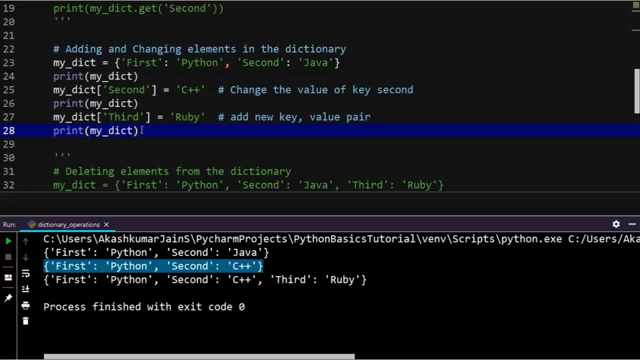 So now, how do you add elements into the dictionary? You do that by giving the key value pair. So you just see that, my dict, and give the key and then you give the value. So that is how I have obtained the output. first, python, second: 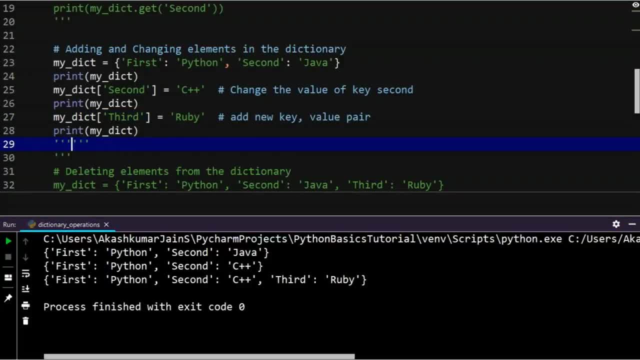 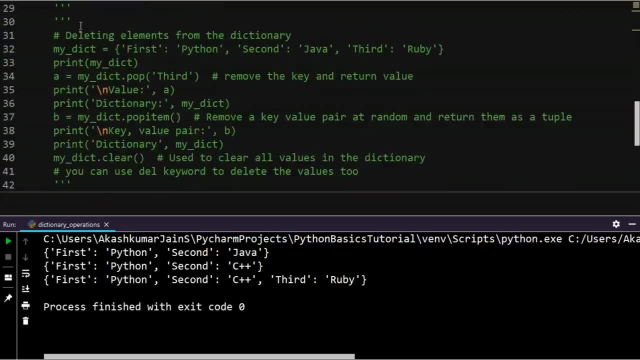 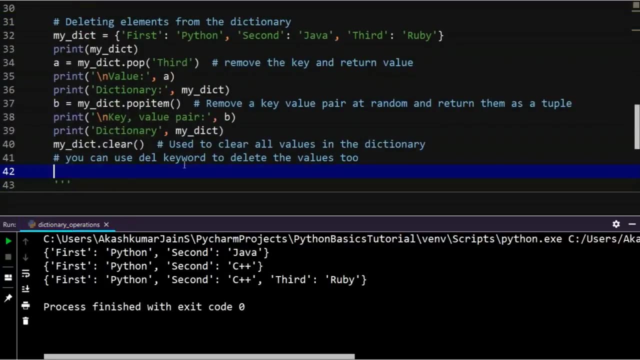 C++ and third as Ruby. So that's how easy it is to add your elements into the dictionary. Let me go ahead and show you how to delete elements Now. one way is to use the del keyword. You can use it accordingly. It works the same way every place here. 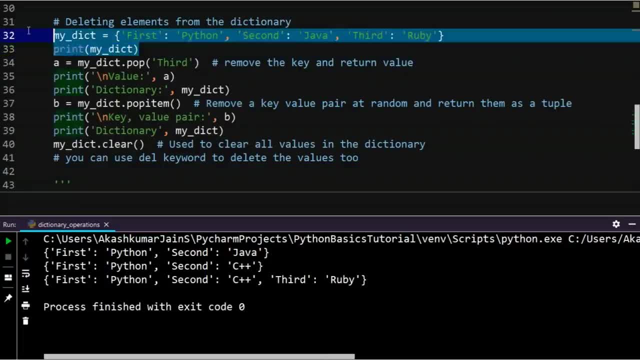 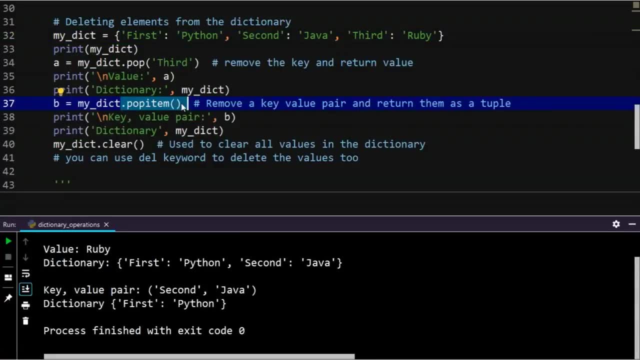 You would just have to give the key name. So I have more than dictionary, which is my dictionary. So the next way Is the pop item function, which will return the key value pair to you in the form of a tuple. and how does this work? the item. 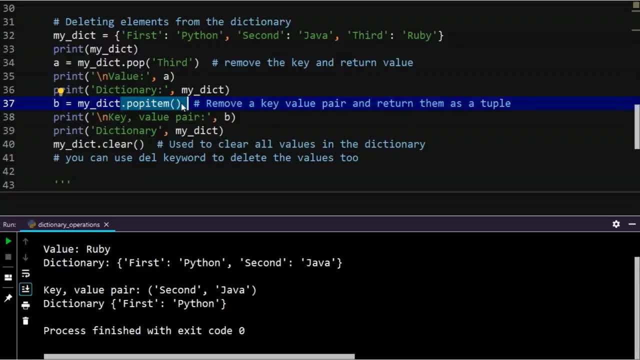 which is in the last position, will be given back to you. So, if you can see over here. second, and Java, which was at the last position, have been popped out as a key value pair in the form of a tuple. So, as you can see here. second, 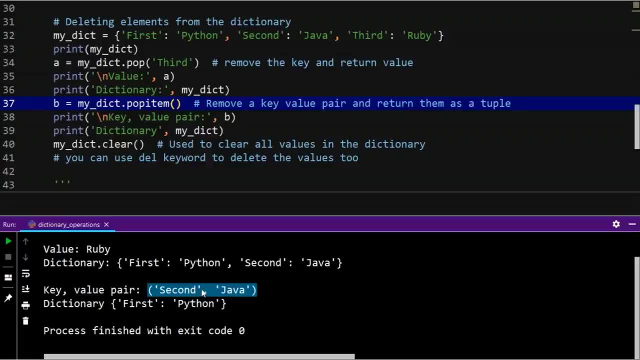 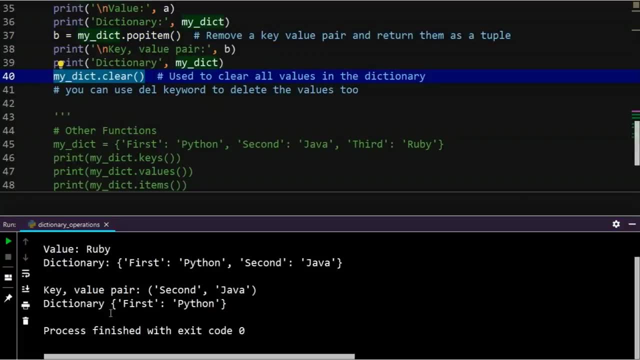 and Java have been returned back and they are in the form of a tuple with a key value over here. So that's how you use the pop item And then you have the clear, which is used to just basically empty the dictionary. I hope you're clear with that. 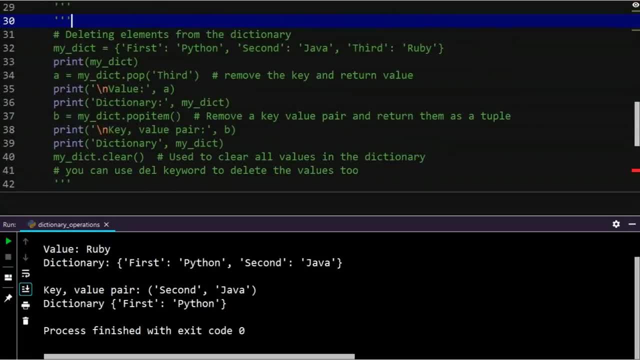 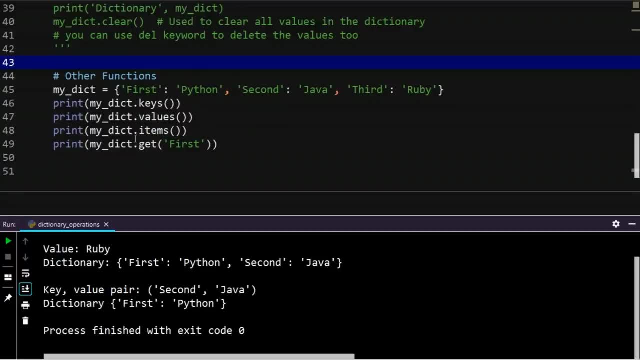 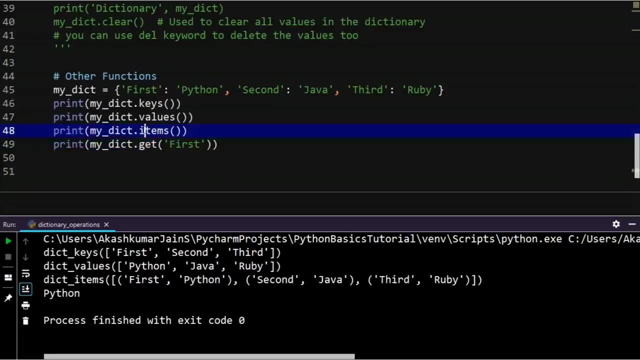 Let me comment all of this out and move over. So we have a few functions that may be helpful to you when you start using dictionaries. So they are the keys, values, items and the get function. You already know what the get function does. We have keys, which basically returns all the keys. 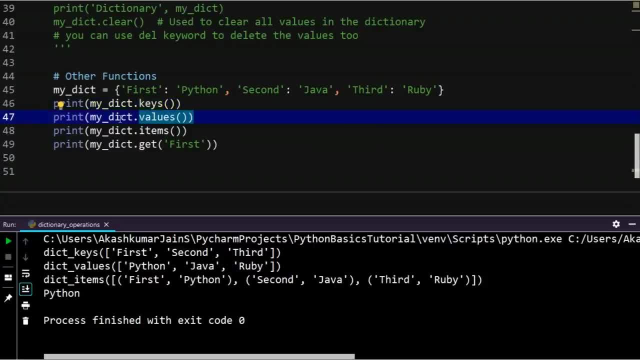 for this particular dictionary. We have the values which returns the values of the dictionary. We have the items which returns the key value pair in the tuple forms. So, as you can see over here, these are the keys for second. third, these are the values Python, Java and Ruby. 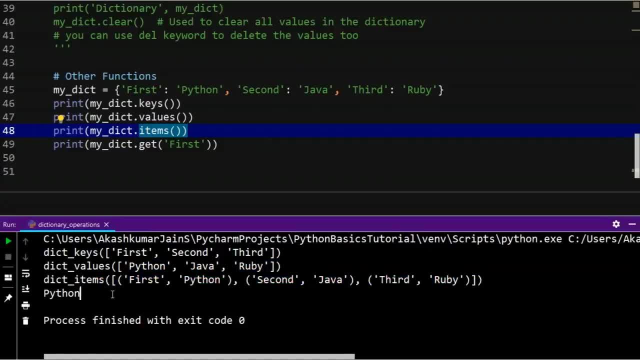 and then you have the dict items, which is the key value pair, and you know how the get function works. You just pass the key and the value will be returned back to you. So that basically wraps up dictionaries. Let's move over to sets, the next data type. 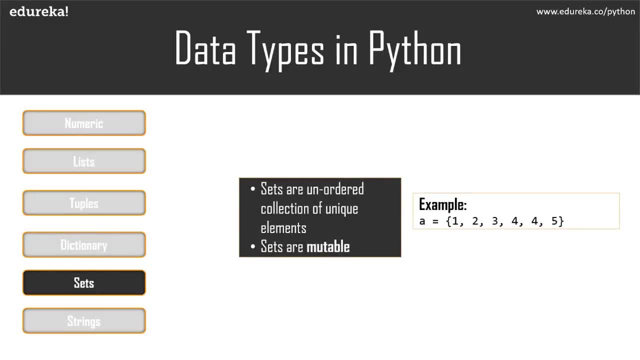 Sets. if you know arithmetic, you would know what sets are. that is basically what we have in Python right now. sets are basically unordered collection of unique elements and they are mutable. So how do you write sets? So sets are basically written in the flower braces. 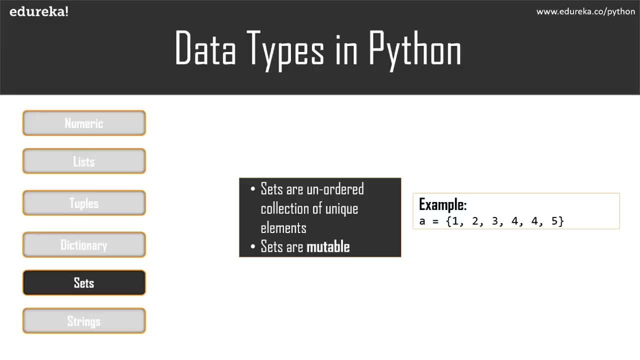 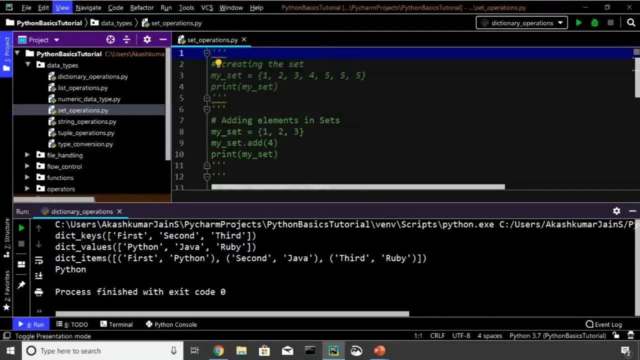 but with a comma only, you do not have a key value pair. Whenever you have a key value pair, It becomes a dictionary. whenever you just have elements, it becomes a set. So let's move ahead and go to the tutorial. So let me move back to the presentation mode. 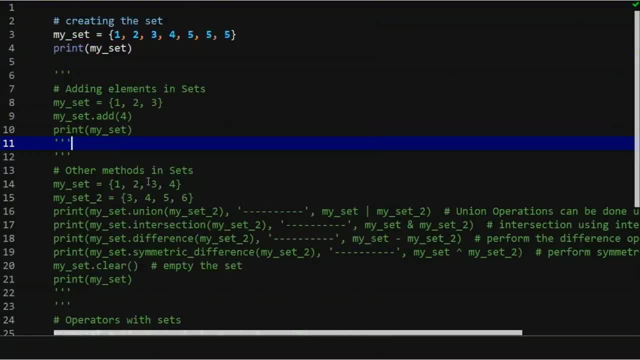 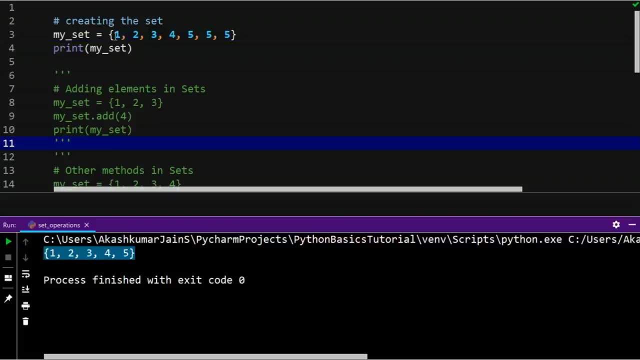 How do you initialize your set? You do it using this way and if you can see the output, it is just 1, 2, 3, 4, 5.. But whereas I have written 1, 2, 3, 4, 5, 5, 5.. 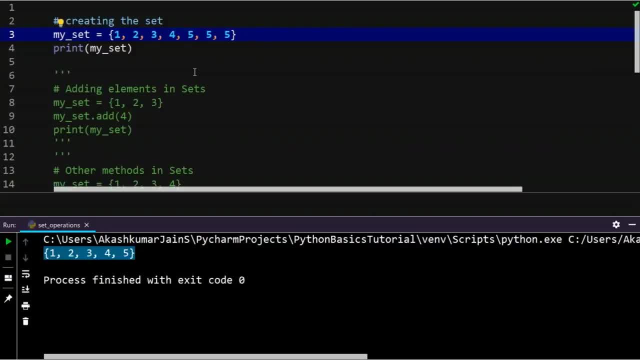 Why is 5, 5, 5 not repeated? Remember the definition: always, set is a collection of unique elements, right? So even if 5 is repeated, even a thousand times, it will still be taken it as one time. So that is what is basically a set: how you initialize your set. 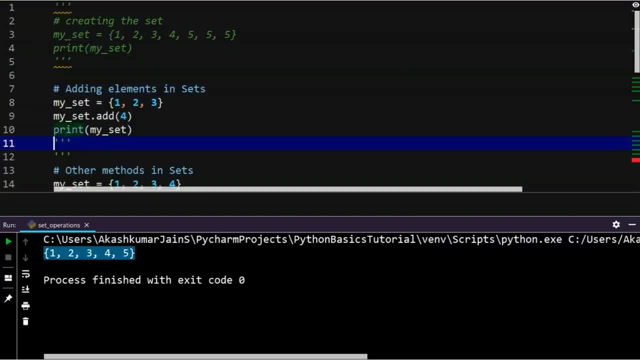 Let us move over to how you add elements into your sets. So adding the elements are done using the add method. You can see I have a list 1, 2, 3 and I just want to add 4 over here. So that's the reason I obtained the output 1, 2, 3 and 4.. 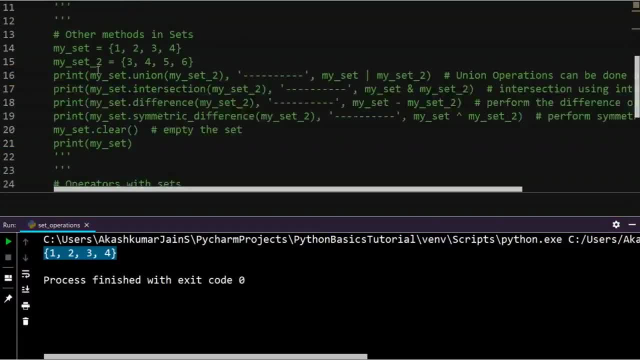 So that's how easy it is to add elements into your sets. So let's move over to the other methods that we have Now. if you remember your arithmetic, you would definitely remember what was Union- intersection difference and symmetric difference, right? So what are basically all these methods? Union is basically. 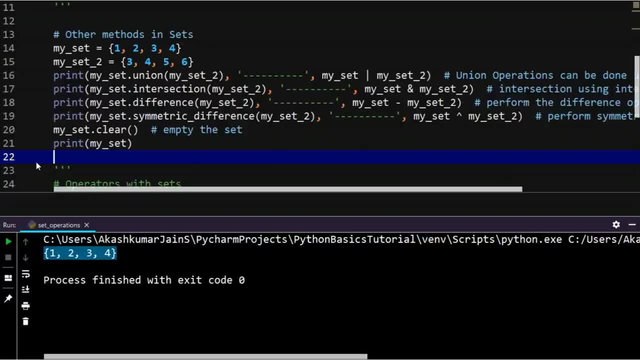 adding the elements of both the sets. intersection is to find out the common elements. difference is to delete the common elements and have the remaining elements given as the output, and symmetric difference is to take out both the common elements that are in the set. symmetric difference is to take. 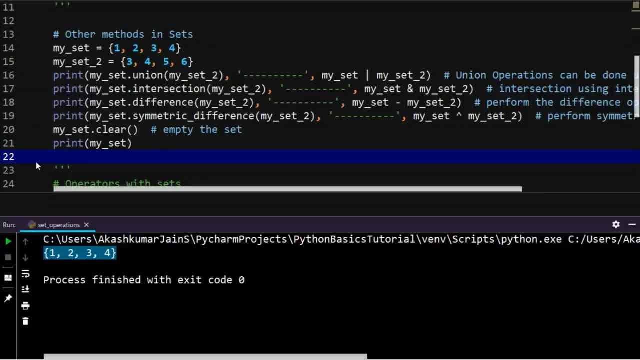 out All the elements that are common in the set and give as output the remaining elements that are in both the sets. that is basically what was Union: intersection difference and symmetric difference. So let me just go ahead and run this program for you. So if you know Union, it is going to add both elements. 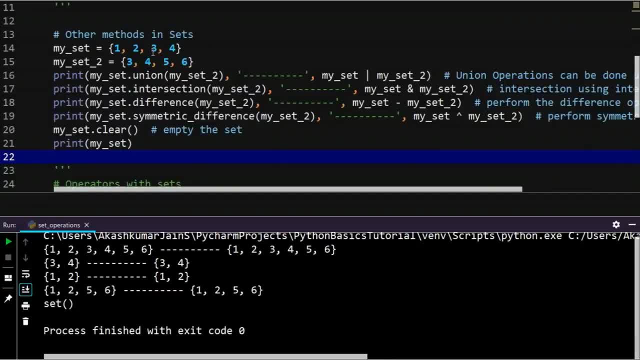 So it would be 1, 2, 3, 4, 3, 4, 5, 6, but it is unique, right, So I would just have 3, 4 repeated once. So it would be 1, 2, 3, 4, 5, 6. the same can be done using the pipeline. 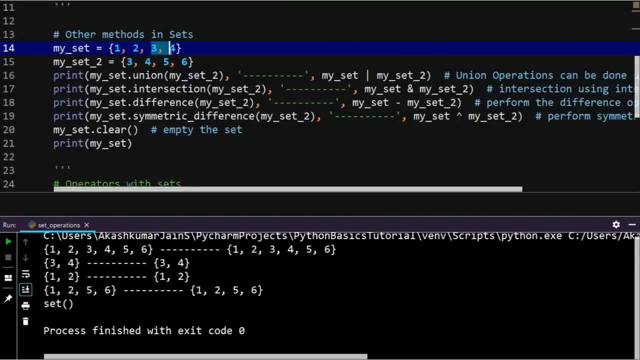 operator. The next is intersection. So 3 and 4 are common. So that's why 3 and 4 will be given as the output, and it can be also done using the and operator. then you have the difference, which is to take out the common elements. 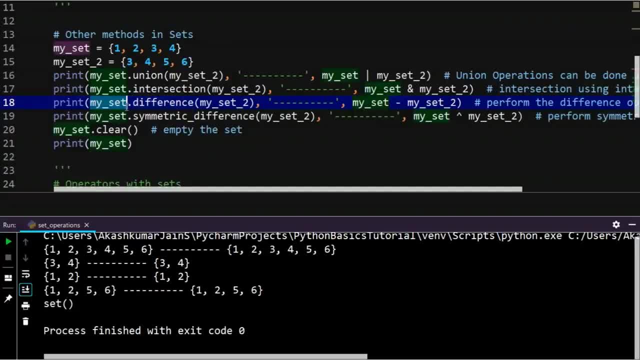 and then show the elements that are present in my set, which is the first set that you give over here. So 3, 4 are common and the remaining elements in set 1 are 1 and 2. so 1 and 2 has given us the output. next you have: 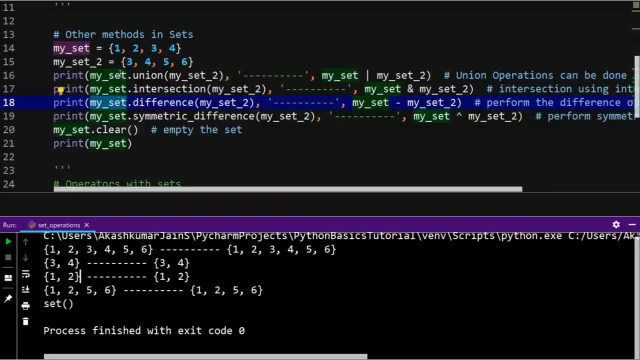 the symmetric difference, which is basically the same as the difference function, but it would take the elements that are remaining in both the set. So 1, 2, 5 and 6 will be given as the output. So I hope you're clear with that, and then we have the clear. 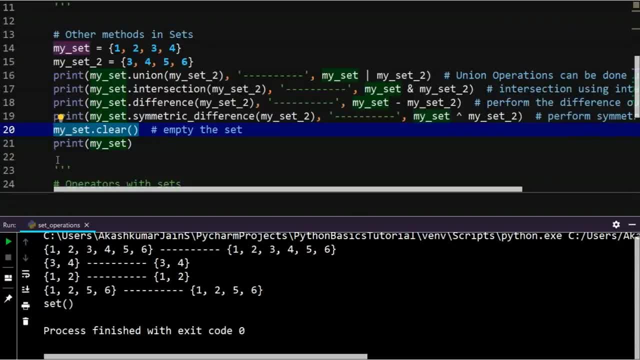 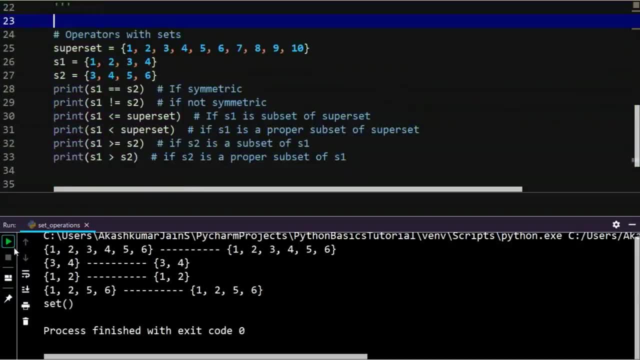 function which is used to basically give you back the empty set. Let's move ahead to the operators that we have in sets. Let me go ahead and run this. So we have three sets over here: superset, set 1 and set 2, the. 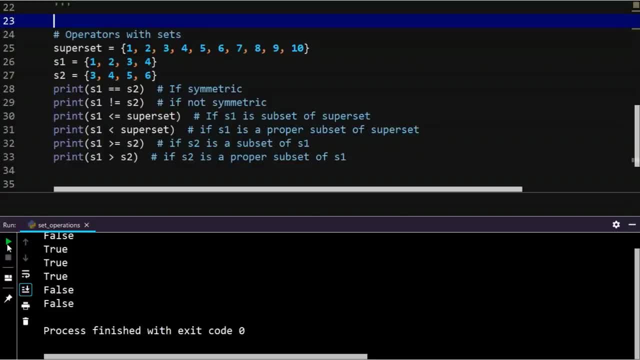 double equal to is just to compare. if both the sets are equal, It would be true, but we have got false meaning that both the sets are not true. The second one is to check if both the sets are not equal. We know that both the sets are not equal. 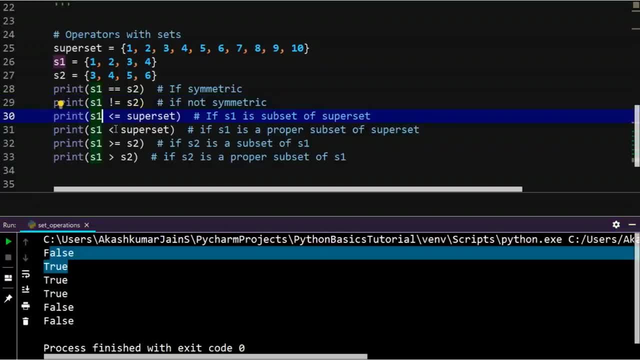 That's the reason we obtain a true. next, We have the subset and the proper subset. Now what is a subset? subset is basically to show that all the elements of one set are present in the other set. So set ones elements are definitely present in the. 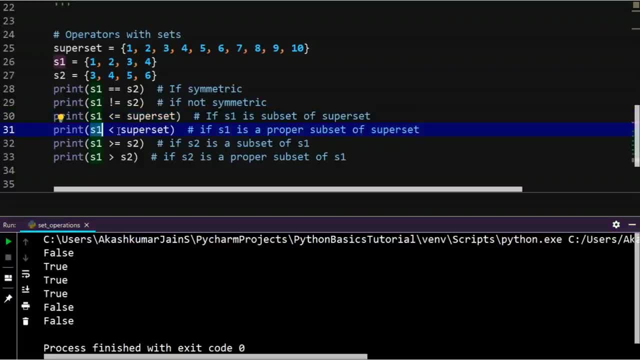 superset. That is the reason this is a true and we also have the set and we also know what is a proper subset. So that is the reason we also obtain a true over here. and then we have s1 and s2.. We are just checking if s2 is a subset of s1. 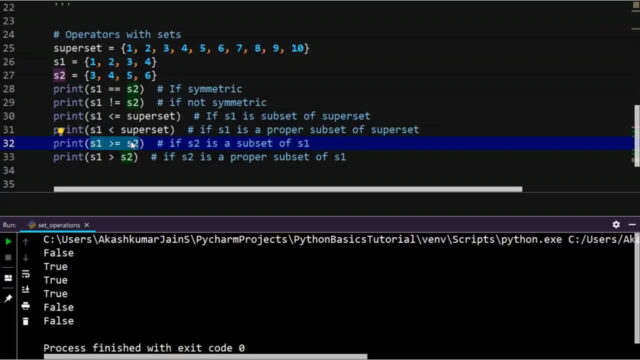 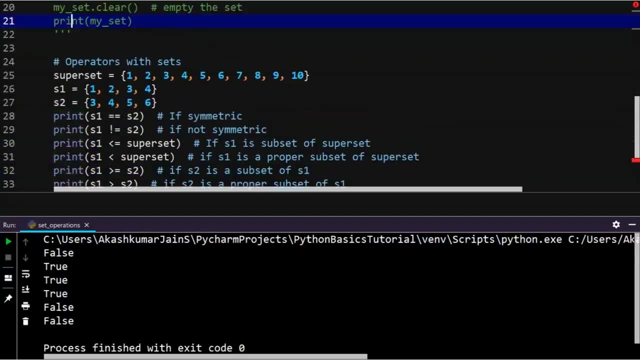 Obviously it is not, and that's the reason. even if it is not a subset, It would definitely not be a proper subset. So that brings us to the end of sets. Hope you're clear with all of this. Let's move ahead to the next data type that we have in Python. 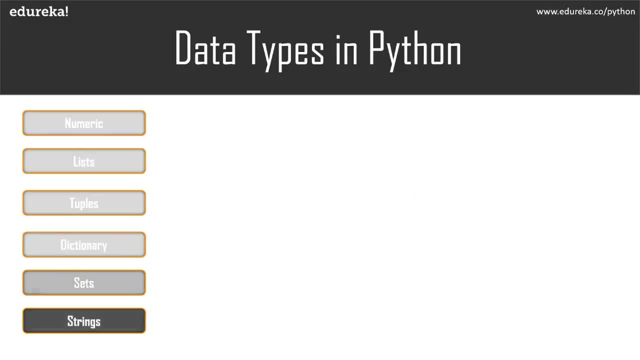 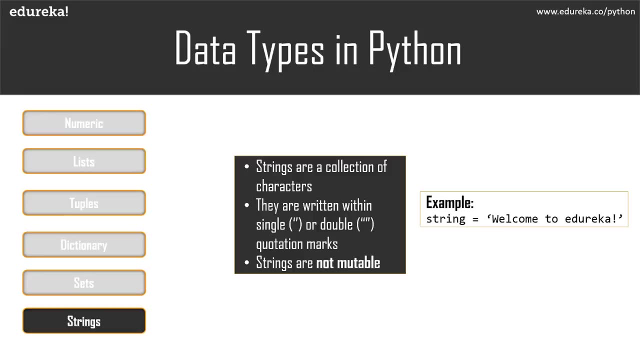 So I hope all of you are clear with sets. Let us move ahead and go to the last data type, which are strings. So what are strings? strings are basically a collection of characters. if you have a BC capital, a capital B capital, C, all these are characters right now. 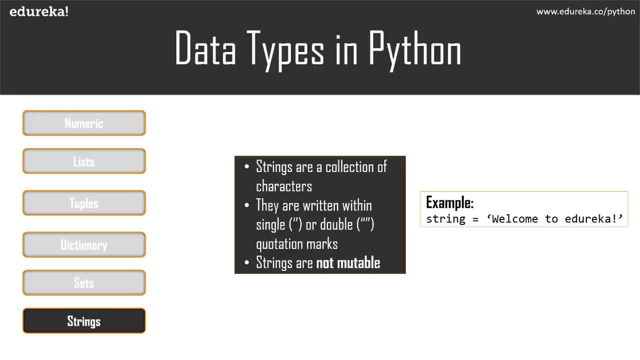 we have to remember that python is case sensitive, which means that capital A and small a are different from each other. So strings are basically written using either the single or the double quotation marks, and they are not mutable, meaning that you cannot change Particular data in the string. 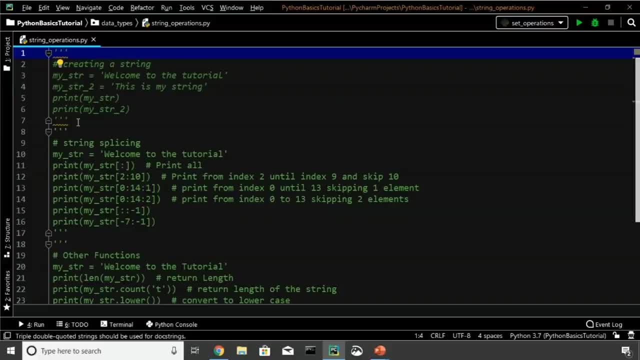 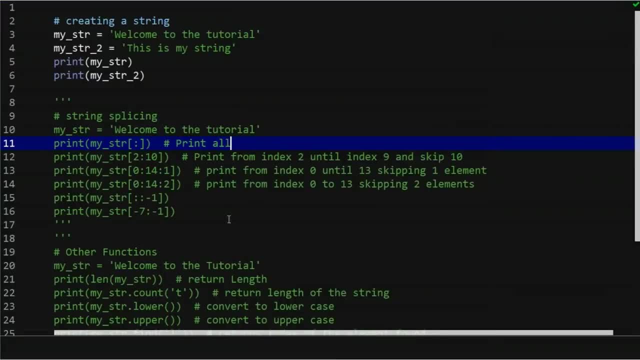 So let's move ahead and go to the tutorial that I have for you guys. Let me just uncomment what is needed. So, as you can see, I have two strings over here. That is, my SDR, and my SDR to, which is welcome to the tutorial. 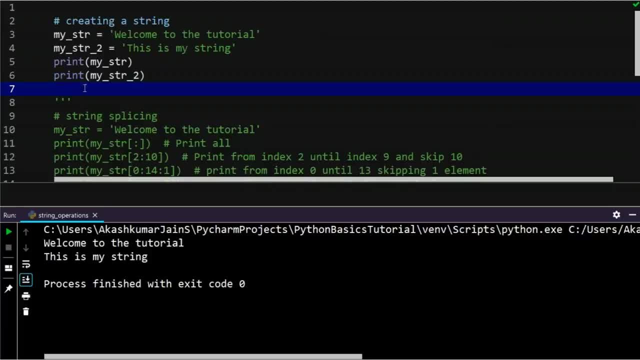 This is my string, So, as you can see, that's the output that we have, and next is string splicing. Now, string splicing may be very much easier for you guys, because you've now Understood how we access particular data in lists- tuples. 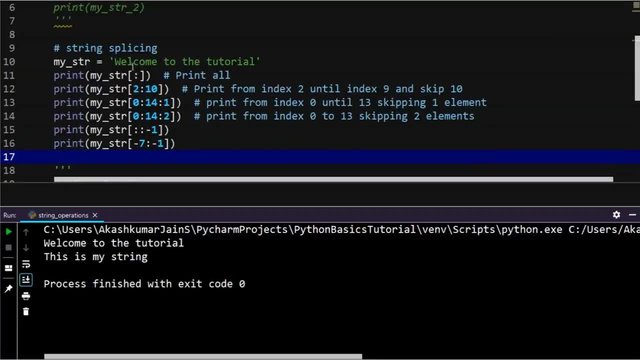 and all of those data types. It's the same with your strings. Also, if you do not have any start or stop index, it will print the entire string. This is from 2 to 9 and is skipping 10.. This is from 0 to 14 and skipping one element. 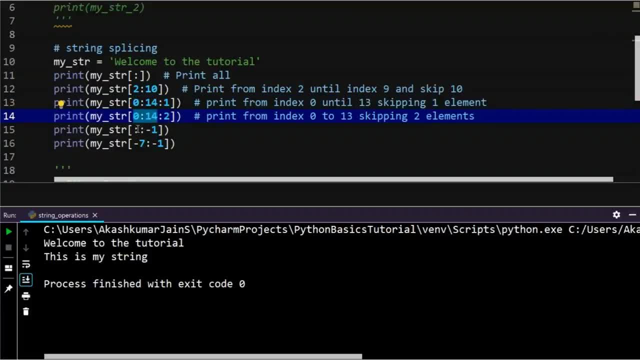 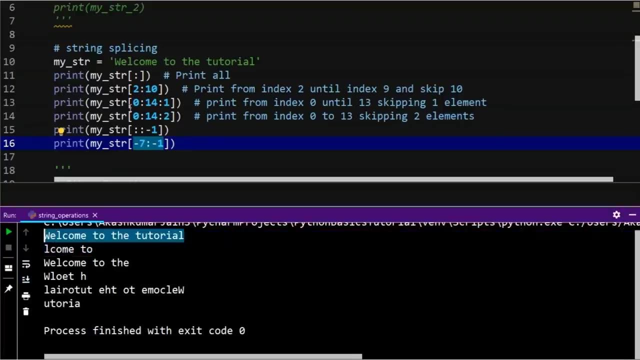 This is from 0 to 14, skipping two elements. This one is to reverse the string and this is from the reverse order. So let me go ahead and run the program And we have our string as welcome to the tutorial. and, as you can see, we have welcome to the tutorial. 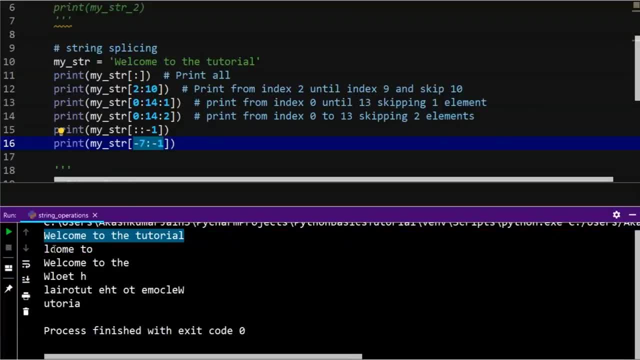 that is for the first one, and next is from 2 to 9, which is L come to, and then we have 0 to 14.. So that is welcome to the, and if I'm skipping two elements, it will be this particular string over here. 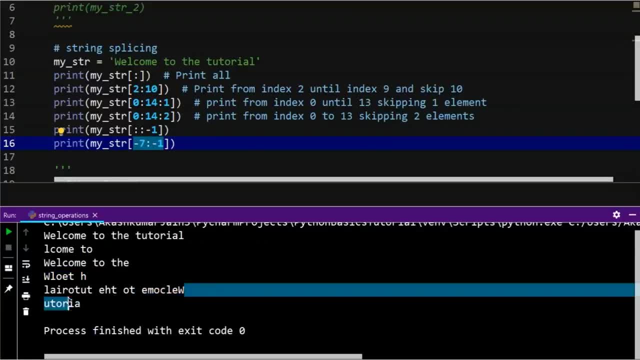 Next, it is to reverse the string. So, as you can see, this is in the reverse order and then we have to print a particular range in reverse order. So this is the output that we have obtained. So I hope you're clear with how you access. 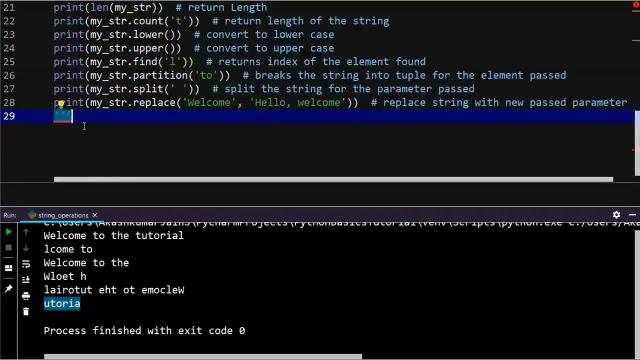 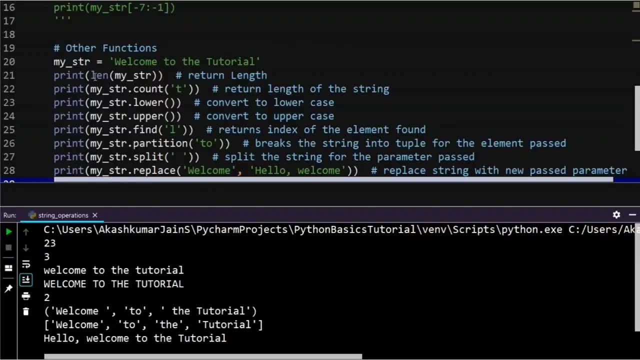 or how you splice a particular string. There are many and many functions that we have for strings. I've just defined a few of those over here. So the length, obviously, which is to give the length of the string, which is, that is 23, then see how many times. 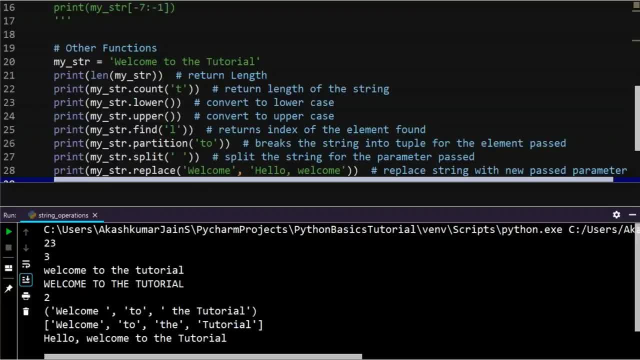 the element T has been repeated, So it is a three times. then this dot lower is to convert The string into a lower case, and dot upper is used to convert it into an uppercase. So, as you can see, this is the output that we have then. 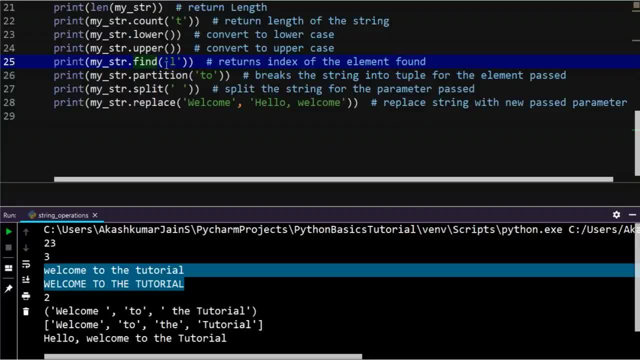 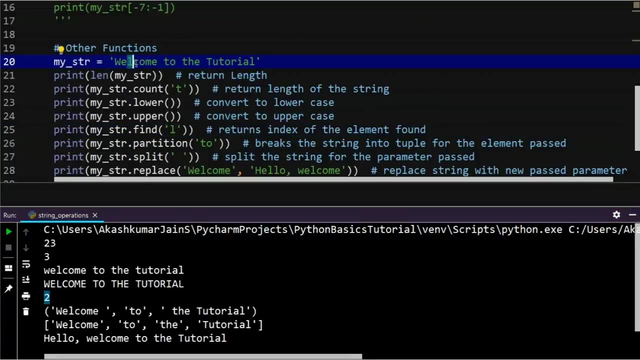 the find function will basically return the index whenever this particular element has been obtained, and if it is not obtained, it just gives out an error. So you can see here: L is obtained at the first time at index number two. That is the reason this index will only be returned to us. 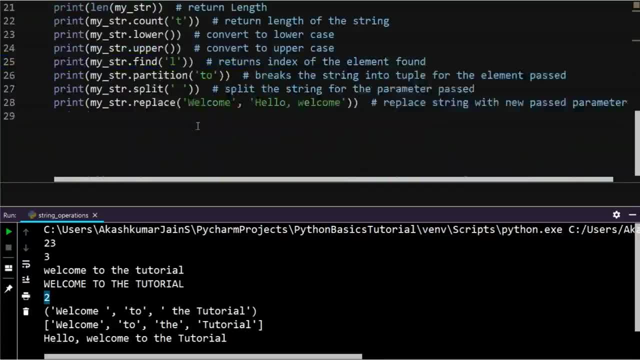 and this particular index for this element will not be returned. The find function will return the index where it has accorded at the first time. next is the partition function, which is basically used to partition the string based on the input that you have given over here. 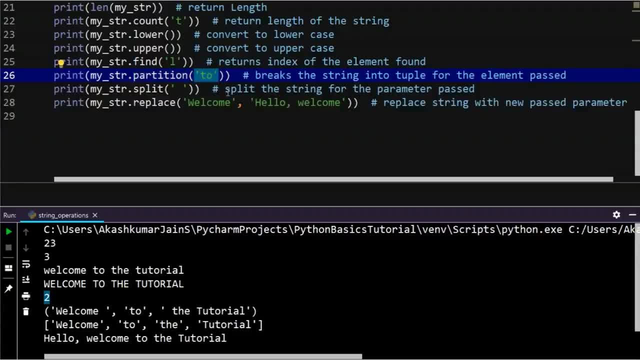 So I am seeing that partition, the mySTR at 2- so welcome- will become a one particular variable. Then we have to, which will be the other variable, and we have the tutorial, which is the third variable, and all of this is now into a tuple, the same thing. 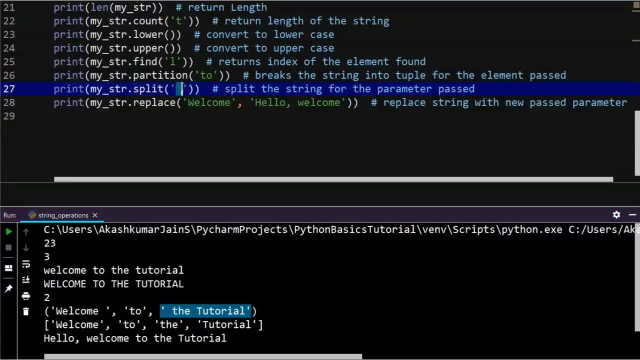 goes to split function, where the data will be split based on the input that you have given over here. So if I do, it split and I have given a space over here, so welcome to the tutorial. and all of this will be converted into a list. 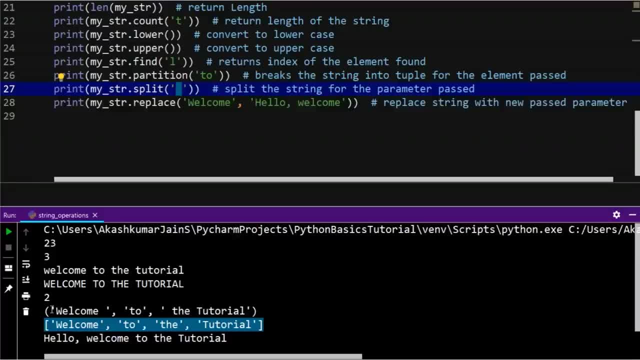 So you have to remember that the partition function converts it into a tuple and the split function converts it into a list and we have the replace function. So it replaces whatever was given in the previous string, and with the new string that it has to be replaced with, I want to change. welcome. 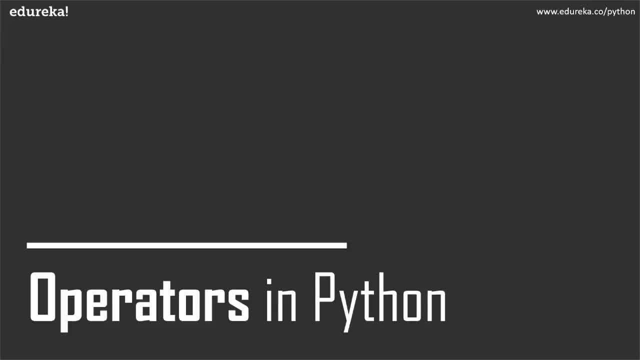 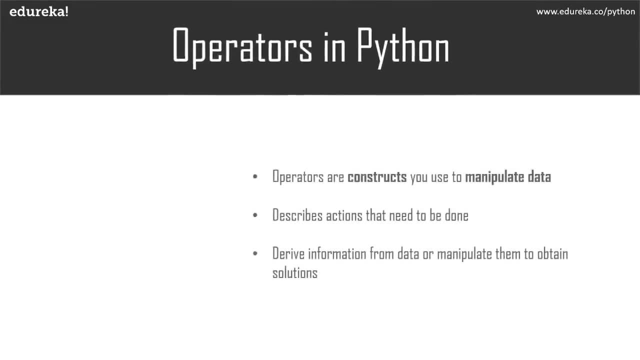 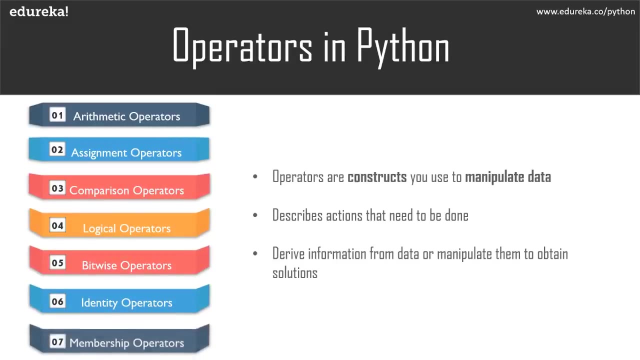 with hello welcome. So hello Welcome to the tutorial. Let's move ahead and understand what are the different operators that we have in Python. What is an operator? an operator is basically a construct that you use to manipulate data. Let's understand this by a real-world example. 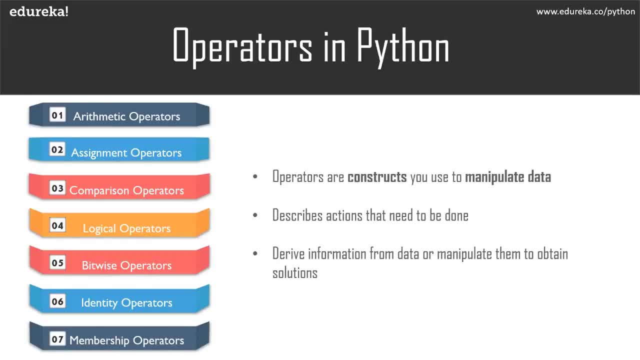 So suppose there are two friends and they want to find out the exact amount of money that both of them have. So what do you do? You take the money from the first friend, You take the money from the second friend and add all of that, right. 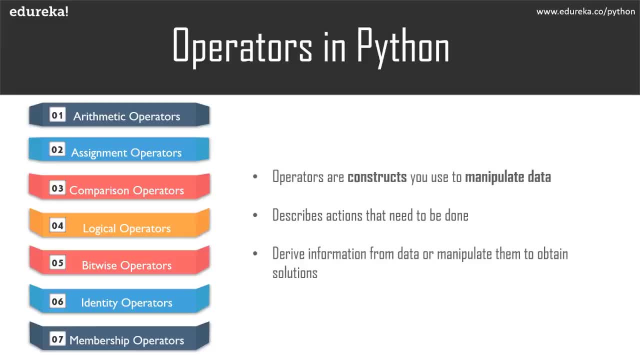 For example, let's say the first friend has 50 and the second friend has 50. So in your mind you just see that, Okay, so 50 rupees plus 50 rupees becomes 100 rupees. So that way of manipulating the data in your brain. 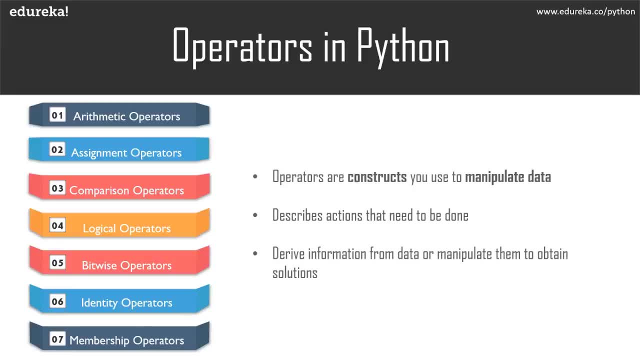 That is what you have done here, and the operator that you use was the addition operator. So that is basically what our operators- they are basically constructs that are used to manipulate the data, So they can be used to derive information or to manipulate to obtain a solution. 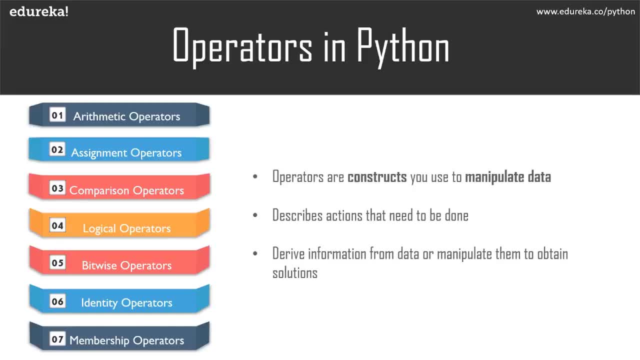 So, as you can see, we have seven operators over here. They are the arithmetic, assignment, comparison, logical, bitwise, identity and membership operators. So let's go ahead and see all of these operators. So the first one is the arithmetic operator. It's as the name suggests. 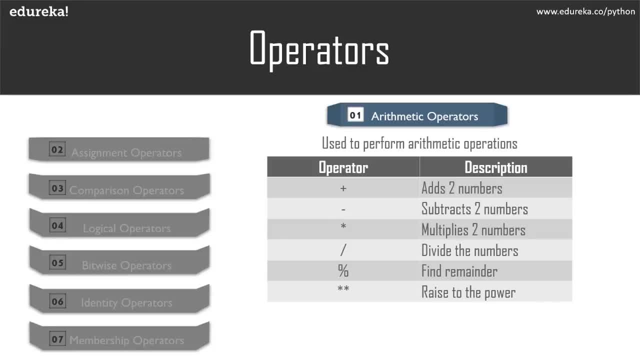 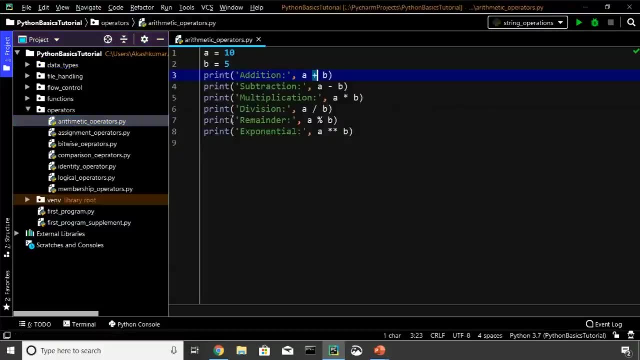 They are used to perform the arithmetic operations. So we have the addition, subtraction, multiplication, division, remainder and exponential operators. Let's go ahead and see an example of these, those data types, and move over to operators. So we have the arithmetic operator. Let me go to the presentation mode. 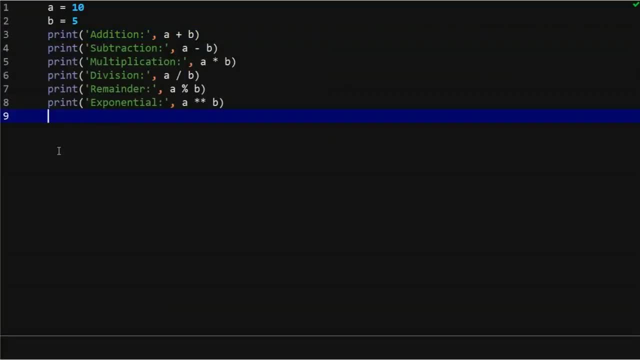 So you can see I have a is equal to 10 and B is equal to 5.. So I want to add, I want to subtract it, I want to multiply them using the star operator. The division operator is the flow division. Then we have the percentage which is for the remainder. 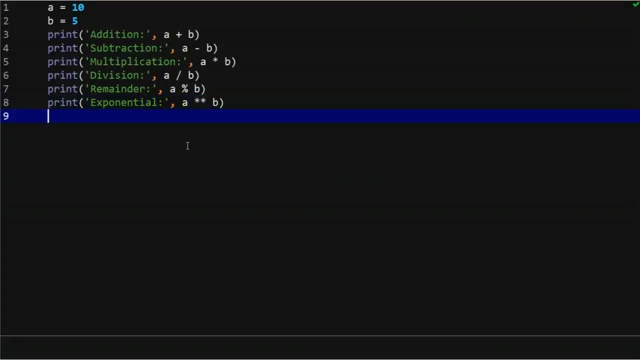 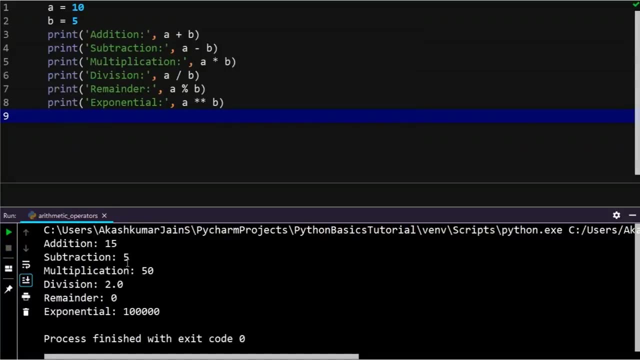 and two consecutive Is basically for the exponential. So let me run it So, as you can see, the addition is 15, subtraction is 5, obviously, because 10 minus 5 is 5. the multiplication is 50. 10, 8, 5 is 50, the division is 2.. 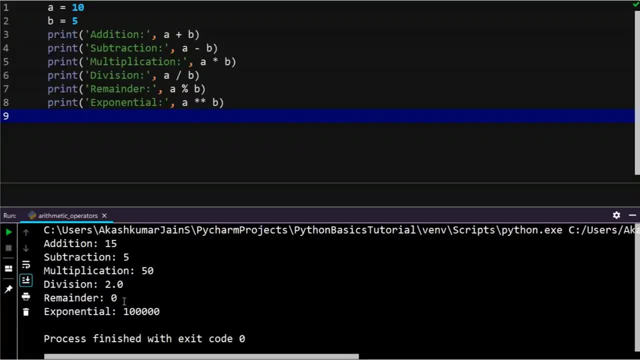 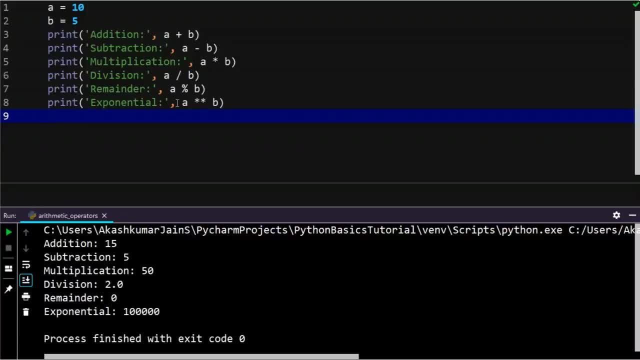 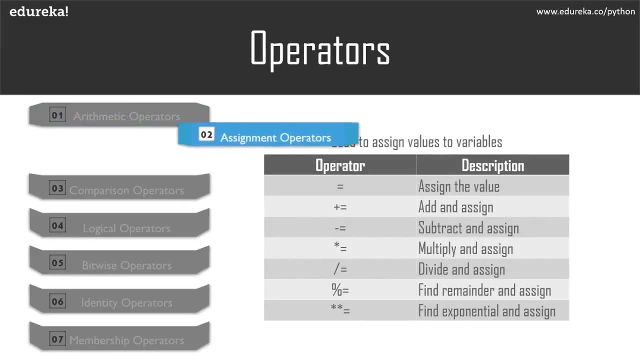 This is where we use the exponential part of operator. Let's move ahead with the next operator, which is the assignment operator. You would definitely know what the assignment operators are. It's because you have been assigning values to particular variables. So this is where the assignment operators are used. 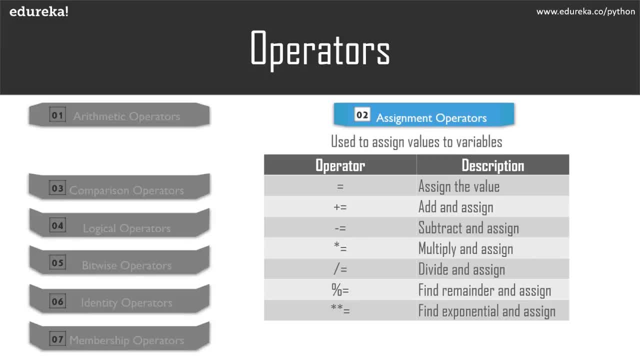 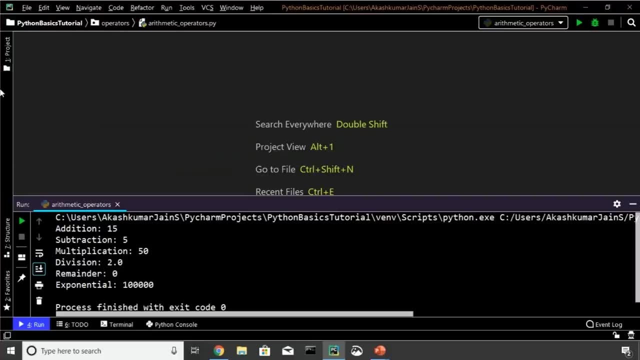 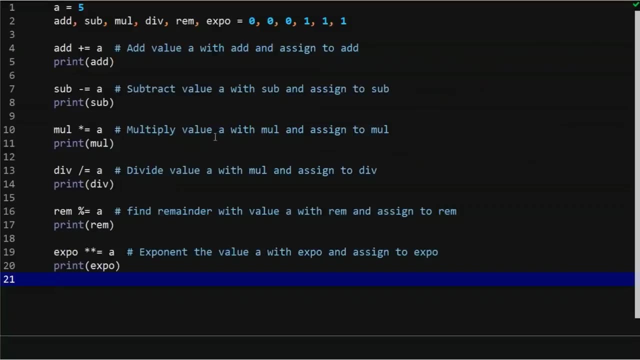 Now there are shortcut notations where you can add and assign, subtract and assign, multiply and assign and so on. So you can understand this better if we have our project Over here and we go to the assignment operators. and let me go to the presentation mode. 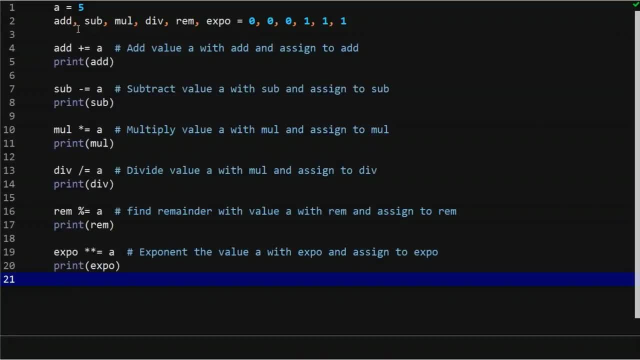 I have a is equal to 5 and I am giving values to these particular at sub mal and so on. So this is called as multiple variable assignment. Add will get the value 0, subtract will get the value 0, multiply will get the value 0, division gets one, remainder gets one. 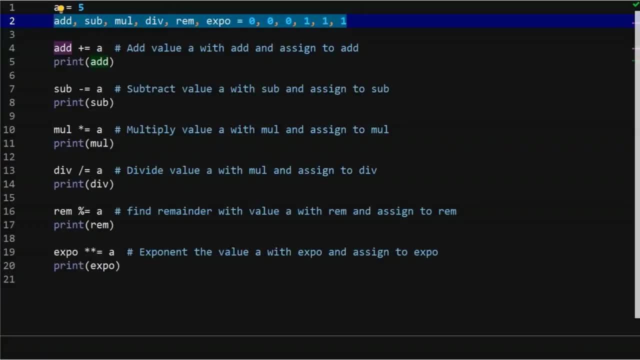 exponential gets one. now, if you were wondering why I have given division remainder and exponential, it's because I do not want error. I do not want to divide anything with 0 because that would give me an error. So let's just go ahead and understand what this does. 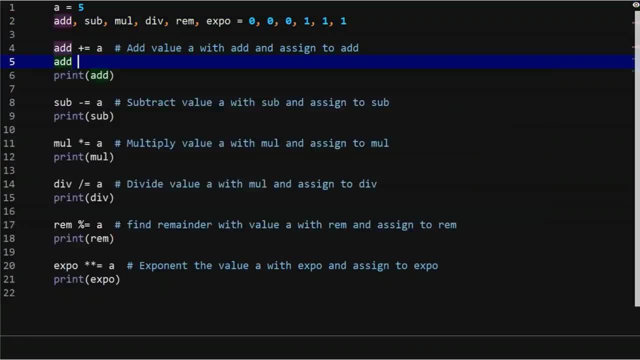 Let me write. what would I actually write for this? So add is equal to add plus a. so instead of writing this big statement, I can just say: add plus equal to a, which means that add is equal to add plus a. the same goes for subtraction, multiplication, division, remainder. 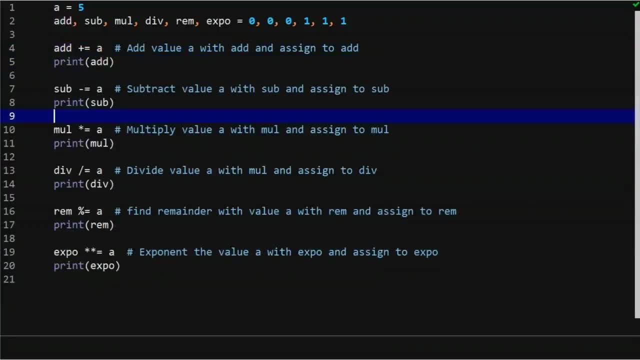 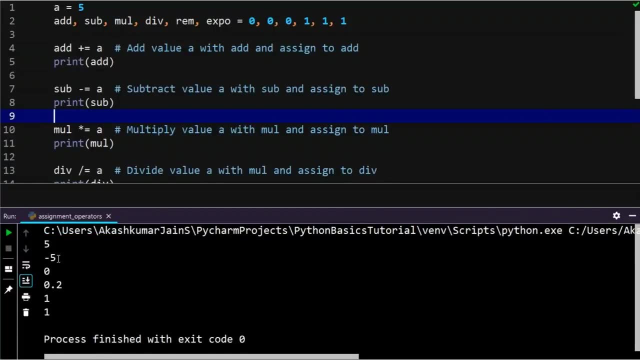 and exponential. So I hope you've understood that. So let me just run the program for you to see the output. So 5 plus 0 would give me 5, 0 minus 5 would give me minus 5, and we have multiplication, which is 0, into 5, which is 0. 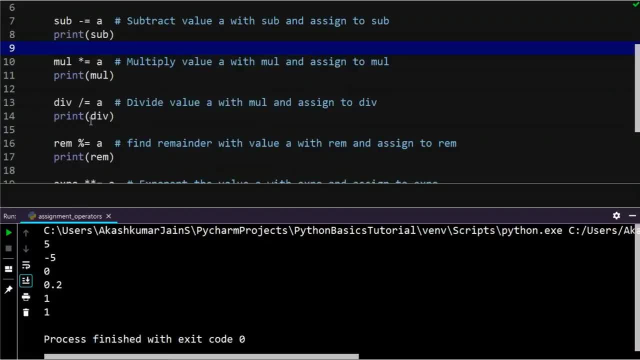 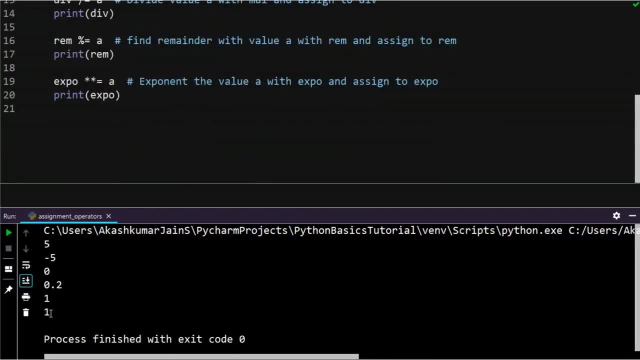 and we have the division, which is 1 divided by 5. So that is 0.2. Then we have the remainder as 1 and the exponential will be 1, because anything into 1 is still 1.. So we have finished the assignment operators. next, 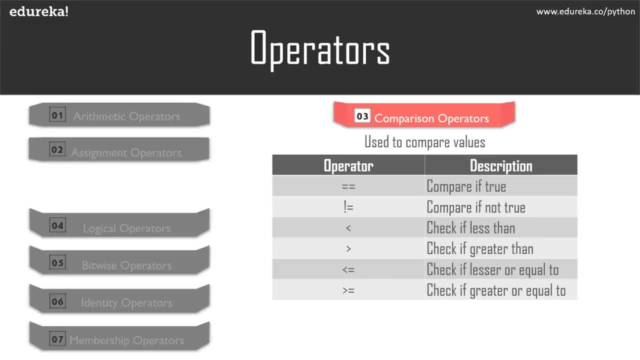 We have the comparison operators, So, as the name suggests, it is used to compare the values. So if Phi is equal to Phi, it will return a true, and if Phi is equal to 6, which will give us a false. So these are the various operators. 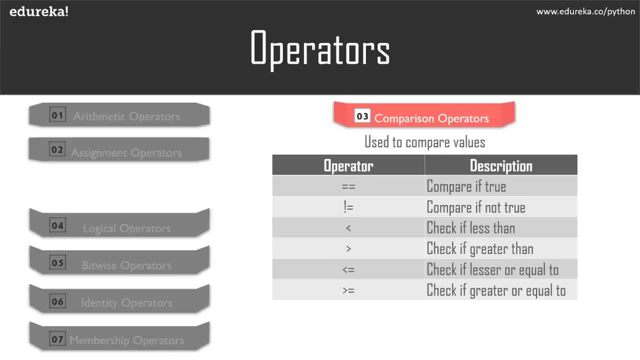 We have the double equal to to compare if it is true, not equal to to compare if it is not true, which means that if it is not equal, then we have the less than or greater than and less than equal to 1, greater than equal to. so let's move. 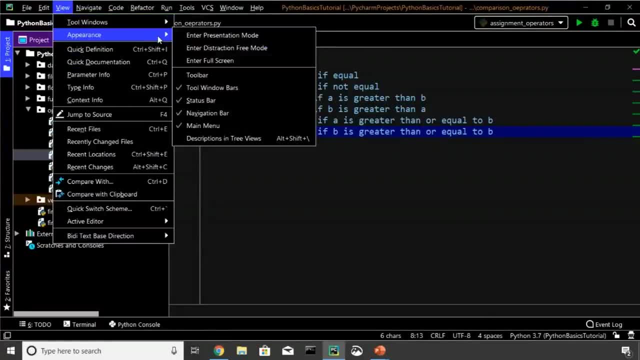 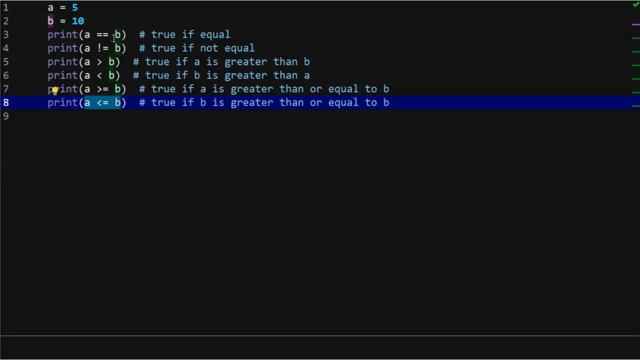 ahead to our program and go back to the presentation mode. As you can see, I have fire and 10.. So if I say a is equal to B, which means Phi is equal to 10. This will be wrong. That means I will get a false over here. 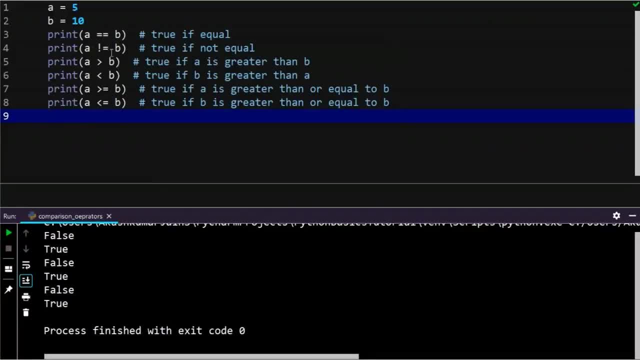 and then Phi is not equal to B, which is true. That means 5 is not equal to 10, which is true. That's why I have a true over here. Then if a is greater than B, so 5 is not a greater than 10.. 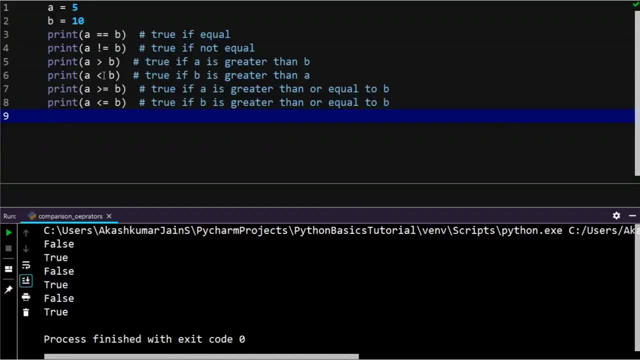 So I get a false. It's over here. So a is less than B, which is true. That means 5 is less than 10.. That's the reason I've got a true over here. the same thing over here to if it is greater than equal to, it will be true. 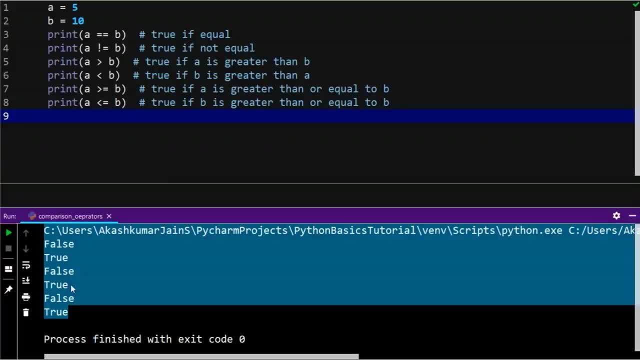 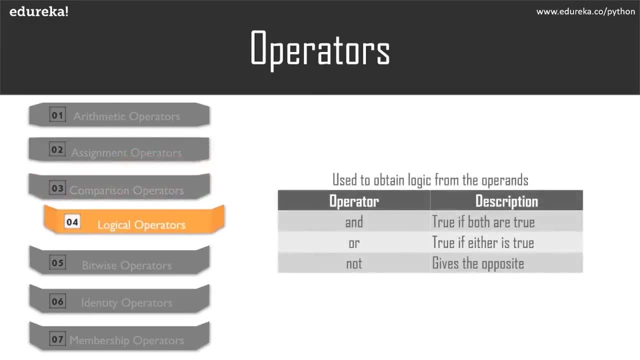 or if it is less than equal to it, will be true. So you can see the output accordingly. Let's move ahead to the next set of operators, which are the logical operators. logical operators are basically used to obtain logic, which means that if both the elements are true, 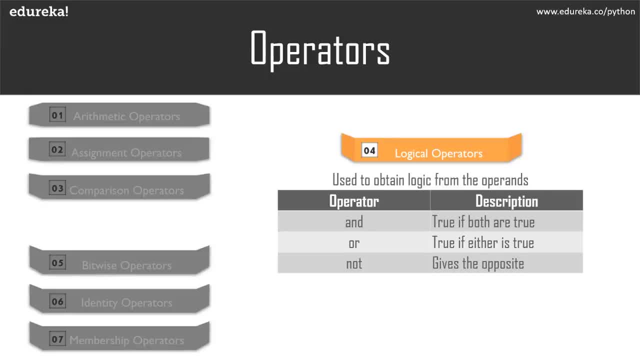 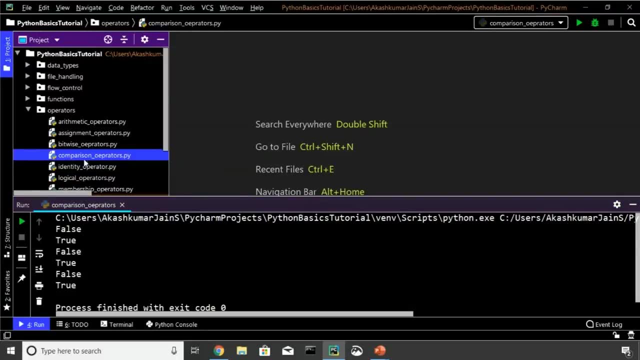 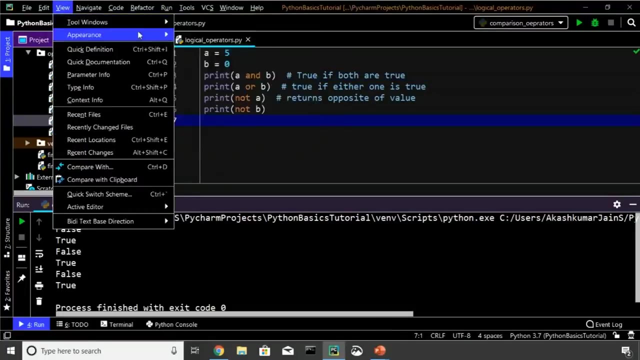 it will be true. If either one of them is true, it will give us a true, or if not, which means that give us the opposite of it. So let's move ahead to the Program over here, And let me go back to my presentation mode. 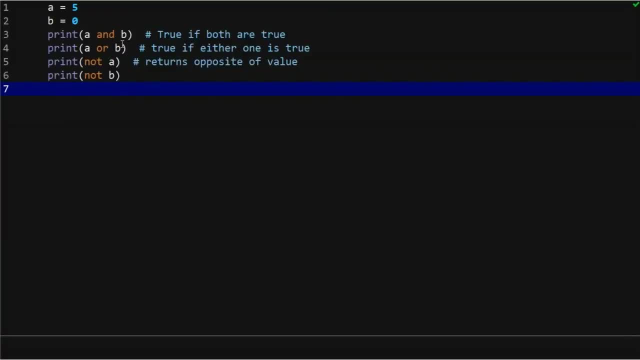 Yeah, so I have five and zero. So I'm seeing that print of a and B, which means that if both of them are true, this will be given a true. now you have to remember something: If it is 0, that means it is always false. 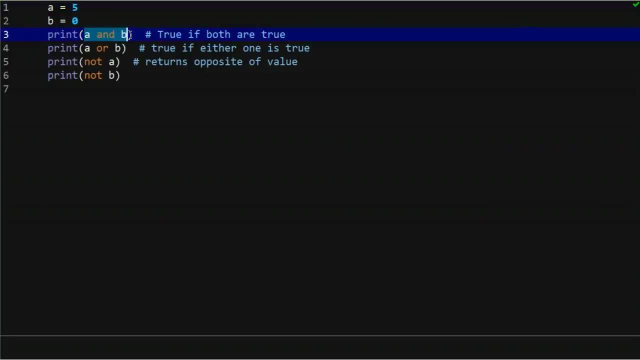 If it is 1 and anything greater than 1, it will be true. A and B will be 0, because this will give us a true only if both of them are true, and a or B, which means that it is either 5 or 0. 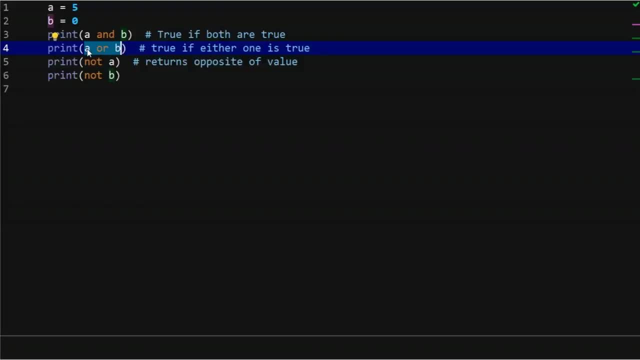 So this will also be a true, because I am having either one of them to be true. So not of a. this will give me false, because five over here is the value of true. So not of a. so not of true will be false and not of false would be true. 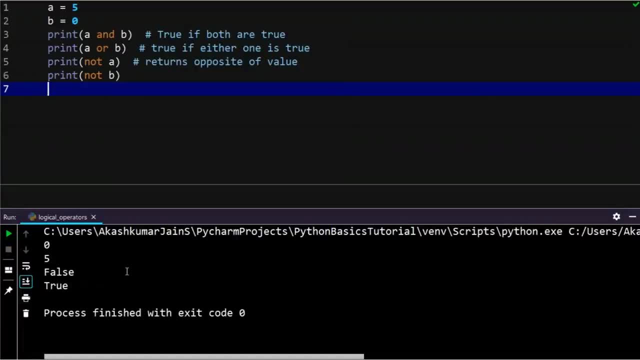 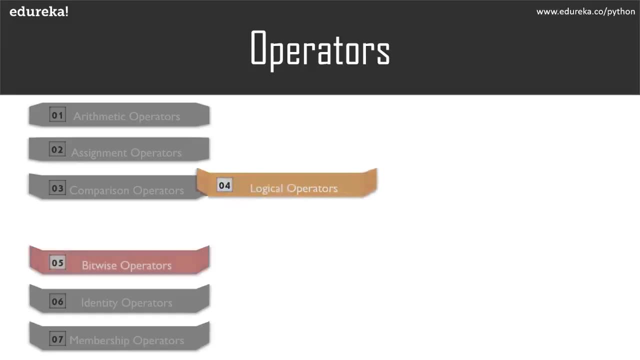 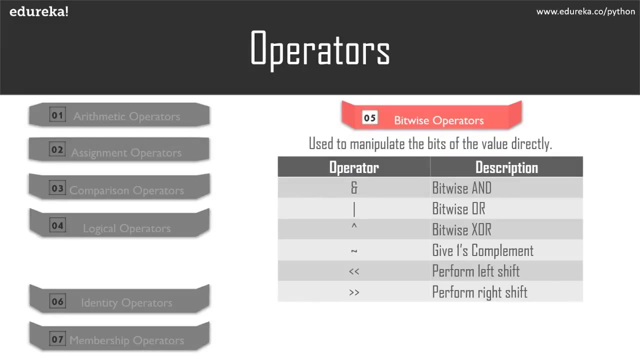 Let me run the program So you can see the output accordingly how we had discussed it. So now that we have understood the logical operators, let's move ahead to the next operators, that are, the bitwise operators. bitwise operators will be much more understandable If you know what the theory of bits is. 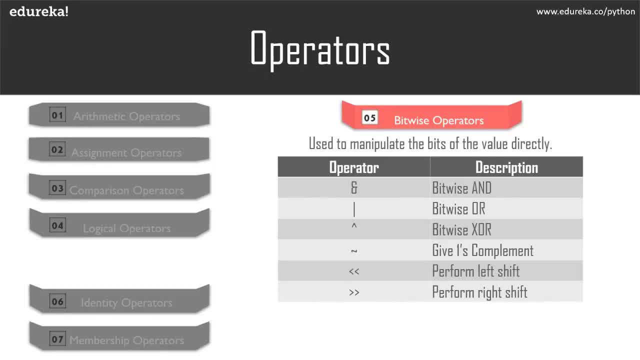 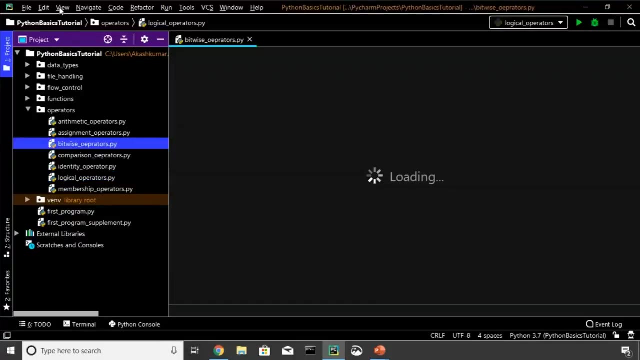 because they are basically used to manipulate the bits directly. So we have the bitwise and or X or once complement and the left shift and the right shift. Let's move ahead to our demo. It was the bitwise operators, and let me go back to the presentation mode. 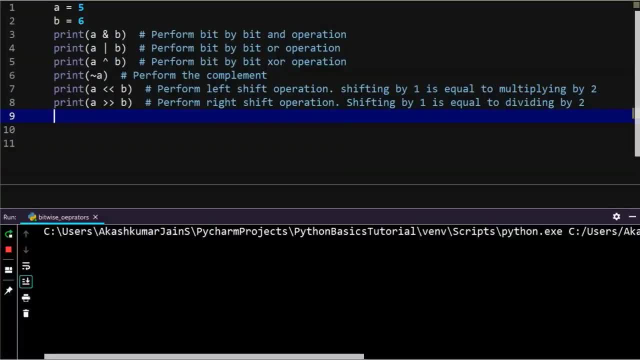 So let me just run the program for you. So if you and five and six, the number will be four. if you ordered, it will be seven, and then you have the X or operation that gives us the value three. So we have the not of a, which is the not of five. 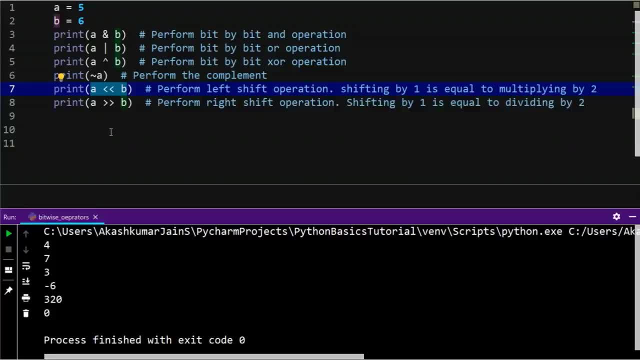 will give us the value six. So next we have the left shift and the right shift of Prater, which is equivalent to multiplying with two. So basically what this means is that you will be multiplying 5 into 2- 6 times. So whenever you have 5 into 2- 6 times, 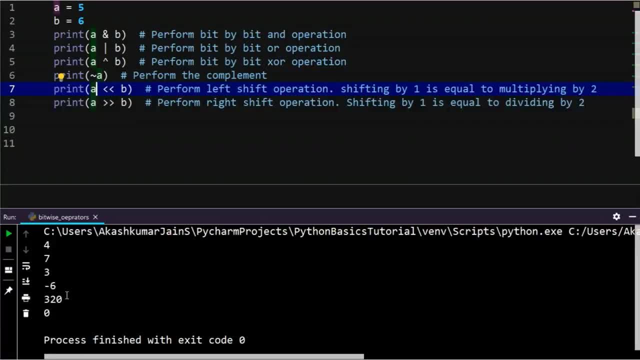 this will become equal to 320.. So it will be 5 into 2, that will be 10, 10 into 2 will be 20, and so on. That's how the calculation works, and then you have right shift, which is basically the equivalent of dividing by 2.. 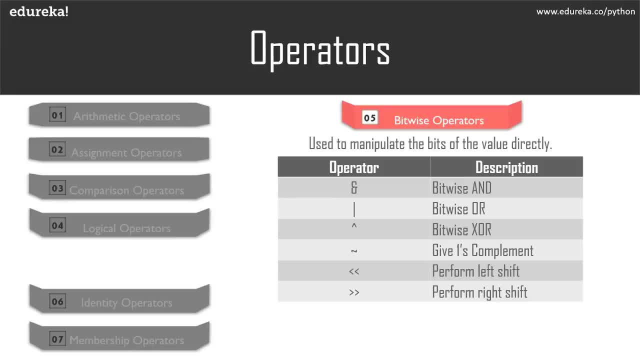 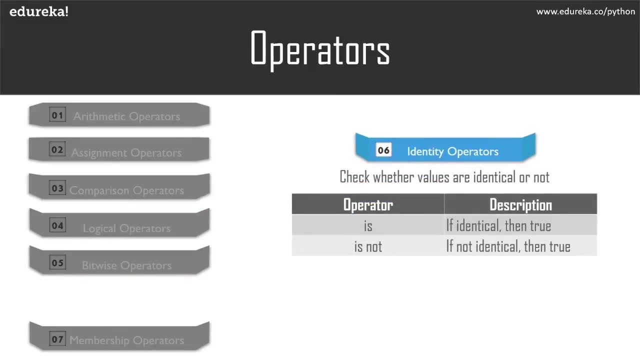 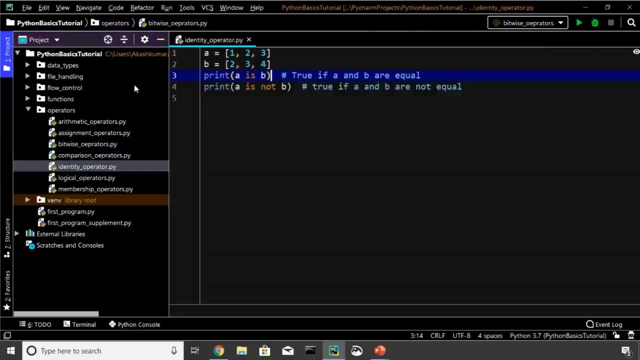 So we have the value as 0.. Let's move ahead with the next operator. This is the identity operator. So identity operator is basically to check whether two elements are identical or not. So let's move ahead to our program. that is the identity operators. 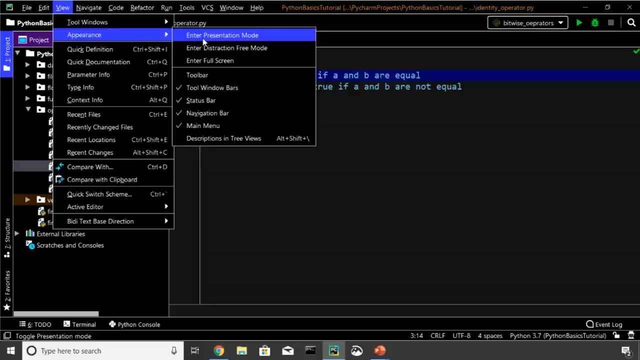 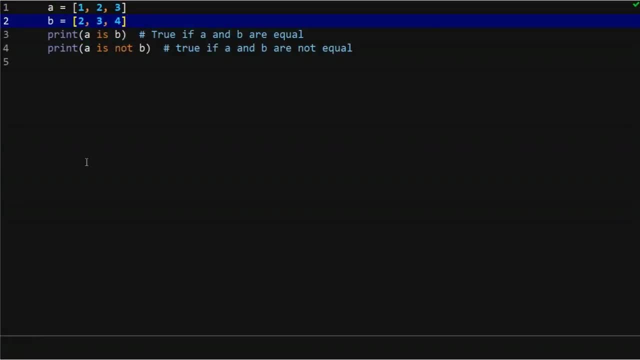 and move ahead to the presentation mode. So we have: a is equal to 1, 2, 3 and B is equal to 2, 3, 4. So is a equal to B. This will be a false and a is not equal to B. 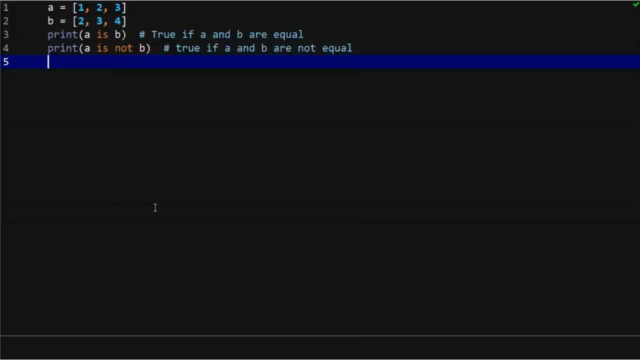 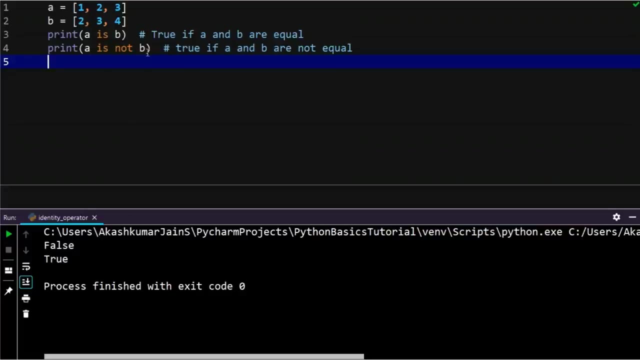 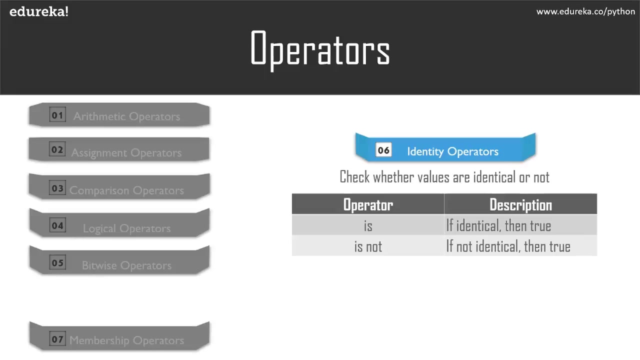 So a is not B, So this will be true. So outputs will be false and true because a is not equal to B and a is not B is actually true. So I hope you've understood. what are the identity operators? also, Let's move ahead to the last operator. 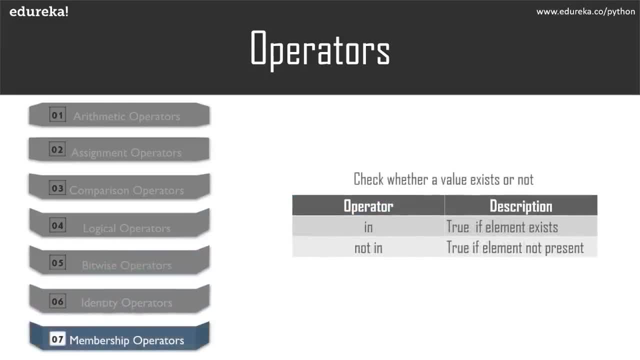 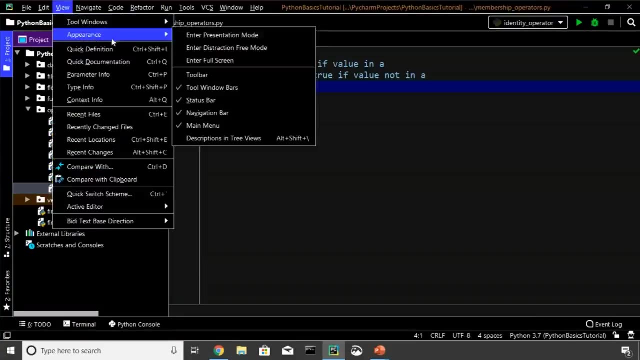 which are the membership Operators. the membership operators are basically used to check whether a particular element exists in another element or not. So we use the in and not in operators. So let me go ahead and open that up. So we have a is equal to 1, 2, 3. 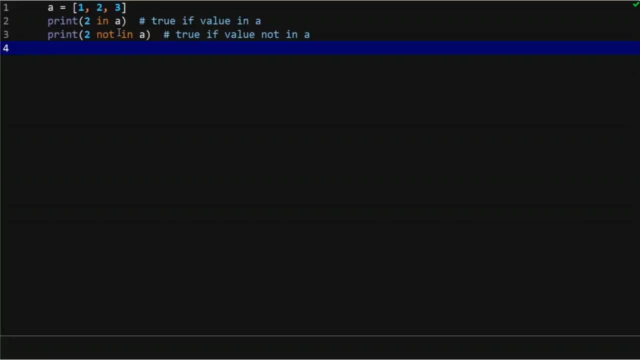 and I am asking: print if 2 is in a and 2 not in a, So print if 2 in a and 2 not in a, So 2 is actually in a. So I will get true and I will get a false over here. 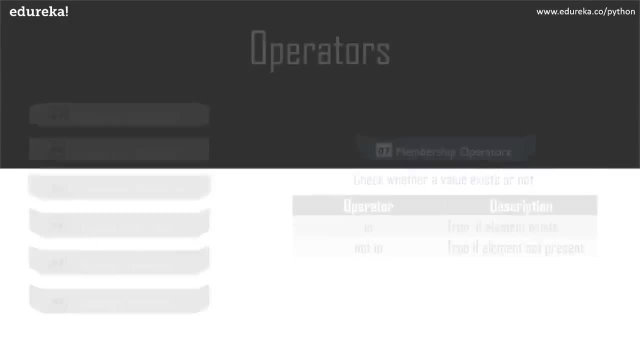 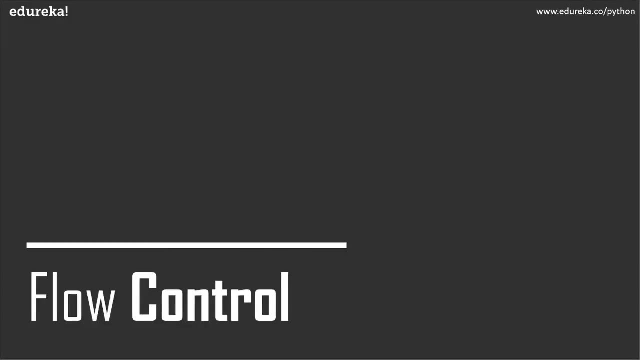 So that's what I have obtained. So that basically wraps up all the operators that we have in Python. Let's move ahead to the next topic, which is flow control. So by now you would have already understood that the program runs in a sequential manner. 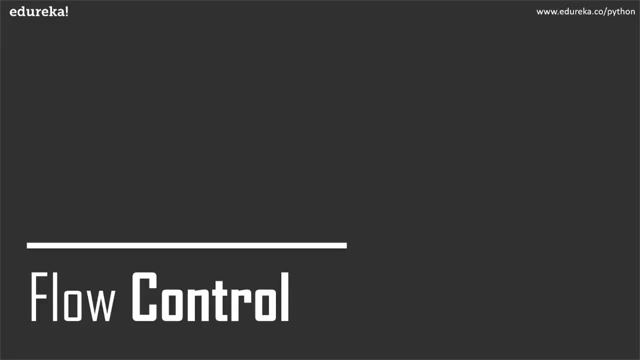 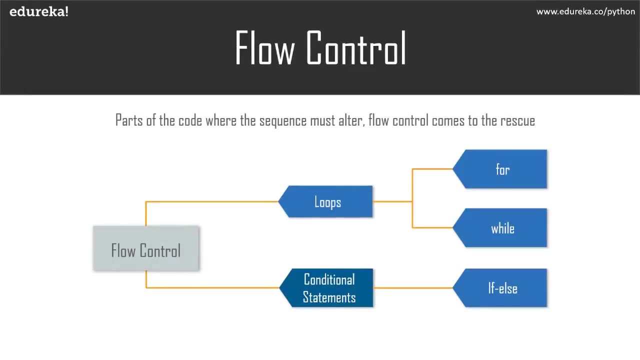 or the program's compilation is done in a sequential manner, That is, line by line. What if you want to break that way of compilation so that it can be according to your own advantage? That is why you use the flow control. So what is flow control? flow control is basically. 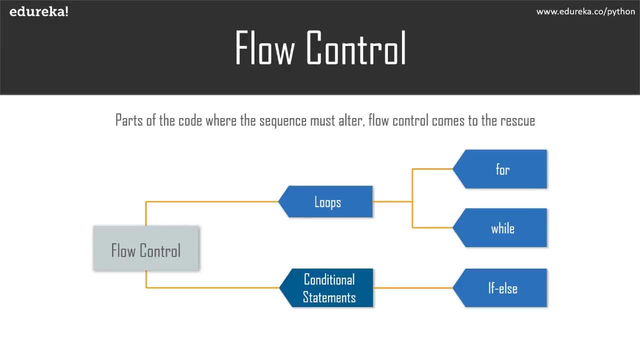 altering the sequence of your code. So how do you do that? That is done using either the loops or the conditional statements. So the conditional statements in Python are the FLs and the loops are the for loop and the while loop. So let's go ahead. 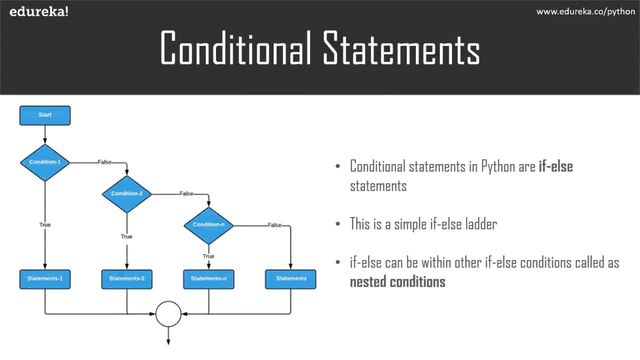 and understand what are conditional statements. conditional statements basically mean that if a particular condition is satisfied, you execute a set of statements or you may execute another set of statements. So let's say you are a user who are expected to enter a number and you can enter either a positive number 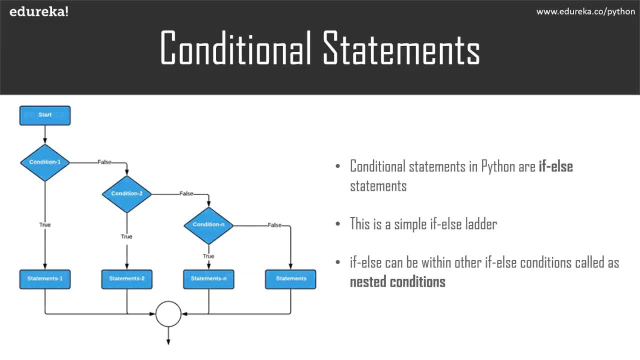 and a negative number, and you are expecting the output to say whether the number is a positive or a negative. So I basically can add a condition saying that if the number is 0 or greater than 0, it is a positive number or else it is a negative number. 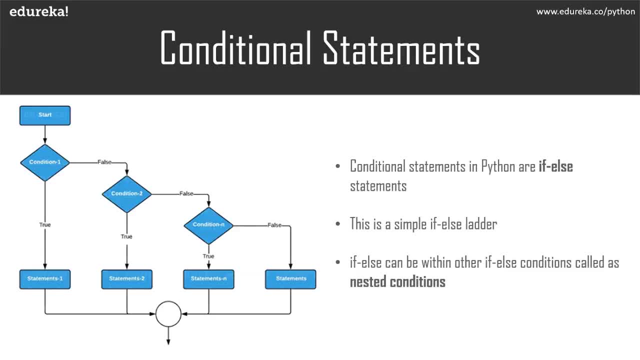 So this is basically a condition, where I am giving a condition and asking that if this condition satisfies, you execute these statements, else you execute these statements. So this is where we use the FL statements. Let me move ahead and show you our demo for this. 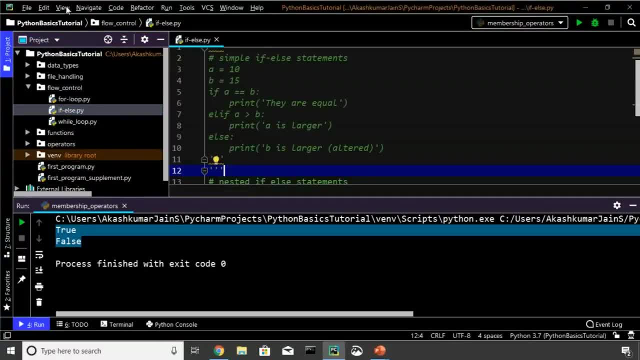 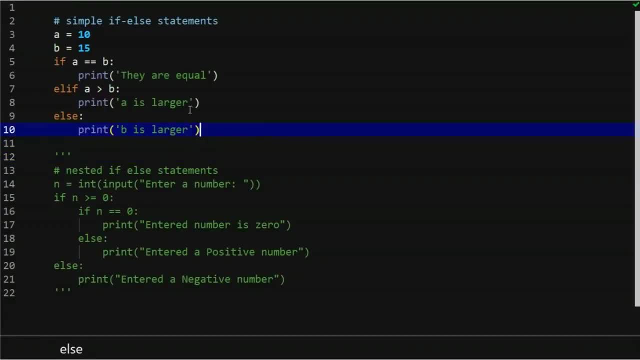 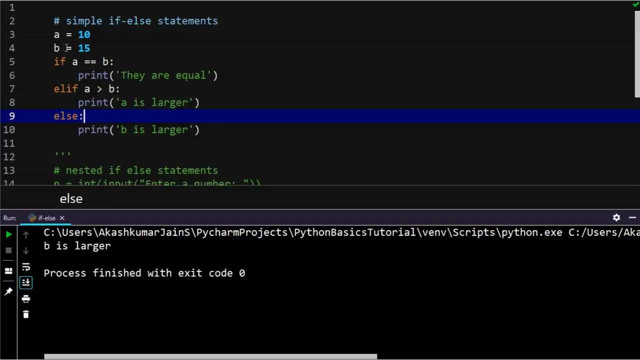 Let me close this up, open up, if else so, as you can see over here. Let me run the program So, as you can see, I have a is equal to 10 and B is equal to 15.. I'm just seeing that if a is equal to be print. 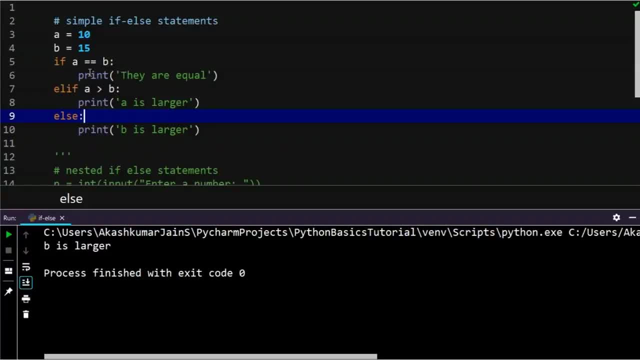 that they are equal. So now, this is where you will understand what indentations are. So in other programming languages we use braces to see which block of code comes under which part of if block or the for loop or something like that in python. 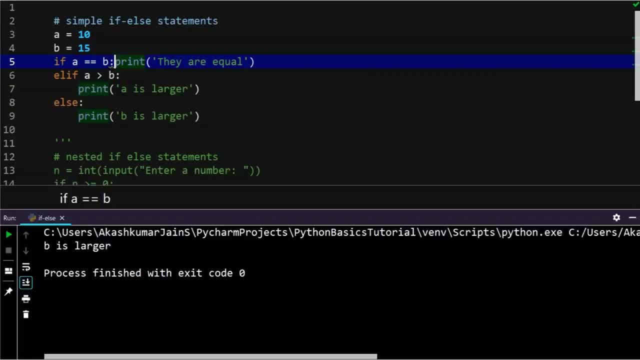 It's not in that way. It is basically using indentations. So how do you write the if statements or any other statements? it is using the keyword. So over here, if is the keyword, and then a is equal to B is the condition, and now I want to say the set of statements. 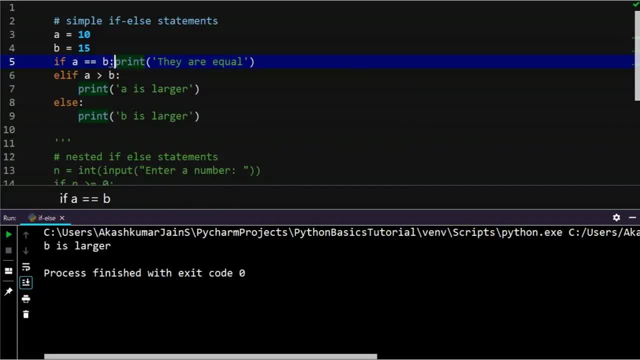 that have to be written under this. So I just do a colon and then, in pie charm, you do not need to worry, because if you hit enter, it will automatically intend it. So, as you can see, this is now four spaces, or one tab space, right? 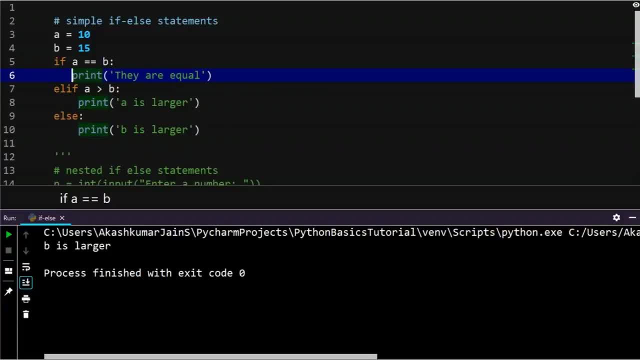 So let me just count it for you: One space to space, three space and four space. four spaces is how you can see that this particular statement is under the if block or directly. you can just give the tab and it will automatically take care of it. 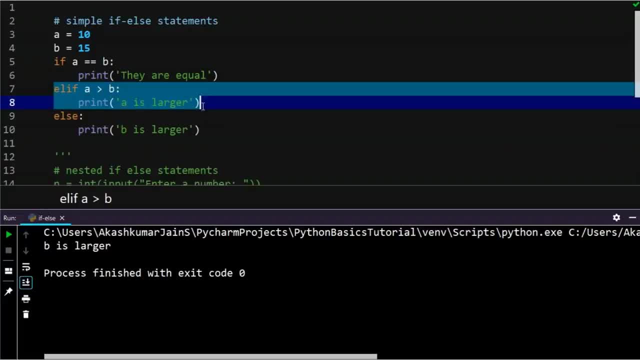 And then you have the else, if, which is to see the other if conditions. so the same way with the colon, and then print: a is larger and then else, which is if all the conditions that you have written are not working, you just have to execute a certain 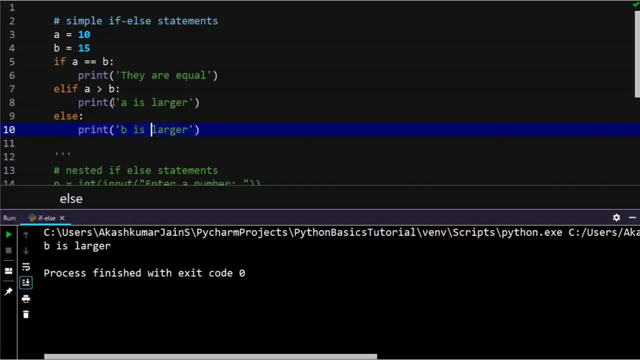 I'm out of statements, so that comes under the else block. So, as you can see, a is not equal to B, So this will be skipped. then is a greater than B, So 10 is greater than 15, which is false. So this is also skipped. now. 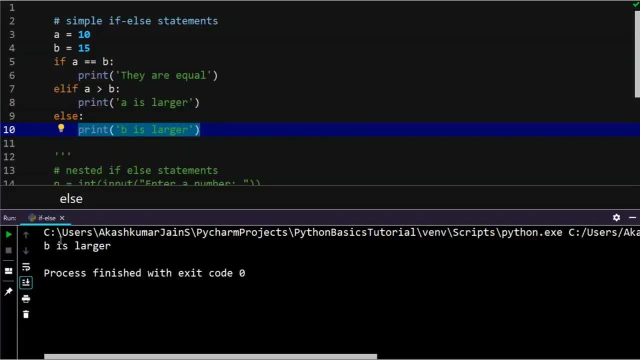 I go down and finally see that B is larger. So that's the output that I get over here: B is larger. I hope you've understood how the if and else statements works. These are really simple to understand, but they can become much more complex according 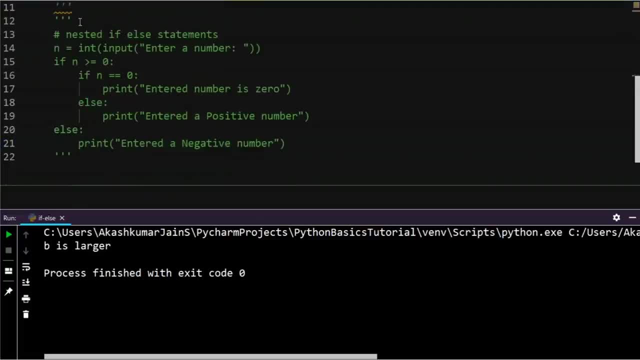 to your applications in the future. So let me just show an example of nested, if else blocks. Let me go ahead and run this. So yeah, I was seeing as an example. you enter a number if it is greater than equal to 0. 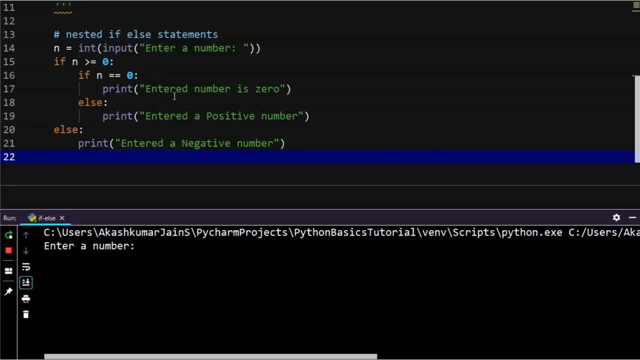 So here I am checking if it is equal to 0.. I just say that the number is 0, else It is a positive number. So let me go ahead and show this to you. So if I enter 10, it is a positive number. if I enter 0.. 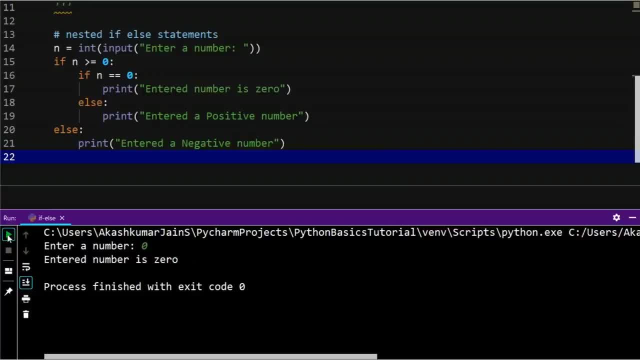 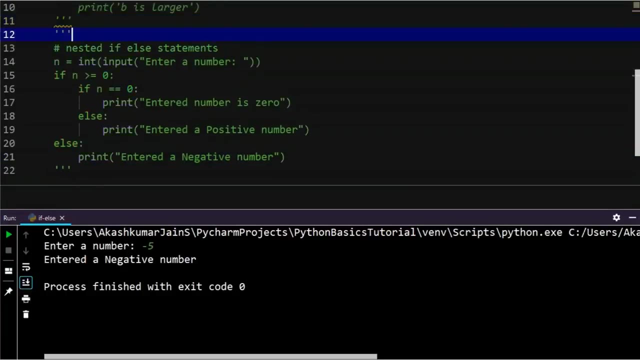 It is 0 over here and if I give a negative number, say for example minus 5, hit, enter, enter. it is a negative number. So I hope you've understood what are nested if else blocks also. that basically wraps up our if-else statements. 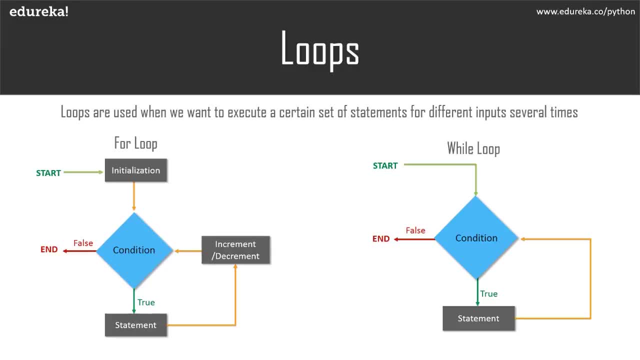 Let's move ahead with loops. loops are basically used to execute a certain set of statements for a different set of inputs for several times. That is where you use loops, For example, if you have an addition statement that you want to keep adding accordingly. 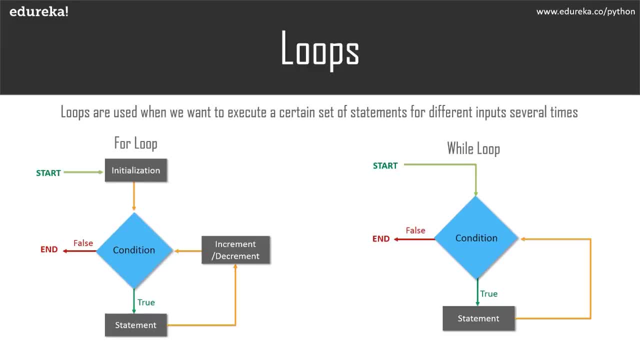 but it has to be done for 10 times, 15 times, 20 times. You would not sit down and write every ad statement accordingly. So this is where you use loops, because loops are basically used for breaking down the redundancy and to make the code much more smaller. 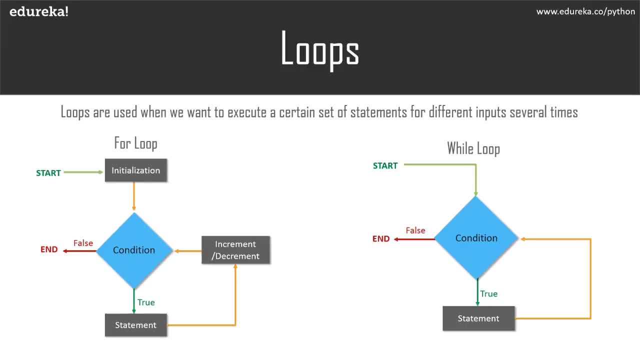 So we have two loops in Python that are the for loops and the while loops. So the for loops will have your initialization and all your increment decrement operations that are being done exactly in the first statement, So you do not need to explicitly do the condition updation. 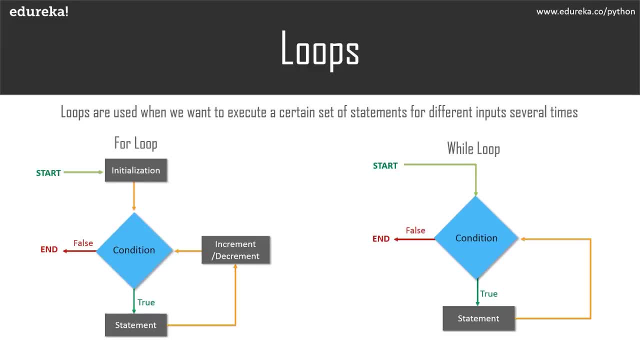 whereas in the while loop you would need to do the condition updation so that you can terminate the loop. So the for loops are used whenever you know how many times you have to execute a certain set of statements, whereas in the while loop you may not necessarily. 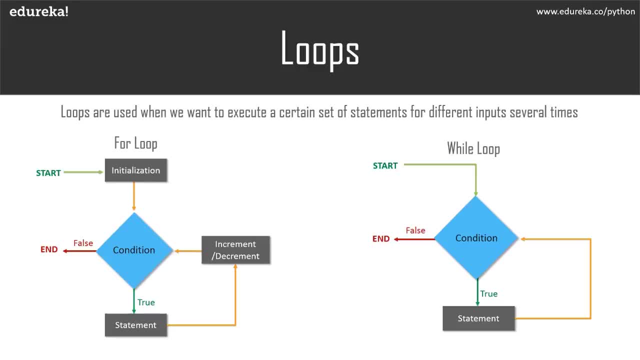 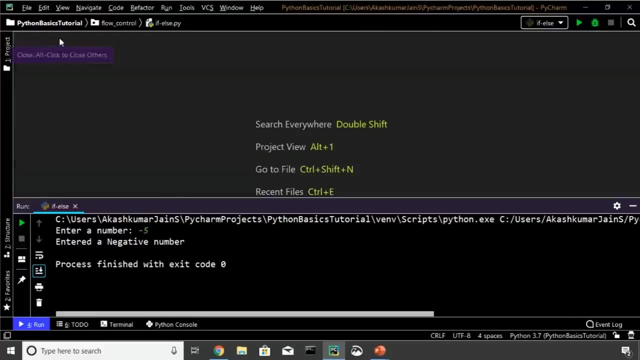 know, and that's the reason the user is given the option to explicitly change the conditions inside So that he can terminate the loop. So let's go ahead and go to our program. Let's go ahead with the for loop first and let me open while loop also. 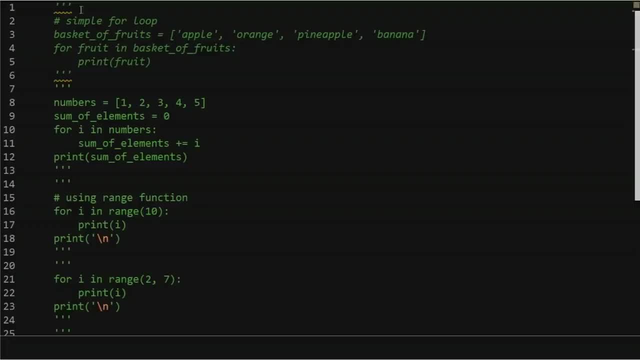 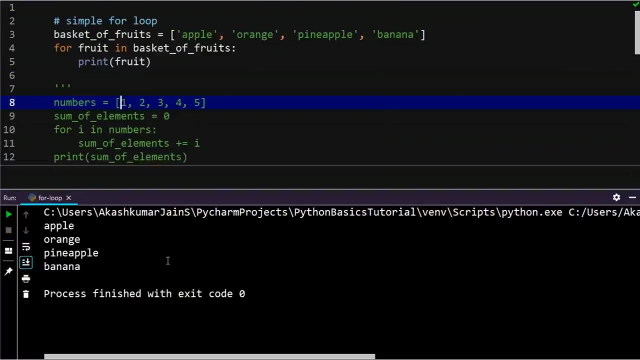 and so let us see how a simple for loop works. Let me just uncomment what is not required. So, as you can see that I have a basket of fruits, which is a list of all the fruits that are apple, orange, pineapple and banana, and I am seeing 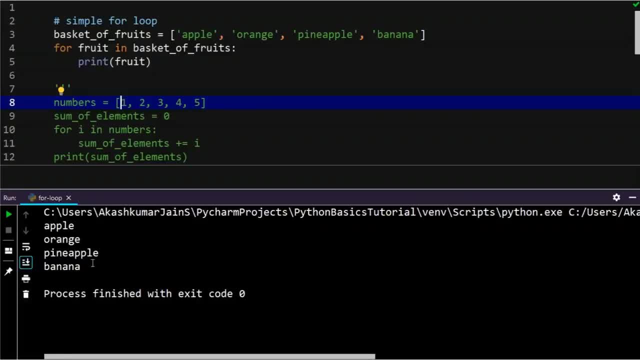 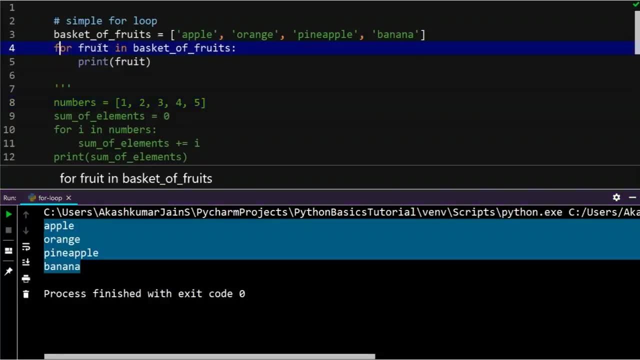 that for the fruits in the basket of fruits, just print the fruit as the reason. I have the output like this. So as you can see how the for loop is written for the particular variable in the particular list, with the colon and with the indentations over here, 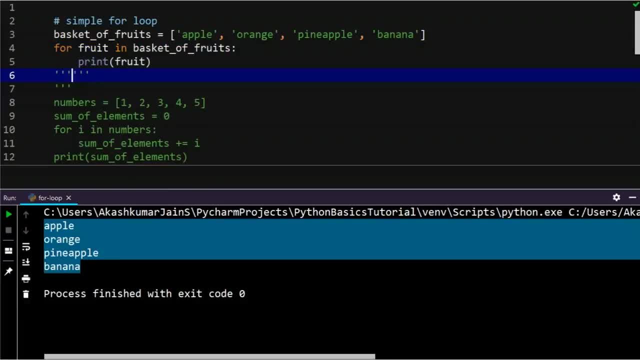 So I hope you've understood how this works. Let me just give you another example so that you can understand how and why you should also use loops. So let me just uncomment all of this. Yes, so I have numbers 1 to 5. 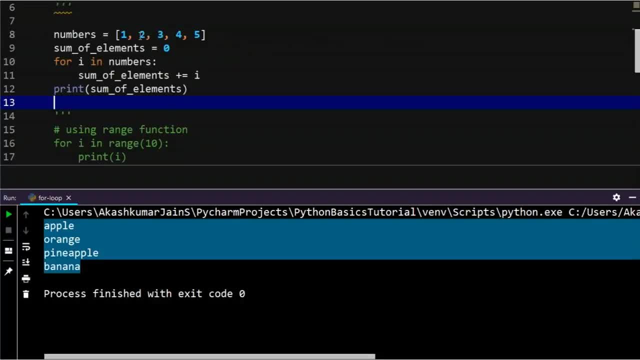 and I am seeing that I want to add all the numbers in this particular list. So if I would have to use explicit statements where I add each number, it would become very much longer for me. So instead of that I just say for I in the numbers some. 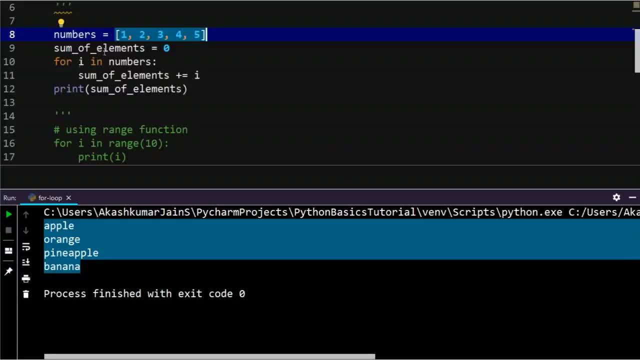 of the elements is equal to plus equal to of I. so if I will take the value 1, then I will take the value 2, which will become 3, then it will become 6, then it will become 10 and then 15.. So let me go ahead and run the program. 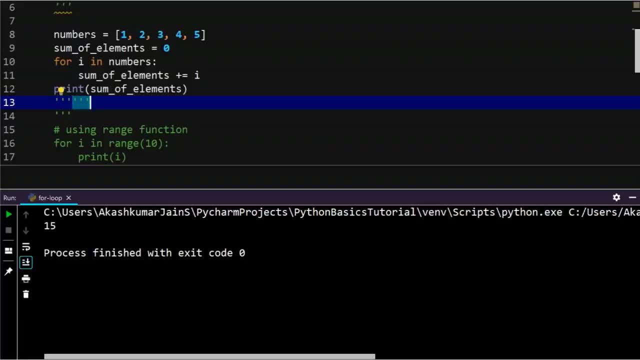 So, as you can see, 15 is the output that I have obtained. as you can see, instead of five statements, I just had to write one statement and my work was done. So next, let me show you something called as the range function. So range is basically used to give a particular set of variables. 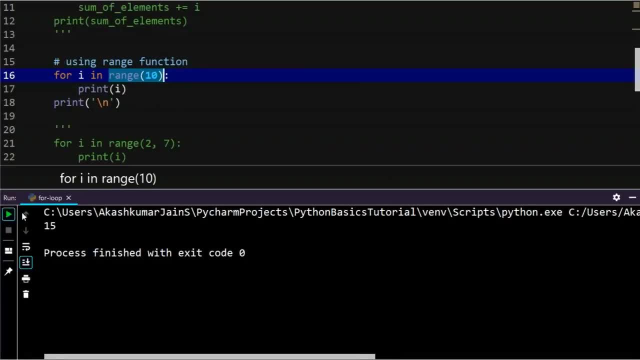 So if I say range at 10, it would basically mean that the numbers from 0 to 9.. So, as you can see, I have obtained the number 0 to 9.. Let me go ahead and uncomment the next part of the range function. 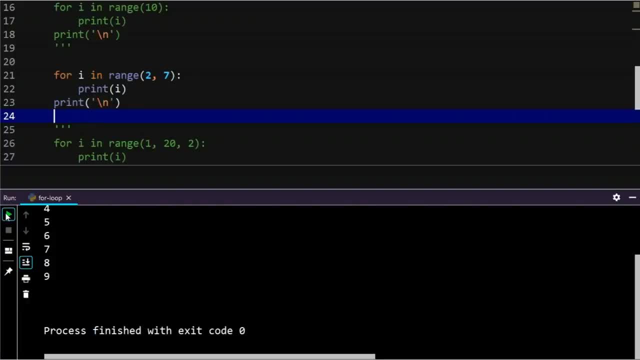 And let me run the program. So it is from range 2 to 7.. So it will be from numbers 2 to 6.. So I hope you've understood that also. and I have another range function here with the skip element, So let me go ahead and run this. 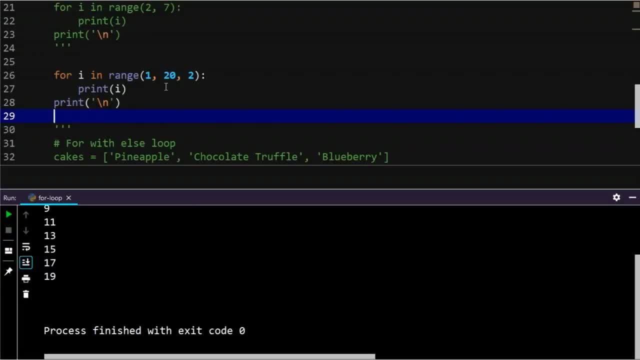 So here I'm seeing that I want the elements from 1 to 20, but I want to skip the elements in the numbers of 2 as a reason. I have 1, 3, 5, 7, 9, up to 19.. 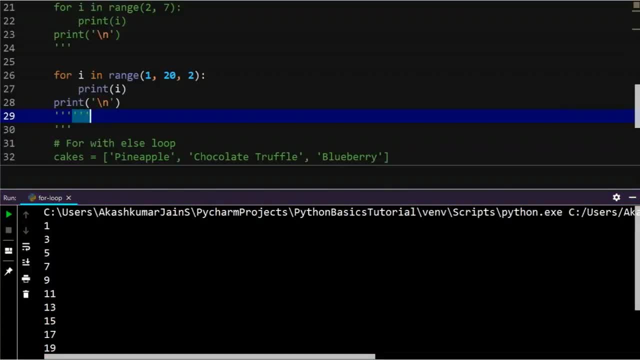 So this is how the range functions work. They may be used for your applications, accordingly to how you want it to work. And then we have the last for loop, which is the for, with the else loop. So basically, what this means is that if you have a for loop, 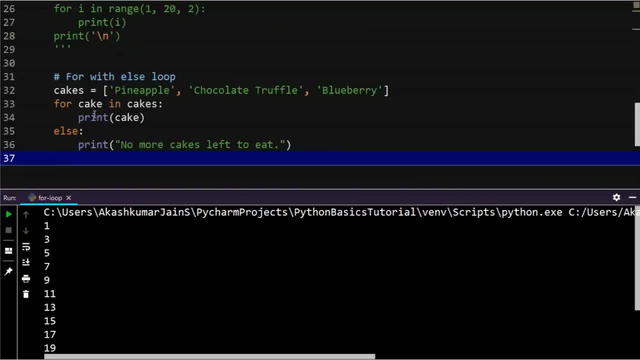 and that condition is true, it will always execute the for loop. once the for loop becomes false, The else statement will be executed. So let me just show it to you. So I'm seeing that. how many cakes are there? print all the cakes. 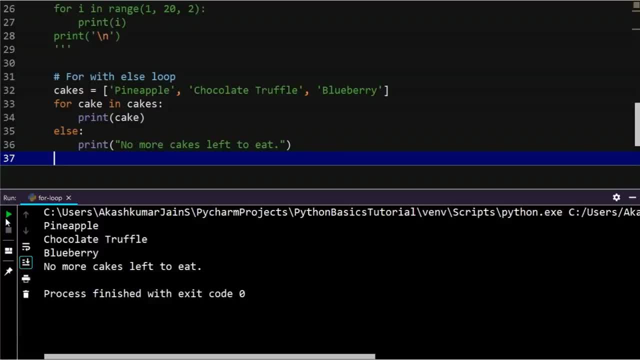 So I have pineapple, chocolate, truffle and blueberry, and then there are no more cakes left to eat. Once the for loop is false, the l statement will be executed, So I hope that also clears up ways in which how you can use the for loops. 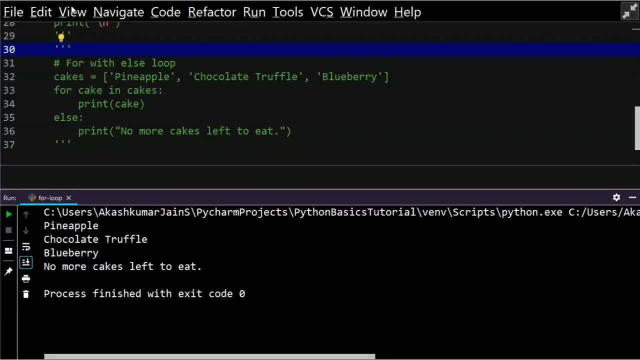 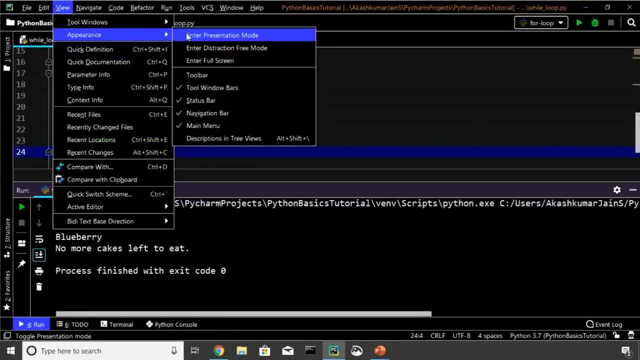 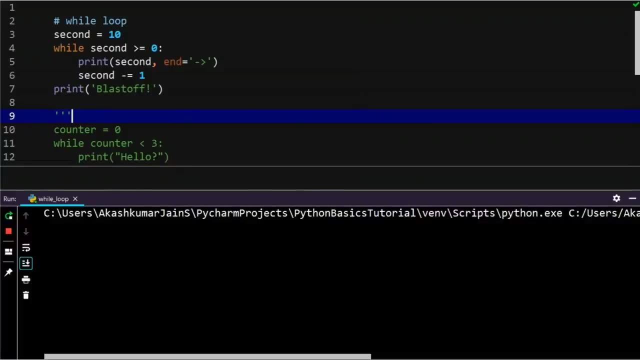 that basically wraps up for loops for us. Let me go ahead and exit the mode. So let's go ahead and understand what are y loops. So let me just run the program for you. So, as you can see, I have seconds equal to 10. 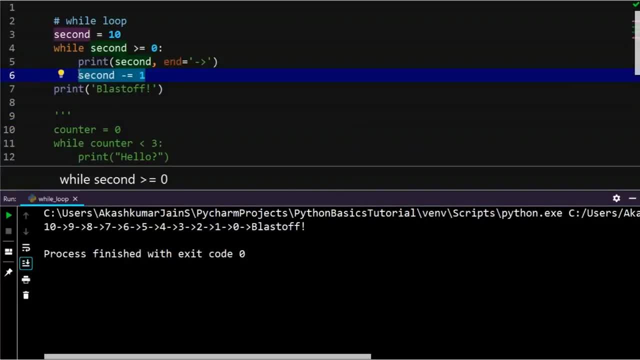 but here is where I am explicitly changing the condition, because here, if you see so, as you can see over here, that this is the condition but there are no sort of, you know, iterations or changes to the conditions. the conditions I have to be changed by the user itself. 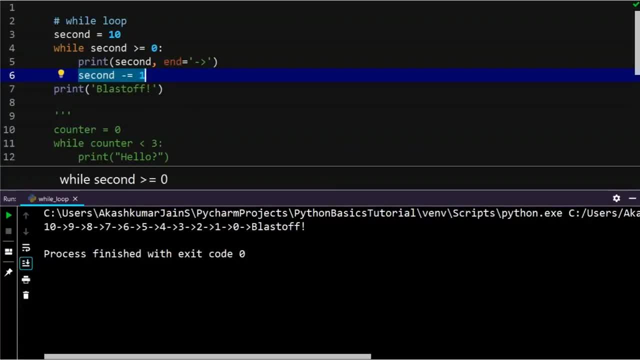 and that is what I have done here. So I'm just printing the second and once the loop is done, I just print the blast off. So, as you can see, this is basically a countdown and you get up to 1, 0 and then the blast off. 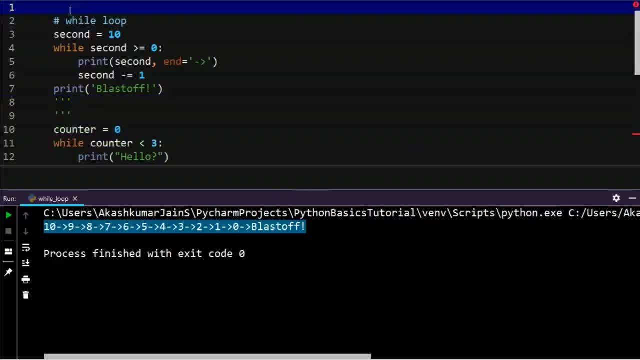 So I hope you've understood how the while loop works. These are really simple examples. keep practicing more and more to understand how these work. So next we have the while and the else loop, So it is basically the same concept of the for else. 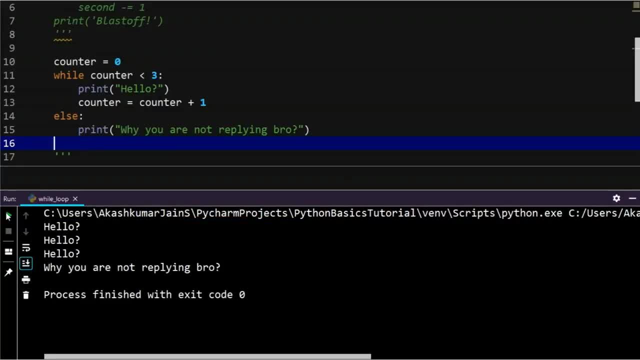 Loop where, if the condition is true in the while loop, you execute those statements as you come out of the while loop and then perform the else loop condition. So it's basically saying hello, Hello, Hello three times and then asking: why are you not replying next? 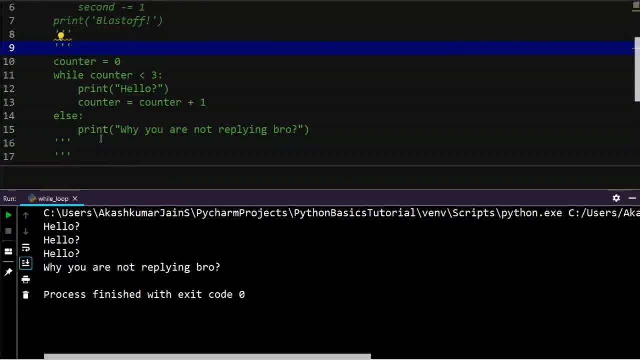 We have something called as the nested loops, So you can have different sort of loops. You can have for loop within a for loop. You can have for loop within a while loop. You can have while loop within a while loop. You can have for loop and a while loop- anything. 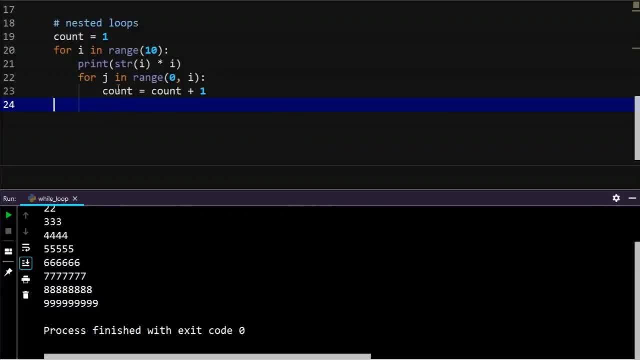 like that is possible. So I'm basically printing a pyramid over here. So, as you can see, this is how it works. You will understand more about nested loops If you keep working with them. that basically wraps up our loop session. Let's move ahead to the next topic for the tutorial. 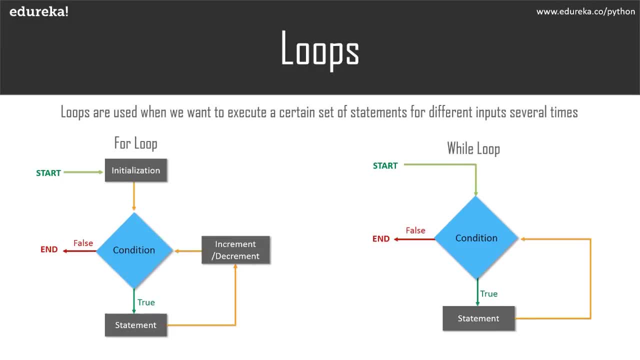 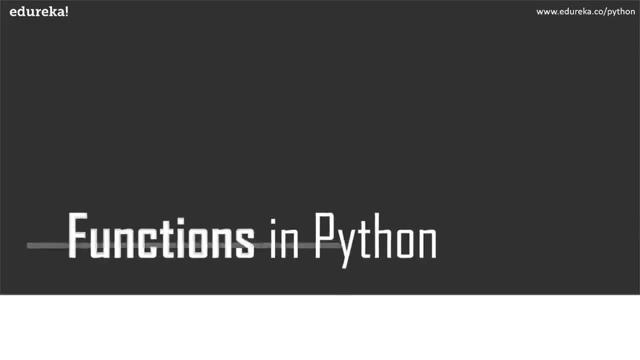 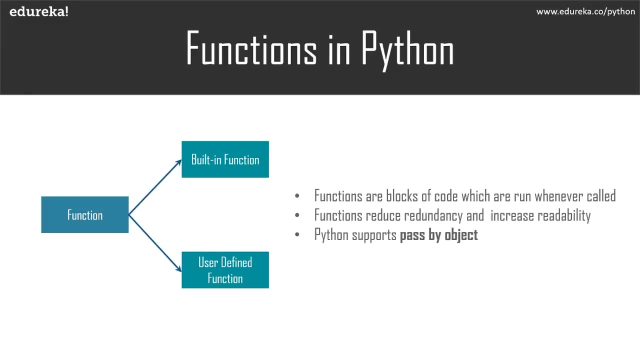 So I hope you've understood what flow control is and how you can have the conditional statements and the loops. So let's move ahead and understand what are functions in Python. functions are basically blocks of code which perform a certain particular sort of application and they can be run whenever they are called. 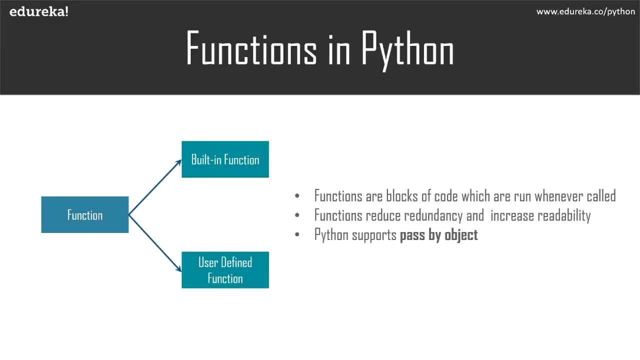 So why functions are required? because functions reduce the redundancy and they increase the readability, and there is something called as pass by object. If you are an old-school programmer, you would know that there is something called as pass by value and pass by reference. Well, Python accordingly supports pass by object. 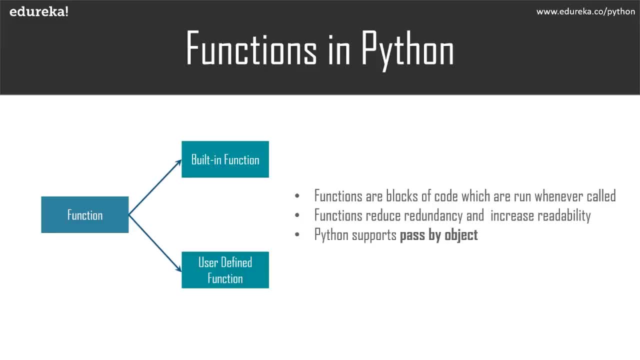 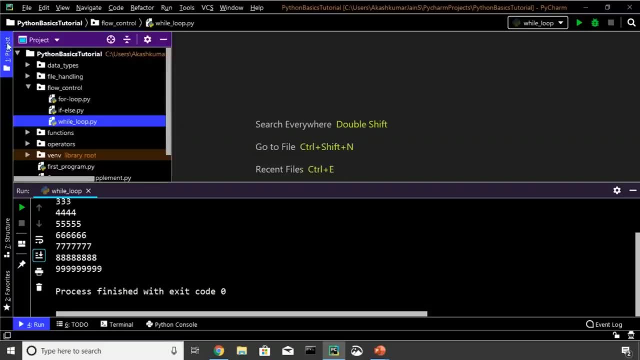 which means that it creates an object whenever a particular function is being called and then, accordingly, does the work. So let's go ahead with the tutorial so that you can understand all of this better. So we have functions over here and I have a pass by. 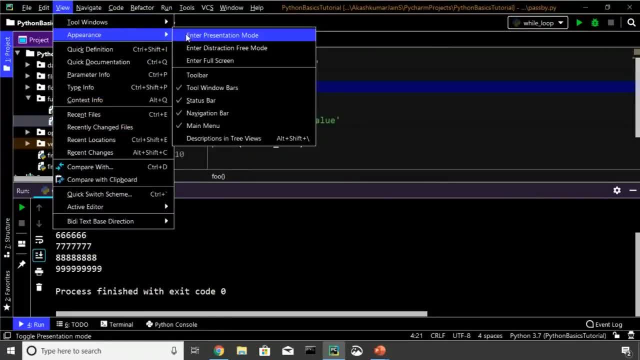 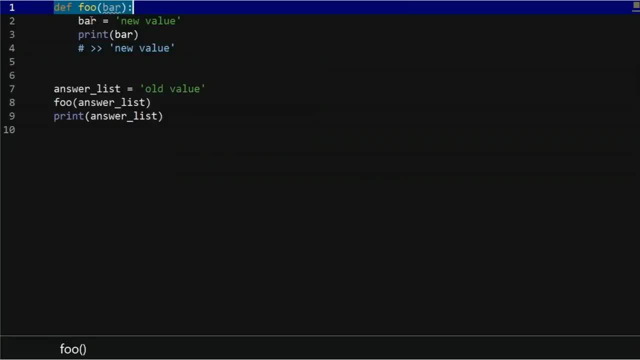 so, basically, what is pass by object? Now, as you can see, I have defined a function over here which is defined for bar and I'm seeing that bar is equal to the new value and print the bar and I have answer list which has an old value. 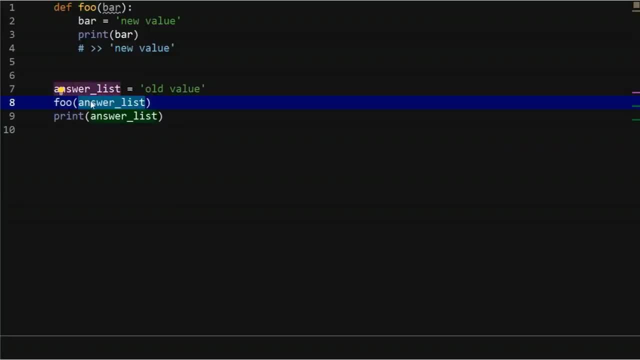 So I'm just seeing that foo of answer list. So now I am passing the answer list, which has the value old value inside it, and then passing it over here. So now, if you can see, the answer list will not be changed. Why is that? it's because this answer list. 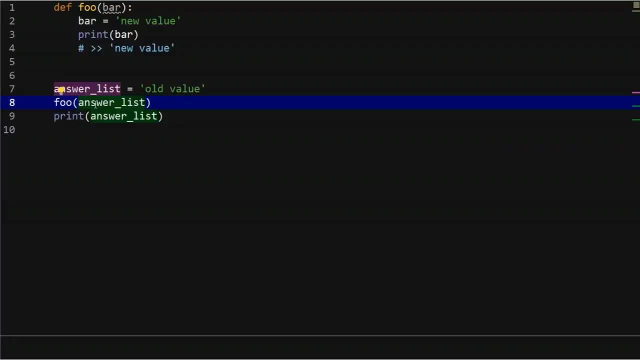 which is being passed is actually a new list or it is basically a new object? as you can see, I have the answer list which has the old value, and I pass that into the foo function and I will print it. So what basically happens over here is now. 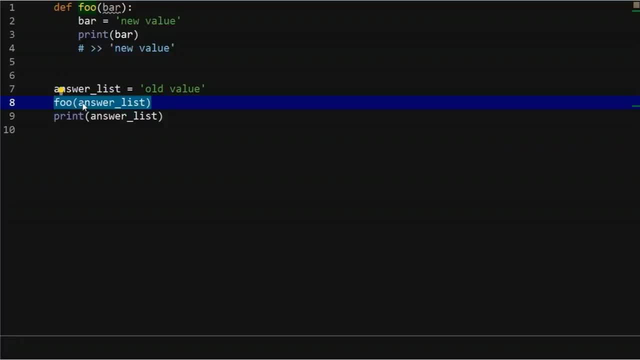 whenever this particular function is being called, this answer list is now being created into a new object, So this answer list is a new object and this answer list is another object. Now this answer list object is being sent to the foo function, where it is being changed into the new value. 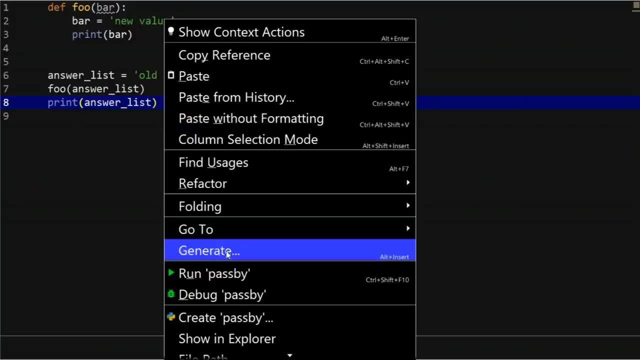 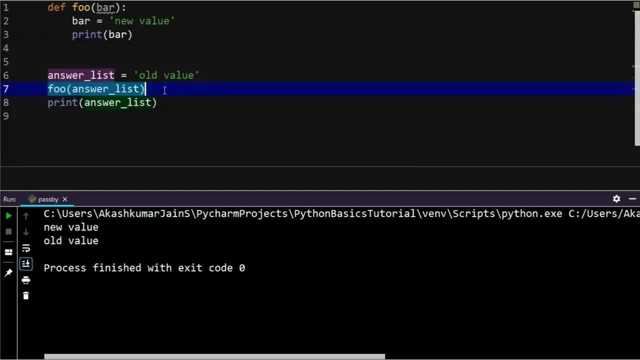 and if I print and now if I run the program for you. so now, if you can see the old answer List which was there, is not being manipulated where, as the new object was created, when the foo function was called and that was sent and that value was being changed. 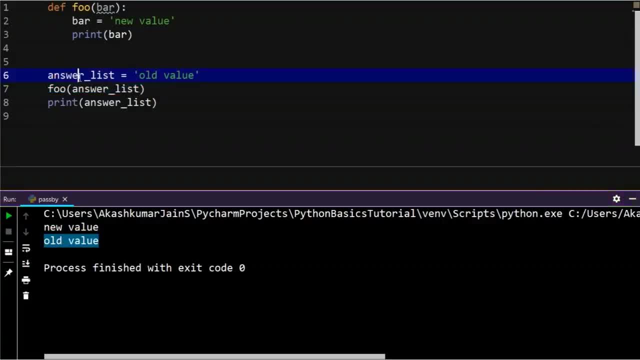 So now we have new value and the old value. So that is basically what pass by object means. You would understand it better if you keep going on programs and understand how each object is being handled by python. Let's go ahead and go to the functions. 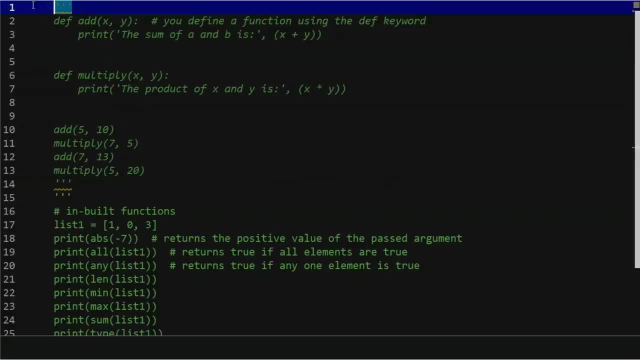 which is our tutorial. Now, if you can see over here, I have two functions over here which is used to add and multiply. So I basically give the parameters or I pass parameters to the two functions and see that I want to add them or I want to multiply them. 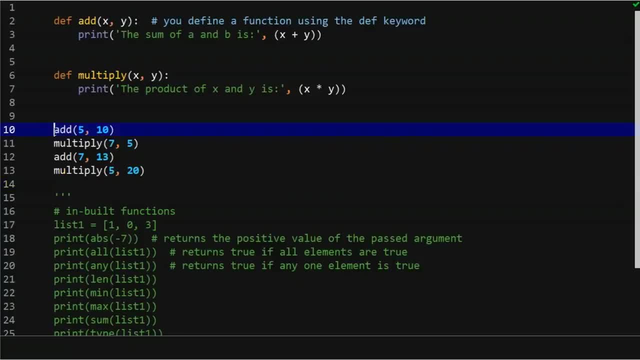 So, if you can see, over here I've just added one statement, which is: add 5 comma 10, multiply 7 comma 5, add 7 comma 13 and multiply 5 comma 20.. Now just imagine if this was not four lines. 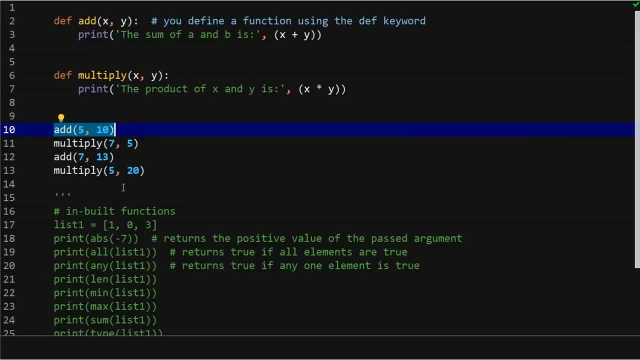 but 40 lines, you would need to have the sum of a and B, sum of a and B, product of X and Y, product of X and Y, which becomes really, really tedious for you. But what you could do instead of that, you can just call these particular functions. 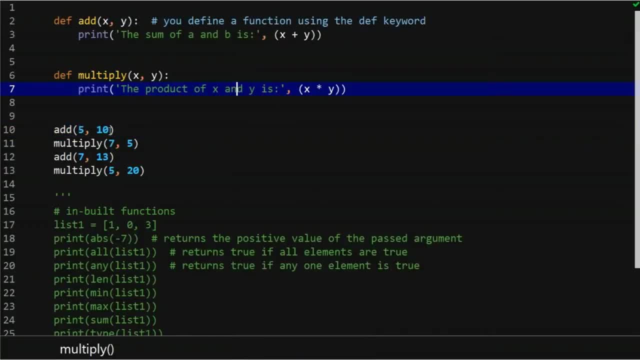 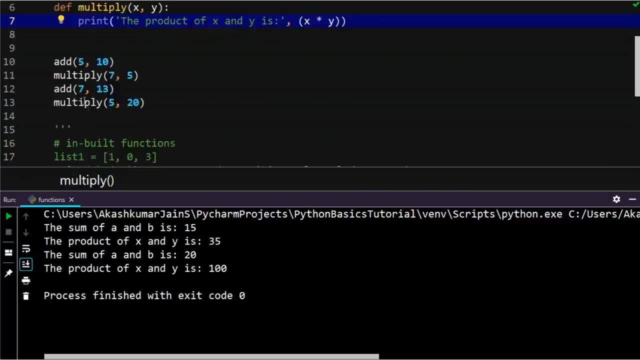 So let me just run this for you: You have 5 plus 10 will be 15. then you have multiply, that will be 7 into 5 will be 35. and then you have 7 plus 13 will be 20, and you have 5 into 20 will be 100. 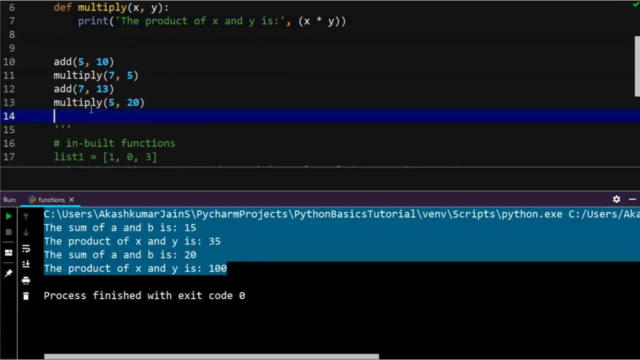 So, as you can see, this is how the functions work, And if you want to understand how functions are written, it is done using the def keyword and then followed the name of the function and then the parameters and, accordingly, the colon and indentations. 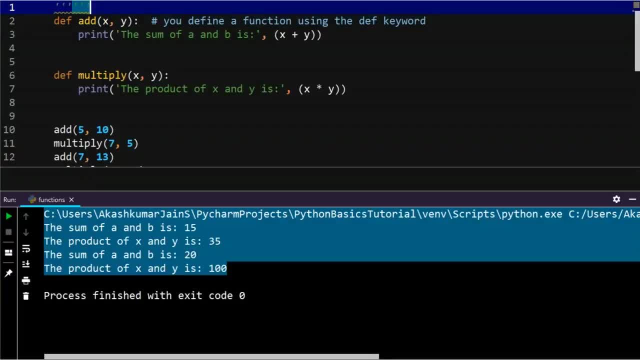 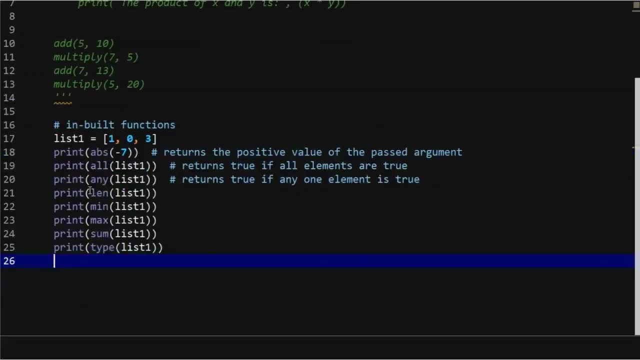 So that is how you define functions, And I hope you've understood what functions actually do in Python. So let's just go ahead and learn a few more of the built-in functions. Let me run the program. I have a list- 1, 0, 3- which we will be using later. 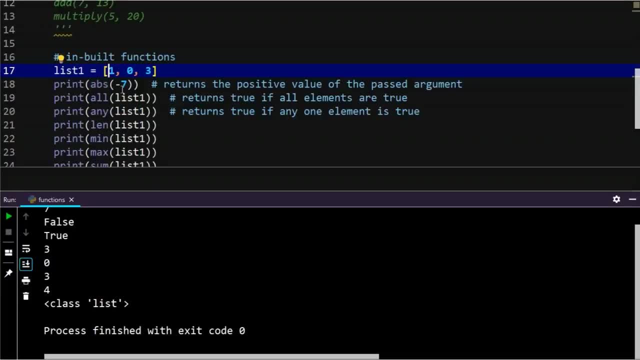 So next I am asking the absolute value of minus 7.. So the absolute of minus 7 is actually 7. now I have the all function and the any function. whenever I use the all function, it will return a true if all the values in it are true. the any function: 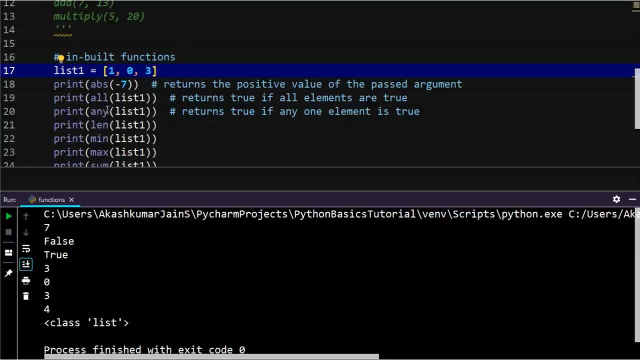 will return a value true, even if one of the values are true. So all will give me a false because I have a 0 over here, and any will give me true because I have at least one element that is true. So, as you can see, these are the outputs. next length function. 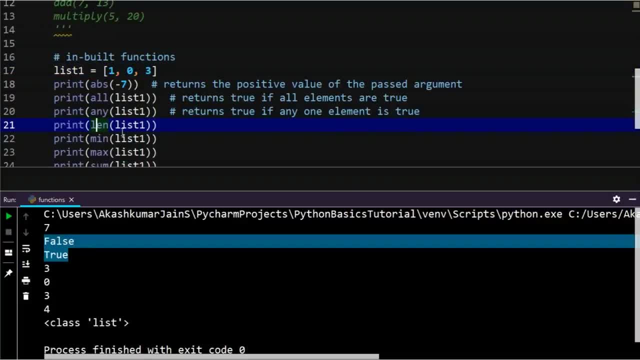 is basically used to give the length, So 3 over here. then I have the minimum and the maximum function. So the minimum function is used to give the minimum of the list, that is, 1, 0, 3 will be 0 over here and the maximum will be 3, so I get 0 and 3 over here. next is sum. 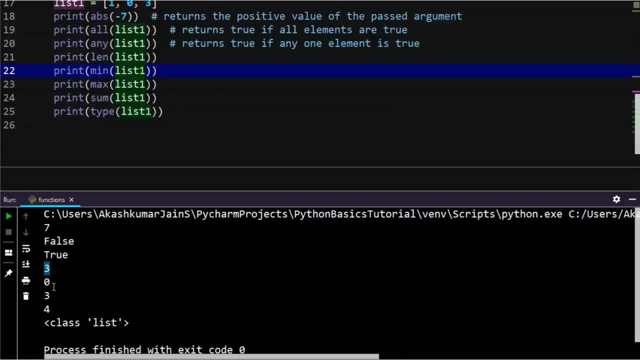 of the list. So, basically, the sum value is used to add all the elements in the list, and it's just not for list. You can even use it for tuples, You can use it for sets, all other sort of data types. This is just an example for you to show the different types. 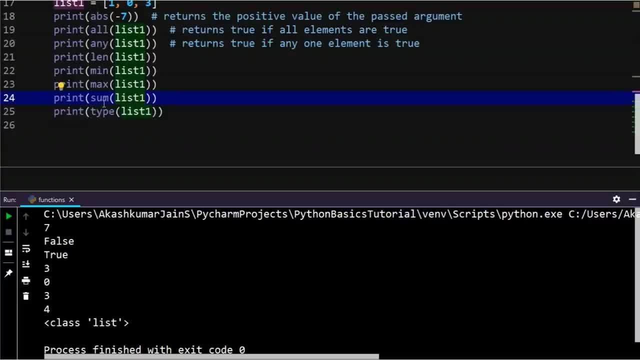 of built-in functions that Python already has for you to use, and I have the sum function over here, which is 1 plus 0 plus 3. 1 plus 0 is 1, and 1 plus 3 is equal to 4.. 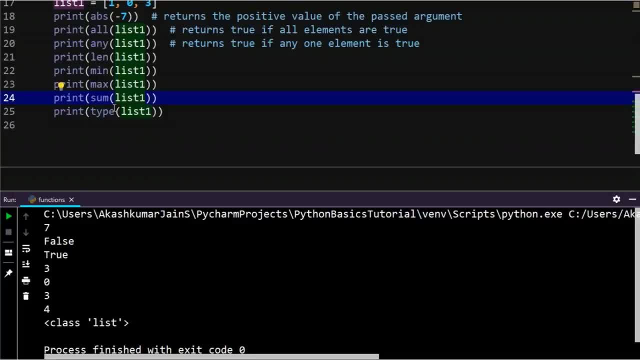 That's the reason I get a 4. and then I have type, which is used to give the type of the data that I have passed to it. So if I am passing a list, I will get the class as list. So that basically wraps up the session. 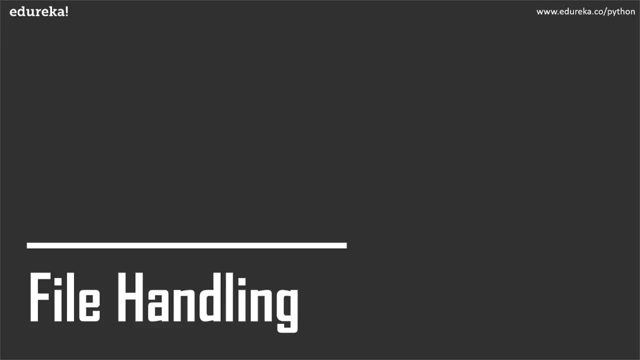 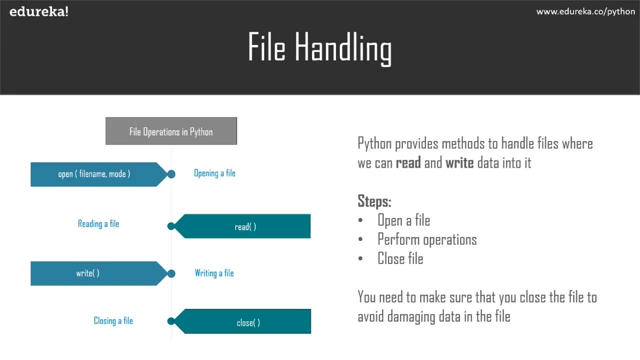 for functions. Let's just move ahead to the last topic of our day session: file handling. you would definitely know what is a file. It is basically where you have data stored inside them. So what is file handling? Well, Python provides you libraries which you can use to handle files within Python itself. 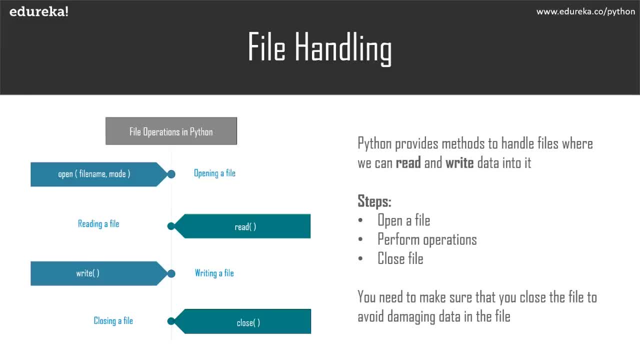 So you can read and write data to and from a file accordingly to however you want to. so what are the steps that you need to follow? There are basically three steps: you open the file, You can perform your operations and you have to close your file. 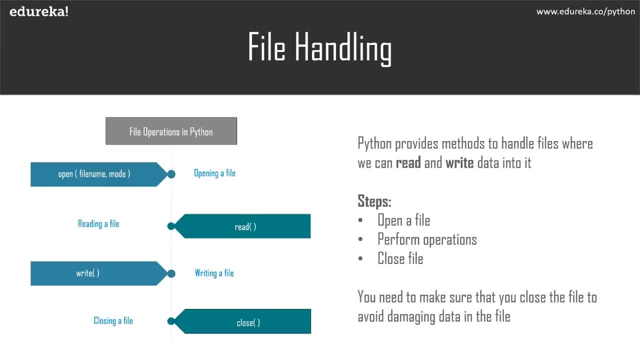 closing your file is really important because what happens is, whenever a file is being read or written to, it is basically bought into the memory. Now, if you do not close the file, it will still remain in the memory and there are chances that the file gets corrupted. 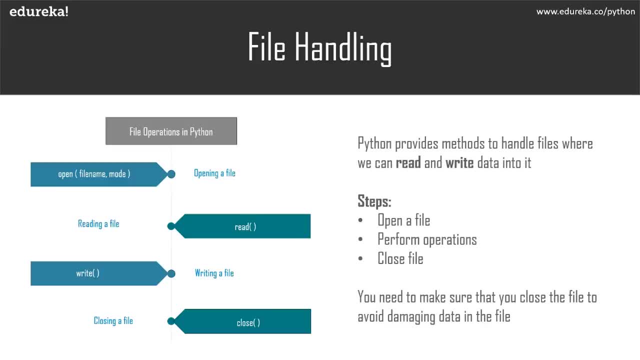 So to avoid that damage, please make sure that you close your files. These are the different operations. So for opening a file you use the open command and then file name and the mode. So mode may either be the read or the right or the append mode. then to read the data: 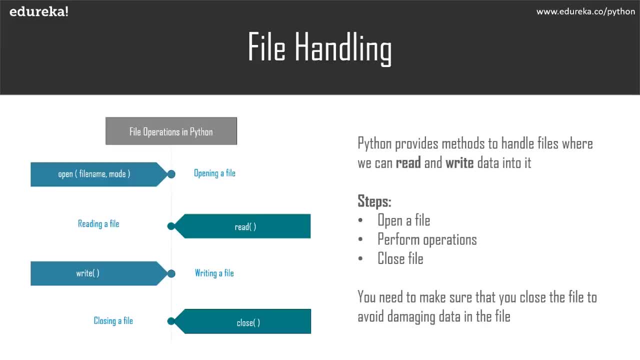 You use the read function to write, you use the right function and to close you have the file dot close function. So let's move ahead to our tutorial and let me open up file handling. So, as you can see, I have some data in this particular file. 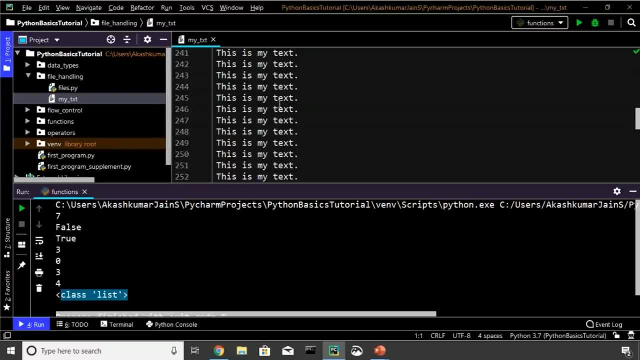 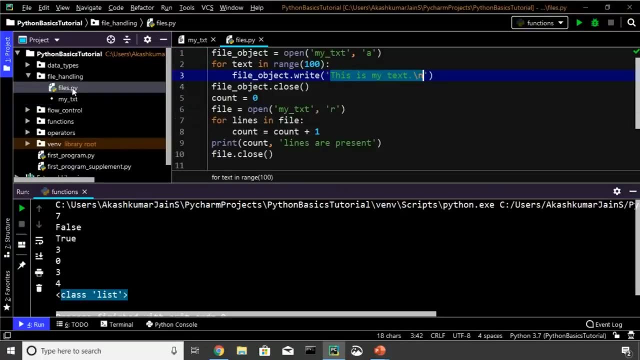 That is, this is my txt. Let me just close all of this, or let me just remove all the data that this has. so let me just go ahead and save this and open files, dot py, and let me go back to my presentation mode. So now we have a file object. 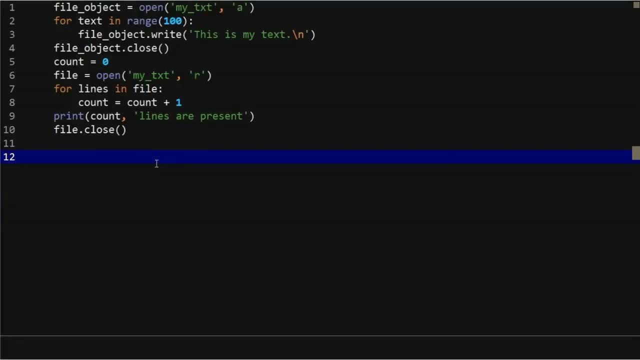 So whenever you want to open a file, you have to make sure that you open it into a file object. So now I am just using that, so file object is equal to open, and I am seeing that I have to open my txt and let me just open. 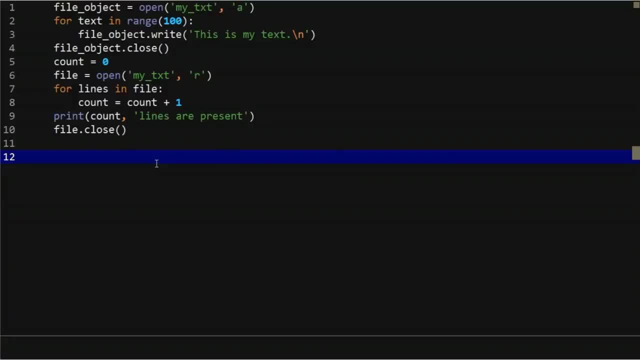 I'll open it in the right mode and then I am just seeing for text in the range of 100 file object dot right. This is my text, and then I close it. So this is one part of where I am writing data into the file. 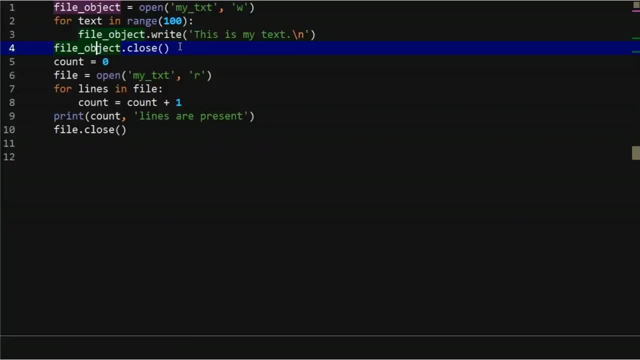 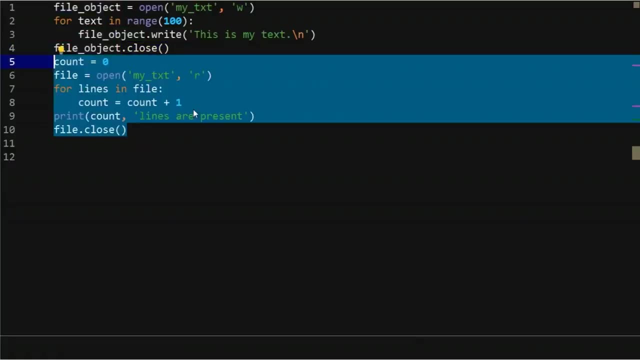 The next part is where I am reading the data from the file. So I just have a count to see how many lines of data is there in the file. So I have file equal to open my txt in the read mode. Then I have four lines in the file. count is equal. 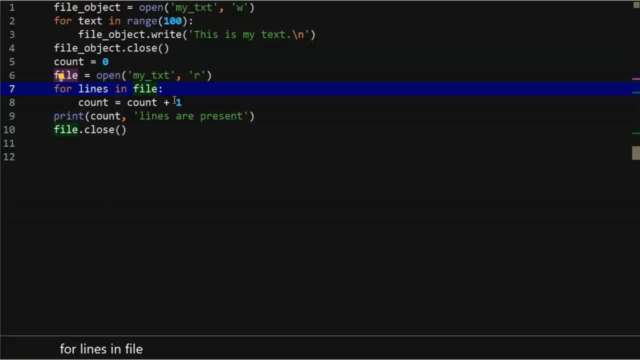 to count plus one. So just print there are count is equal to lines are present, count lines are present and then I close the file. So, as you can see, I opened a file, I perform my operations and I close the file over here Also, I opened the file, perform my operations. 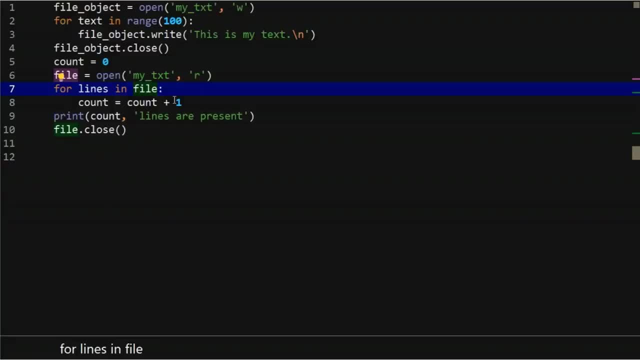 and close the file whenever I have the right mode. right mode is basically used to write data into the file. Now, if there was data that was previously present in the file, that will be removed and rewritten or overwritten. So that is where we use the right function. 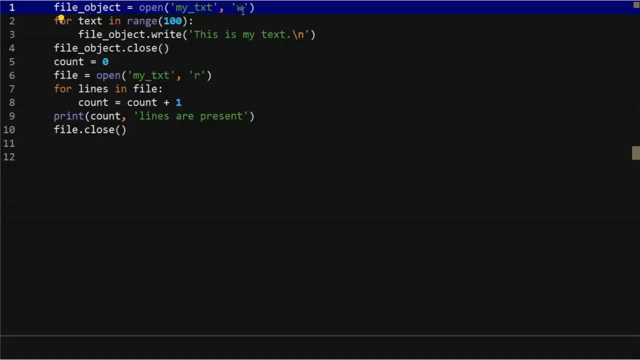 We have the, a function which is used to append data. It will not delete the previous data that was available, but just add data into it, and then the read or read mode is used to basically read the data from the file. So let me go ahead and run this for you. 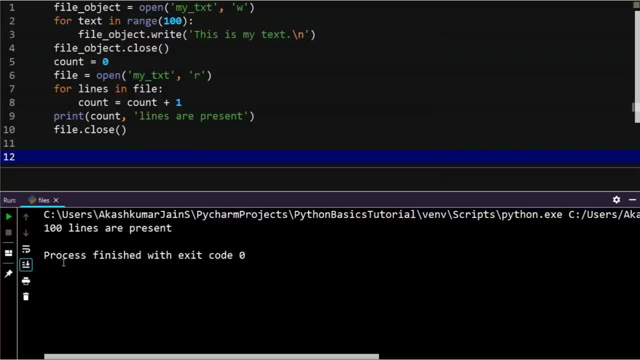 So, as you can see, right now there are hundred lines present. Let me run this again for you: There are a hundred lines present And let me show you that there are hundred lines that are present right now. So that's simple. So if you saw that previously I ran the program two times. 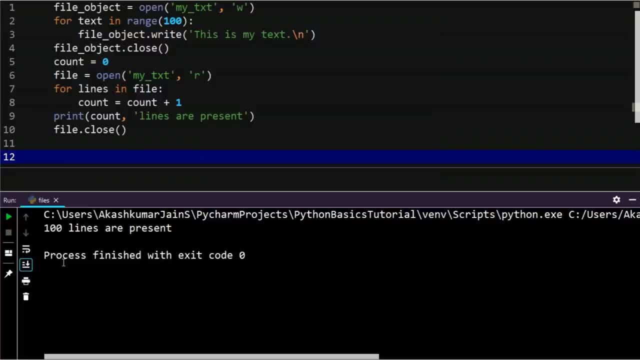 and it was still showing hundred. now let's see what happens Now. it should be 200. that means a hundred lines are added into the file. now again hundred lines will be added. that becomes 300.. So basically that is how we have file handling in Python. 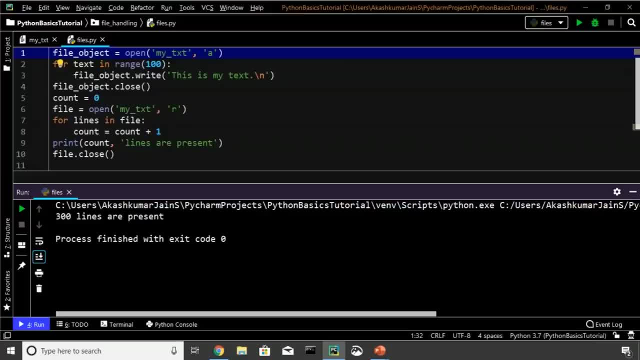 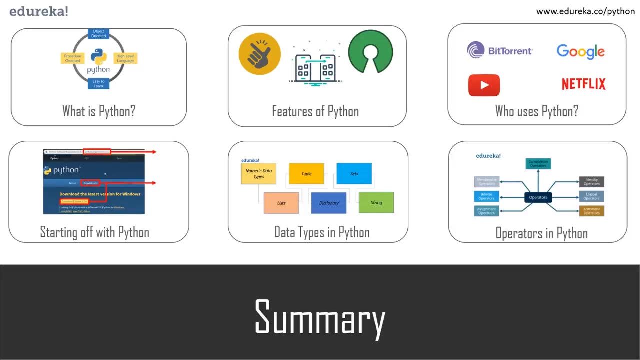 You can accordingly keep changing and keep experimenting to know more about it. So that basically wraps up this session for Python basics. So let us just go ahead and find a summary of what we have studied. We basically studied what Python is, its features and who are the companies who use Python in the industries. 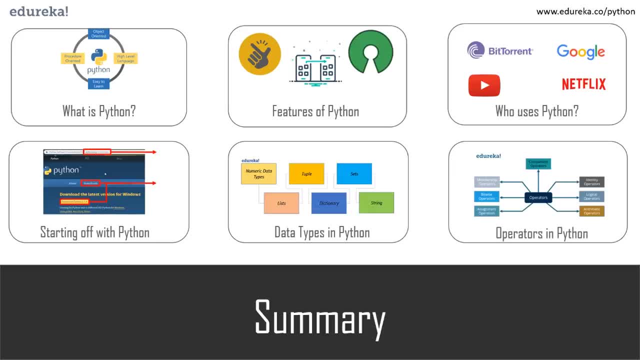 Then we installed Python. He looked at the different data types Python has to operate- is that Python has? and then we understood what is flow control, What are the functions and what is file handling. that basically wraps up our session for Python basics. I hope all of you have had a good time.